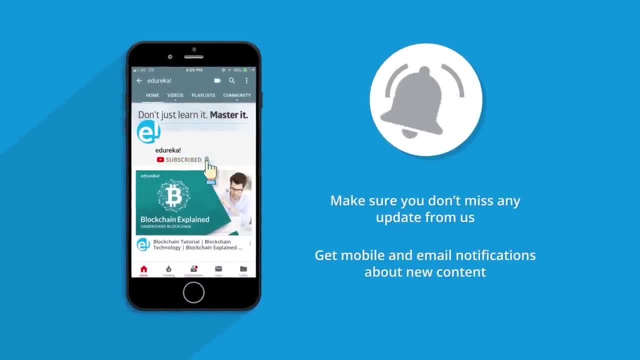 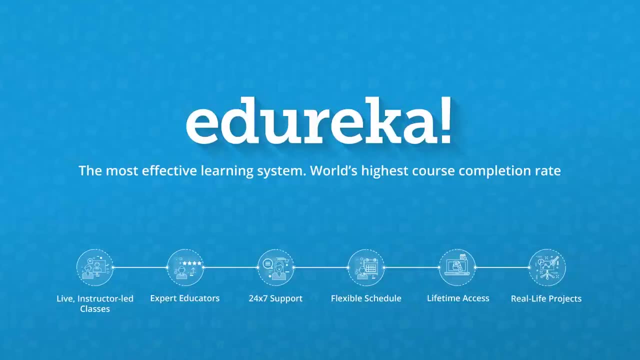 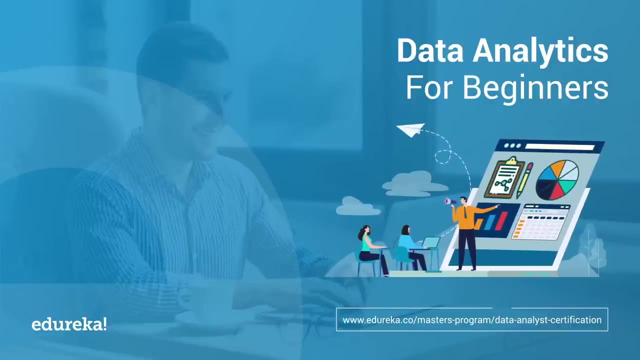 Hi everyone, this is Sahitya, on behalf of Video Rekha, and I welcome you to this session on data analytics for beginners. So this session will help you understand how you can start with data analytics. So before I begin with session, let me just quickly cover the concepts. 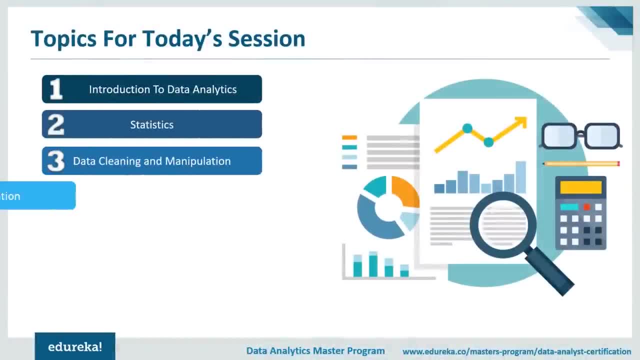 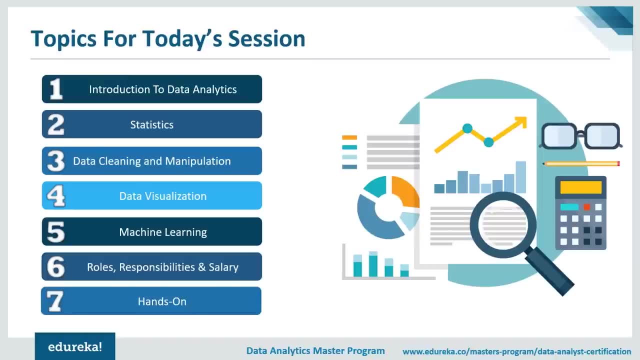 that we're going to cover in today's session. So we'll start today's session by understanding the introduction to data analytics, and then I'll tell you what is statistics. after that I'll tell you how you can perform data cleaning and data manipulation, and also data visualization. 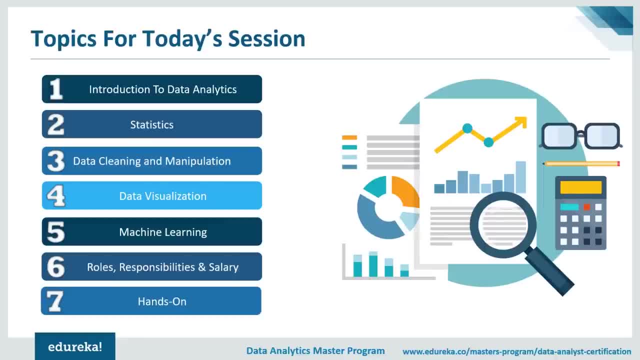 Once you understand the basic skills- that is, the statistics, data cleaning, data visualization- I'll tell you the plus point of a data analyst- that is a machine learning. So I'll just talk about machine learning a little bit and then I'll tell you the roles and responsibilities. 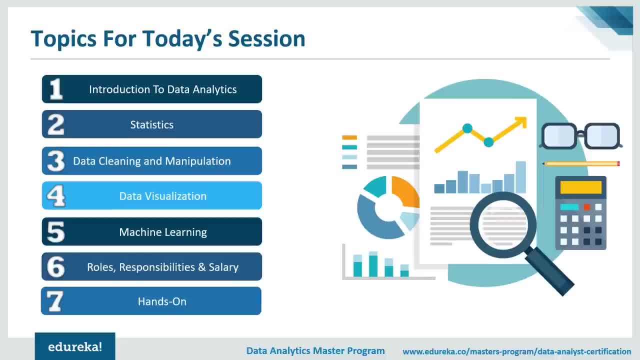 and salary of a data analyst. Once you understand all the theory part of the session, I'll end this session with a hands-on part where we'll see how you can perform data analytics on a specific data set, right? So I hope that you know the agenda is clear to you guys. 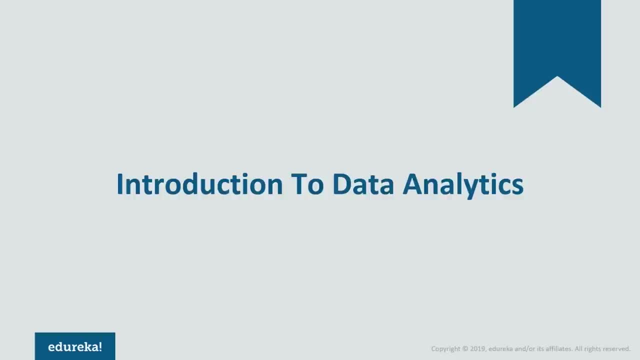 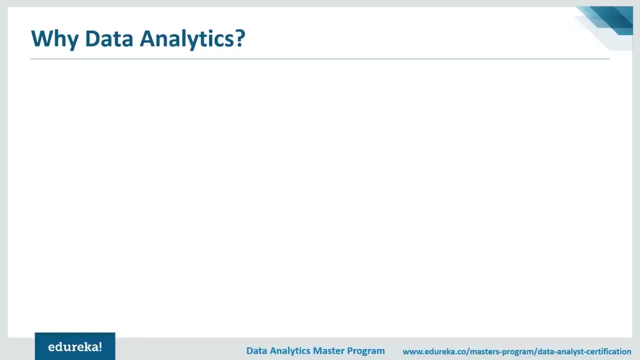 So now, as I said, the first topic is introduction to data analytics. Let me just quickly cover Why do we need data analytics. So, with the presence of humongous data around us, it's obvious that you know we need to analyze the data for our benefits. 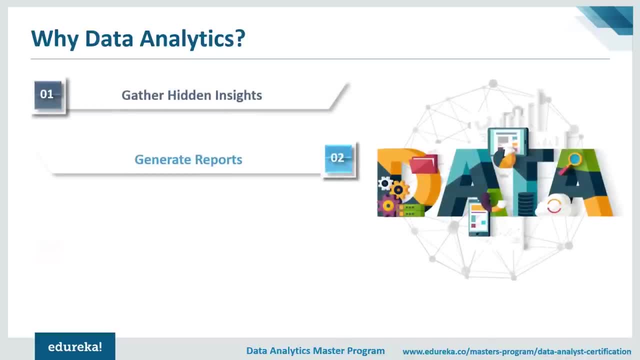 either for gathering the hidden insights or for generating reports. data analytics benefits the enterprises by performing proper market analysis and improving the business requirements. So in today's market, this field has gained a lot of popularity in terms of number, because it lets you gather hidden insights, generate reports. 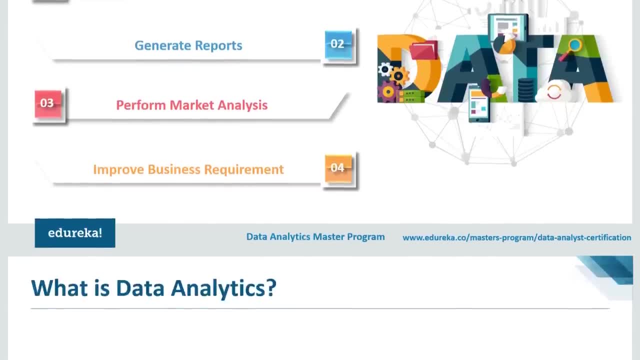 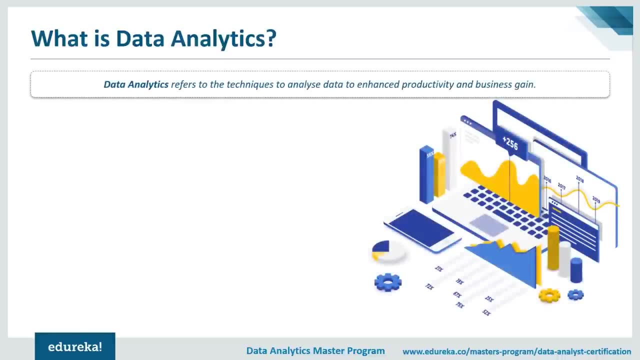 perform market analysis and also improve business requirement. So, with the note of this, let me tell you what exactly is data analytics. So as the word data analytics, such as data analytics, refers to the techniques to analyze the data, to enhance the productivity and business gain, data is extracted. 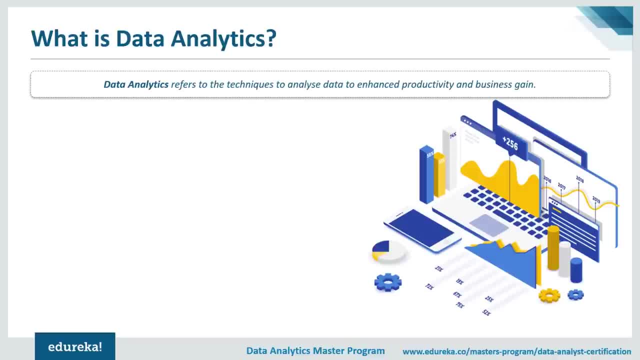 from various sources and is categorized to analyze different behavior patterns. Now the techniques and the tools used to, you know, perform data analytics vary from organization to organization, or you can say individual to individual right. So if I have to define data analytics for you, 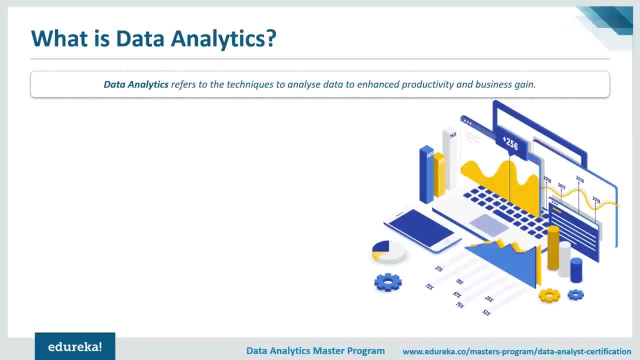 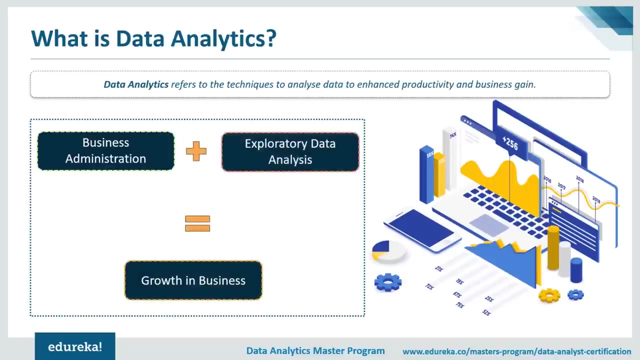 then data analytics is the process of inspecting, cleaning, transforming and modeling the data, with the goal of discovering useful information, suggesting conclusions and supporting decision-making. So, in short, if you have an understanding of your business administration and also have the capacity to perform exploratory data analysis, 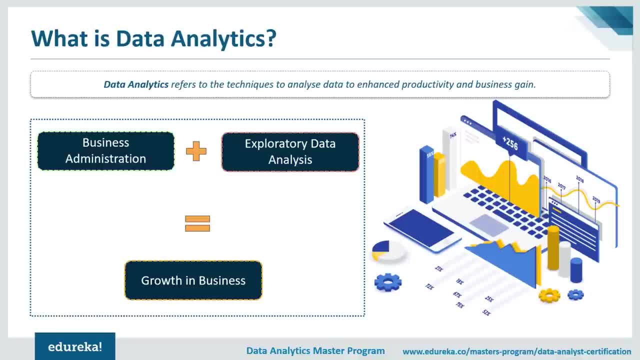 to gather the required information, then you're good to start the carrier in the data analytics feed. So, talking about getting data analytics: once you understand and you have the capability of performing business administration with exploratory data analysis, you would become a data analyst. 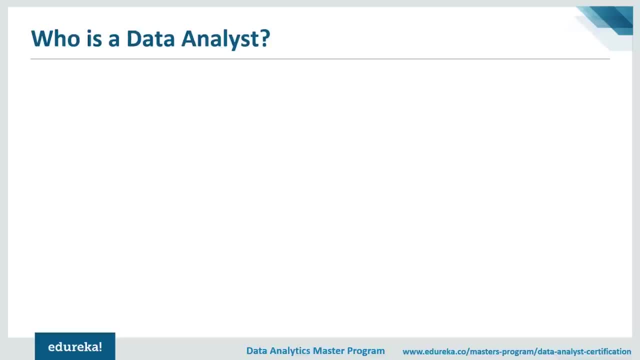 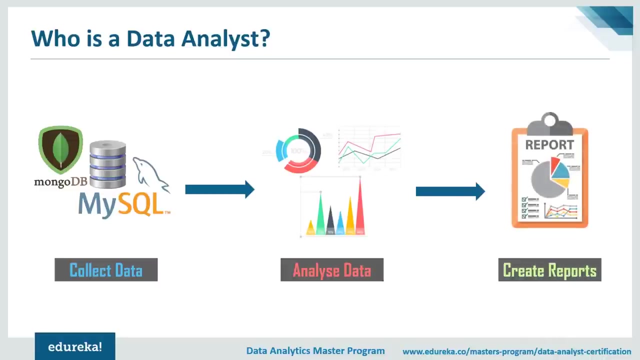 So now let me just quickly tell you who exactly is a data analyst. So data analyst is a professional who collects the data from various sources and analyze the data on various aspects and then finally generates the reports. Now these reports are distributed to the respective teams. 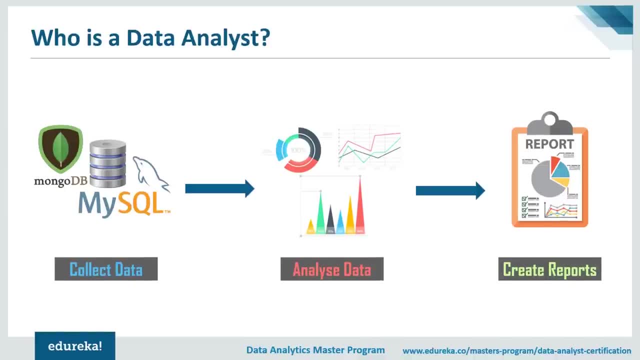 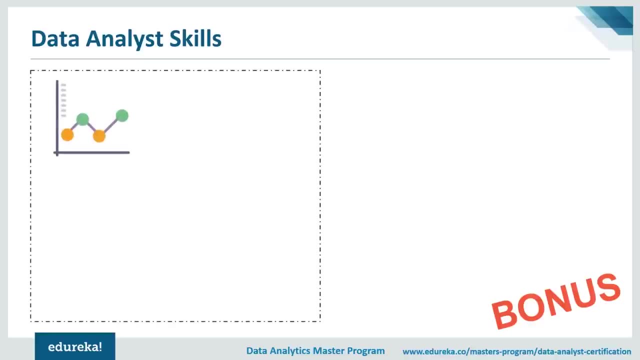 to use the analyzed data and provide improvement in the business. So if you have to become a data analyst and you need a set of skills, as you can see on the screen. So the basic skills that data analyst should possess are the ability to perform statistics, data cleaning, 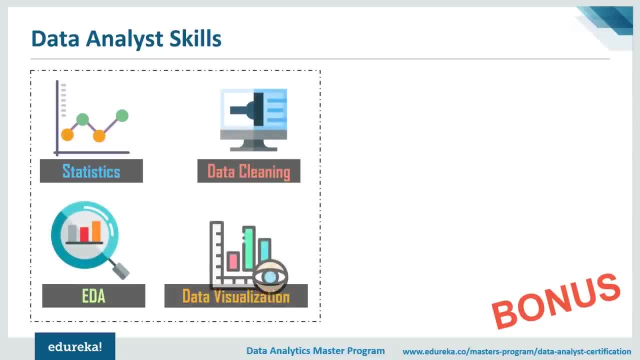 and also have the capability to perform exploratory data analysis and data visualization. apart from these skills, If a data analyst also has a knowledge of machine learning, then that would obviously add a bonus point to his or her skill set, as he or she would be able to build a model. 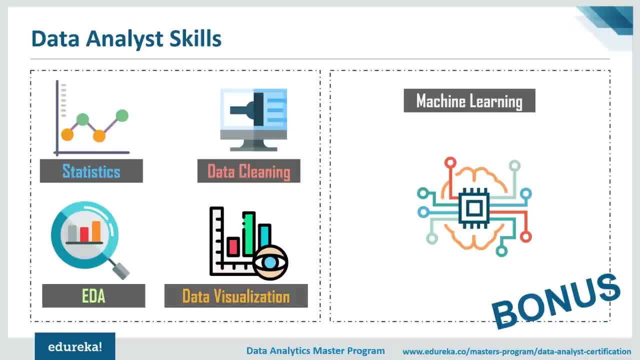 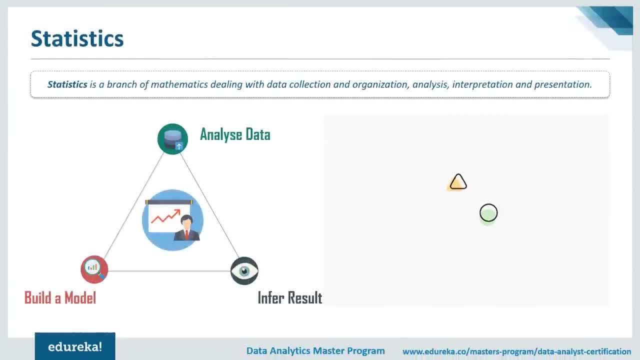 and then test the model, also right. So don't worry guys, I'll be talking about each of the skills one by one, starting with statistics. statistics is a mathematical science pertaining to data collection, analysis, interpretation and presentation. It is used to process complex problems in real world. 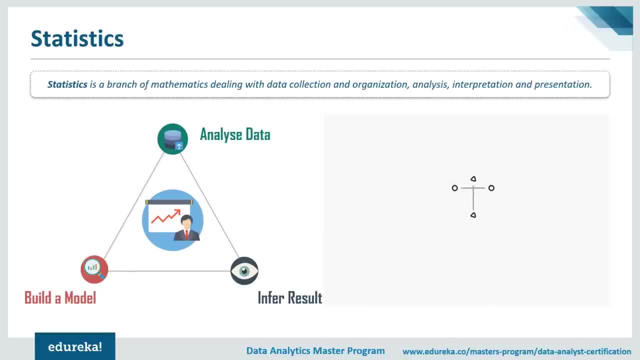 so that the analyst can look for meaningful trends and changes. analyst review The data So that you know they can reach conclusions. and several statistic functions, principles and algorithms are implemented to analyze the raw data, build a statistical model and input or predict the result. 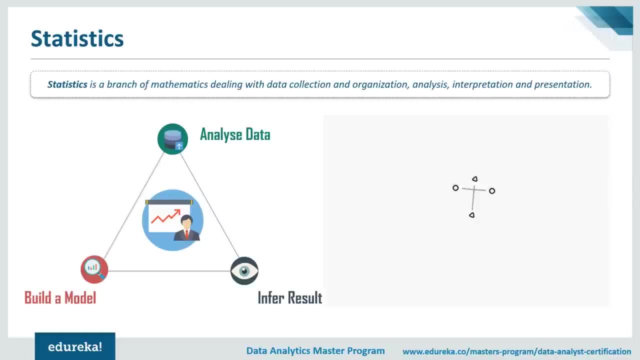 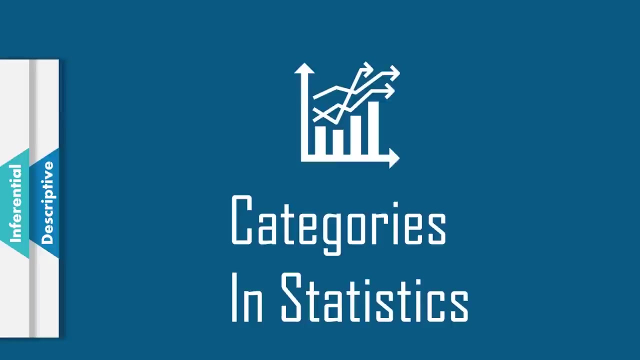 So if you just have to understand statistics in a single sentence, then statistics is a branch of mathematics dealing with the data collection and organization and then performing analysis, interpretation and presentation right. So statistical analysis has basically two categories: the descriptive statistics and the inferential. 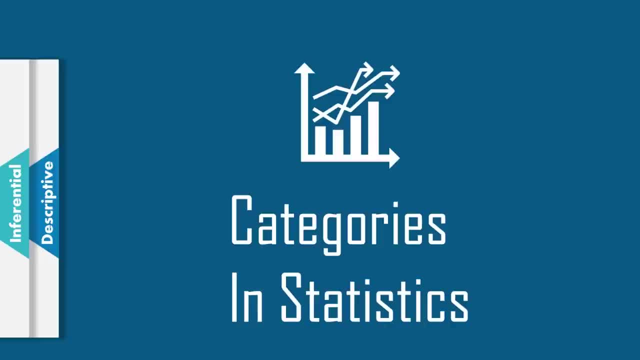 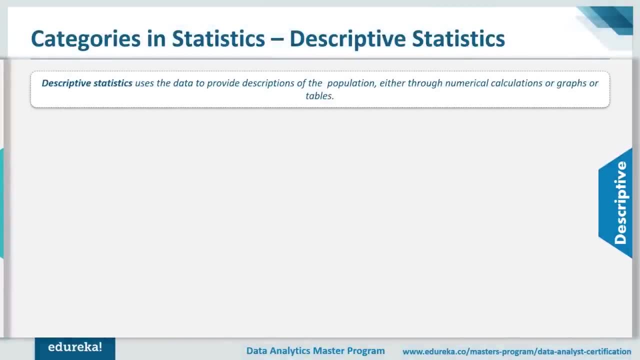 Statistics, so let's get started by understanding each one of them, one by one. So, starting with descriptive statistics, descriptive statistics uses the data to provide descriptions of population, either through numerical calculations or graphs or tables. So now descriptive statistics helps organize data and focuses on characteristics of data, providing the parameters. 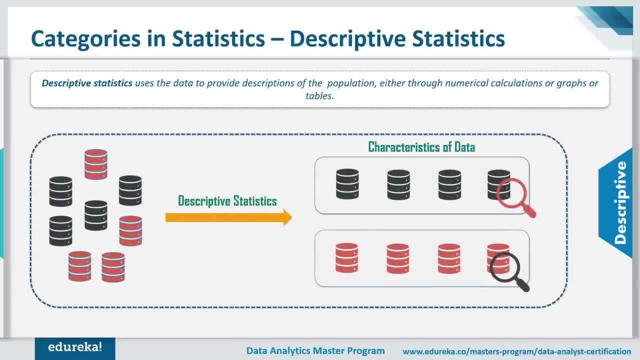 So, as you can see the example on the screen, suppose you want to distinguish the objects based on the color. Then you can see that this type of statistics, that is basically the descriptive statistics. It divides the data into two sections based on the colors. 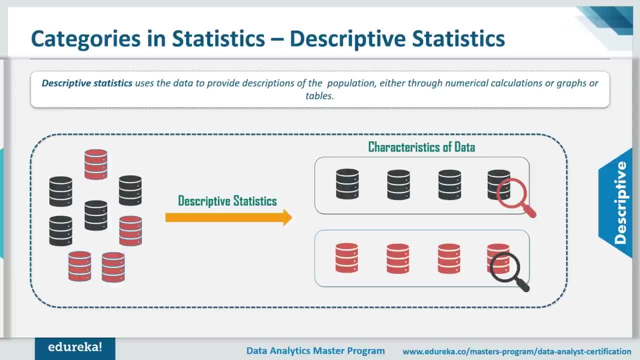 So that's black and red over here. Now, if I have to make it more generalized for you, then suppose you know you want to study the average height of students in a classroom in descriptive statistics. What you would do is you would record the heights. 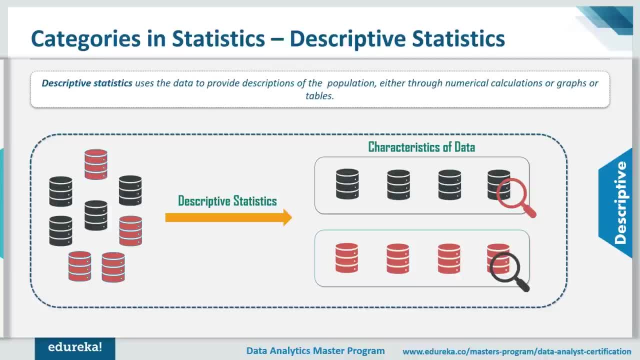 of all the students in the class and then you would find out the maximum, minimum and the average height of the class right now. This was just a simple example, guys, If you look into the enterprise level, then you may have a large data set. 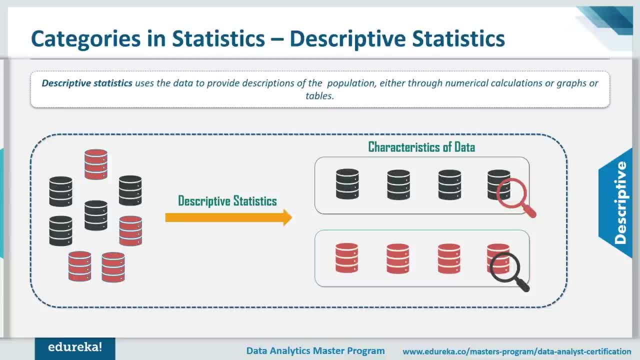 you know, with various number of columns, right? So you can just pick up one column and then you can find the minimum, maximum and the average of that particular column, right? Also, in descriptive statistics we try to represent the data in the form of graphs. 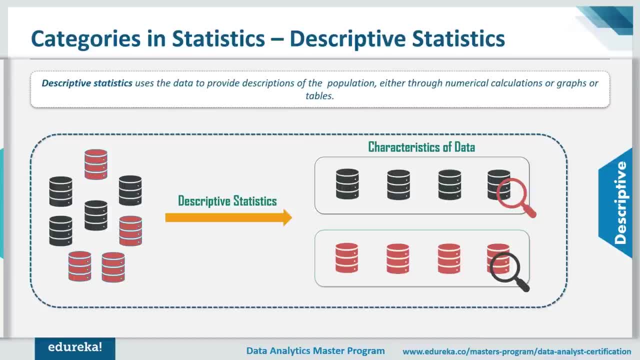 like histogram, blind plots, scatter plots and so on. But yes, the data is represented based on some kind of central tendency. Now, when I say central tendency, I mean that you know particular graph represents the distribution of mean or the measure of spread on. depends on what kind of a graph you're using. 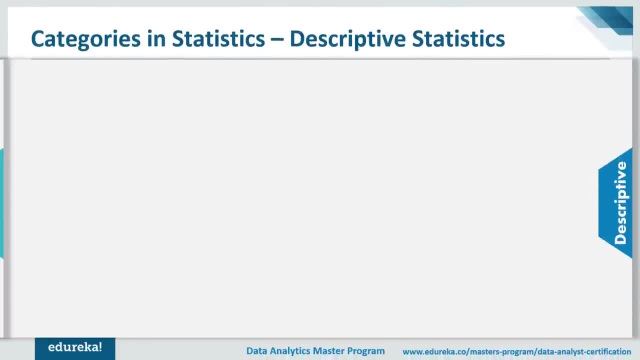 or what's on your graph right. So for that you have to understand few measures in statistics. So those are basically the measures of Center and the measures of spread. So talking about the measures of Center, there are mainly three terms that you need to understand. 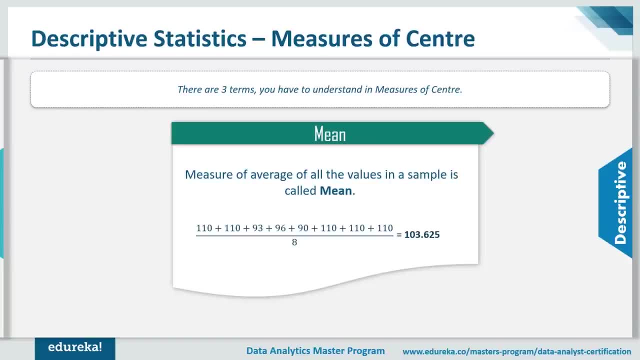 which are the mean, median and the mode. So starting with the mean, mean is basically the measure of average of all the values in the sample. So suppose you know, if you consider the example in the screen, then if you want to calculate the mean of the sample, 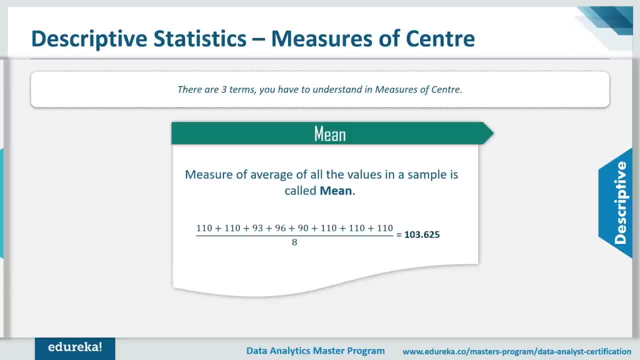 that is present on the screen. you just have to add all the numbers and divided by the number of numbers, right? So since we want to find the mean of 8 values, we're going to divide the complete sum by 8, and that's how you can calculate the mean of the sample. 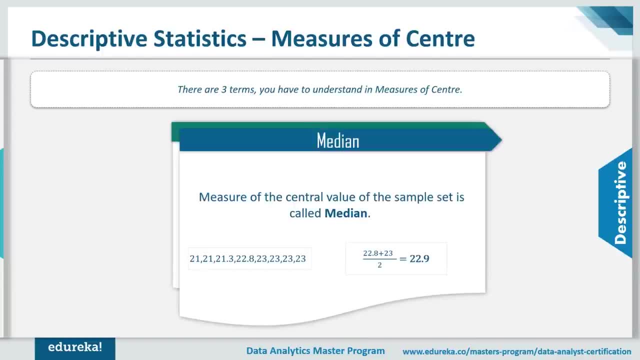 All right, moving on to the next term, that is, median median is basically the measure of central value of the sample set. So if you consider the example on the screen then you can see that you know there are eight values right now to calculate the median. 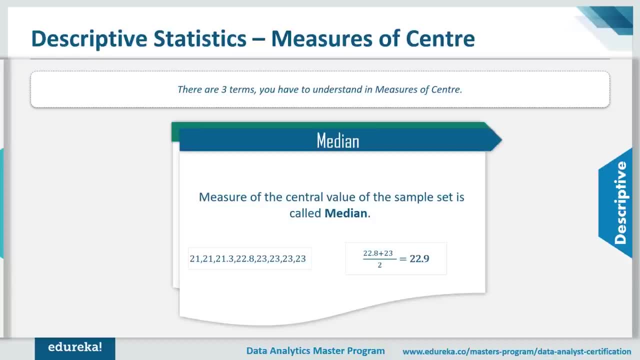 You have to consider the fourth value and the fifth value and then divided by 2.. So, since our fourth value over here is 22.8 and the fifth value is 23,, I'm just going to add both these values and divided by 2.. 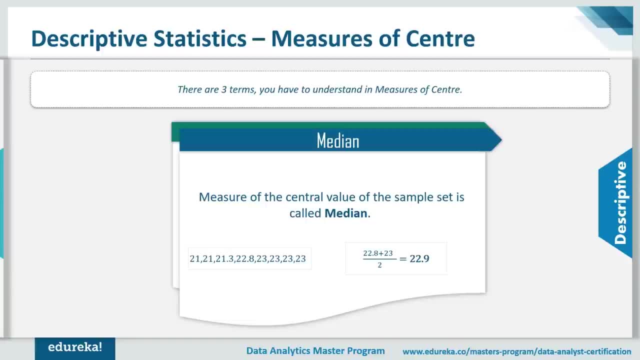 So the value that you get, that is, 22.9, is the median of the sample right now. moving on to the next term, that is, mode. mode is nothing but the value most recurrent in the sample set. So if you consider the example on the screen, 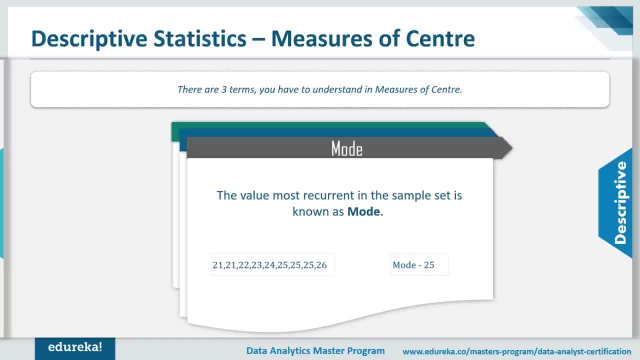 then out of all the numbers that you see on your left hand side, you would see that you know, 25 occurs the maximum number of times right. So 25 would be the mode for this particular sample set, So as in when the sample set changes, the mean median. 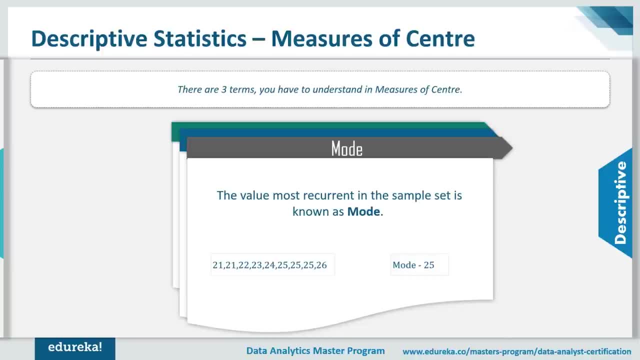 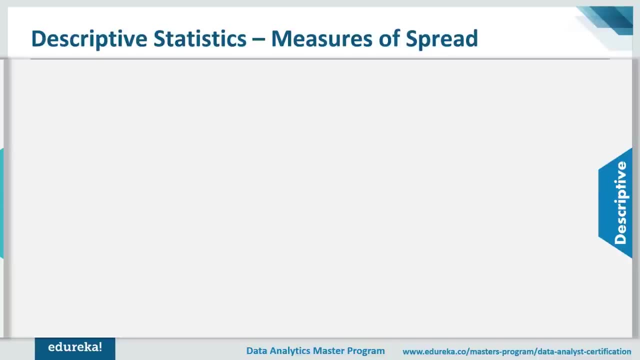 mode values also. so change right. So those were the measure of Center guys. now moving on to the next measure, that is, the measure of spread. the measure of spread again, has basically four terms that you need to understand. that is the range in the quarter range variance. 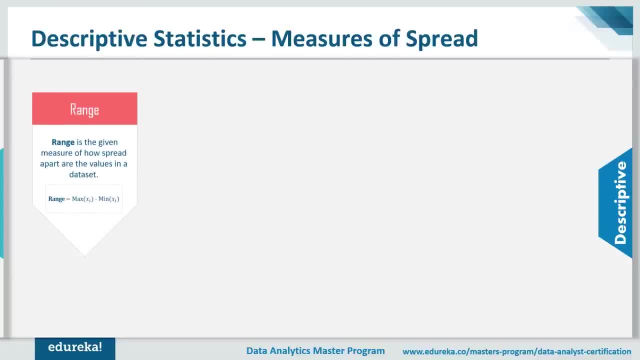 and the standard deviation starting with the range. range is basically the given measure of how, spread apart, the values are in a data set, right? So suppose you know you have 10 values, that if you want to calculate the range of these 10 values, 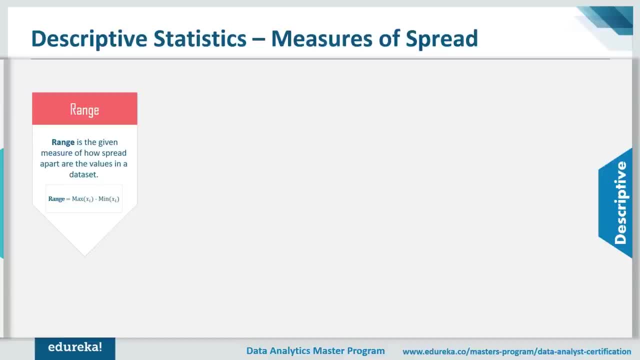 you just have to subtract the minimum value from the maximum value, right? So that's what the formula is, guys. that is maximum minus minimum. now moving on to the next term, that is, the interquartile range. interquartile range is basically the measure of variability based. 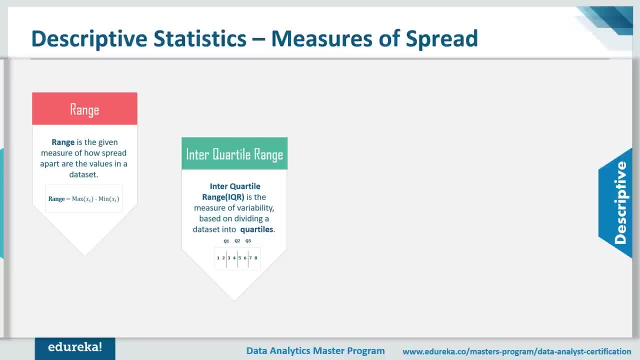 on dividing the data sets into quartile. now, to understand quarter is that we just consider the sample set of eight values, right? So let me just quickly open my notepad and show you how you can calculate the interquartile range. So let's say you know. 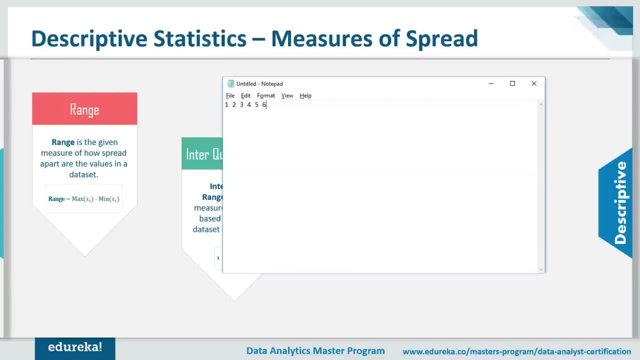 we have eight values: 1, 2, 3, 4, 5, 6, 7, 8. now to calculate the interquartile, Interquartile range. What you simply have to do is: first you have to calculate the quartiles. right now to calculate the quartiles. 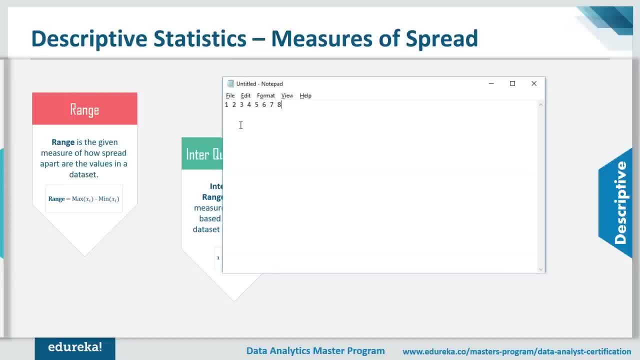 You have to find the average between two numbers. So when I say two numbers, you have to calculate the average between 2 and 3, then you have to calculate the average between 4 and 5, and then you have to calculate the average between 6 and 7, right? 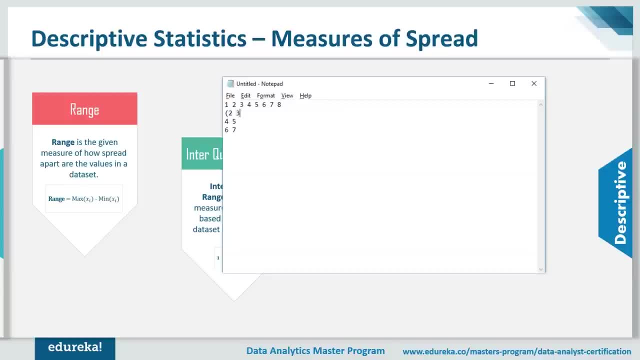 So let me just quickly calculate the average. So what I'll do is I'll just add these two terms and then I'll divide it by 2, right? So this would be equal to 2.5.. So that's 2 plus 3 by 2, that's 5 by 2, is 2.5. 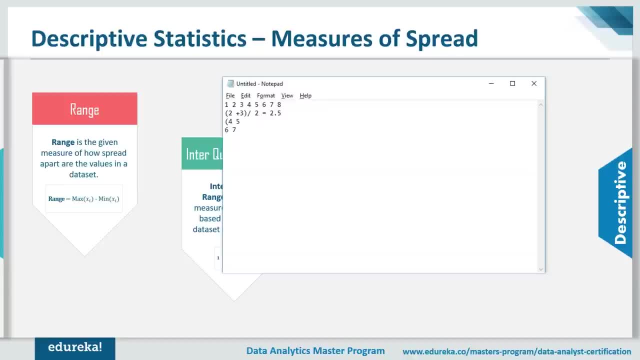 Similarly, I would calculate: 4 plus 5, that is 9, 9 by 2 is 4.5.. So I'm just going to put 4.5 over here, So let me just write that. and then finally let's just add 6 plus 7, that is 13 by 2, that is again 6.5, right? 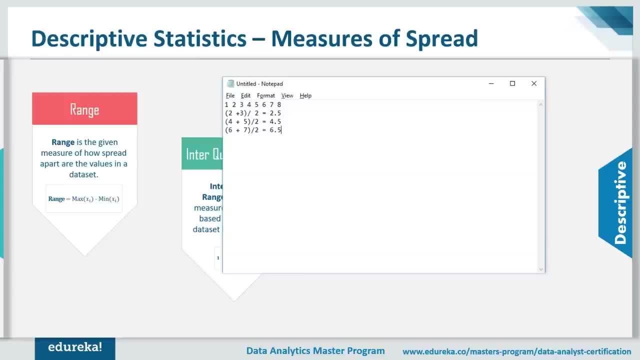 So basically you have three values, that is, 2.5, 4.5 and 6.5.. So basically these values would define your quartiles. So the first quartile would be after 2,, the second quartile would be after 4. 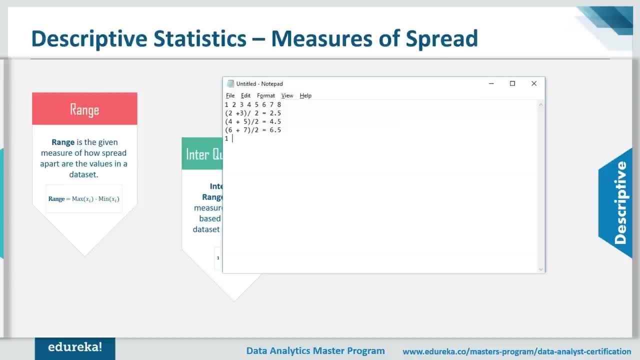 and the third quartile would be after 6, right. So what will happen is your sample set would be divided like this, right? So, as you can see on the screen, we have four quartiles. Now the difference between the first quartile 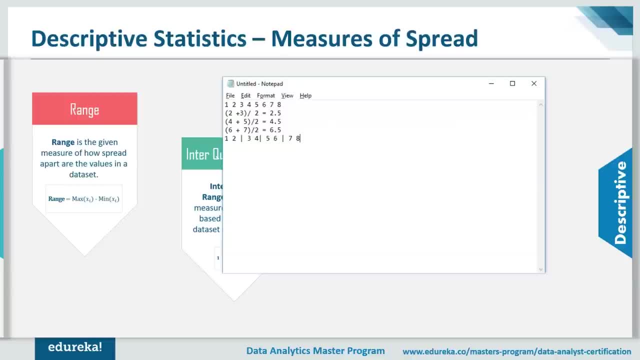 and the third quartile would be your interquartile range. So if you just want to calculate interquartile range, what you simply have to do is we have to first calculate the quartiles for your sample set, and then the difference between two quartiles would be. 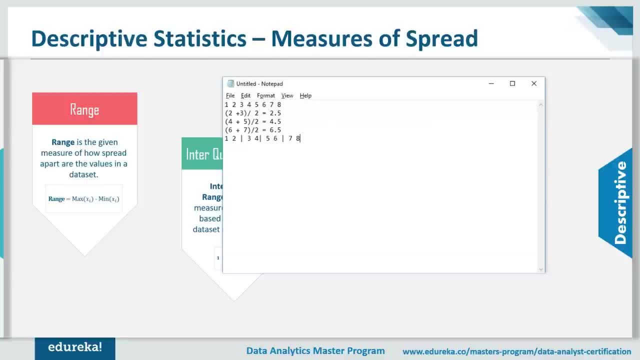 your interquartile range, right? So I hope I'm clear with this part. Now, moving on to the next term, that is, variance. variance basically describes how much a random value differs from its expected value, right? So, basically, whenever you want to calculate, 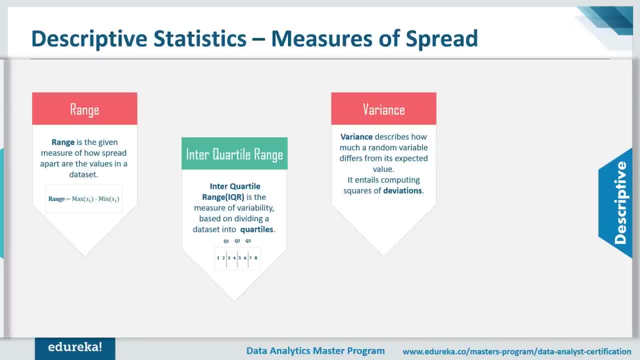 how much any random value differs from its expected value. then you're basically calculating variance. It basically entails the computing squares of deviations. Now, with that, let's move on to the final term, that is, the standard, The deviation. so standard deviation is basically the measure. 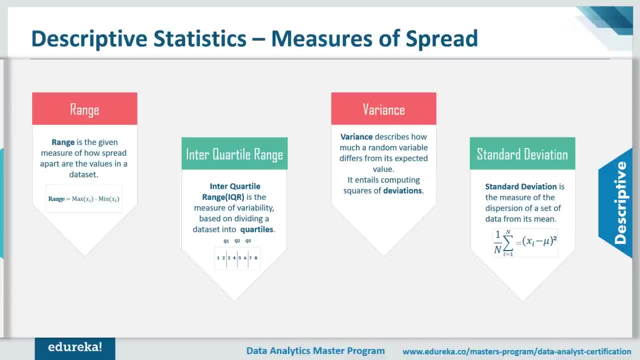 of dispersion of set of data from its mean right. So whenever you calculate the mean and then whenever you want to calculate how far is the dispersion of the set of data from its mean, you would basically calculate standard deviation. So, folks, I'm not going to go into depth of you know. 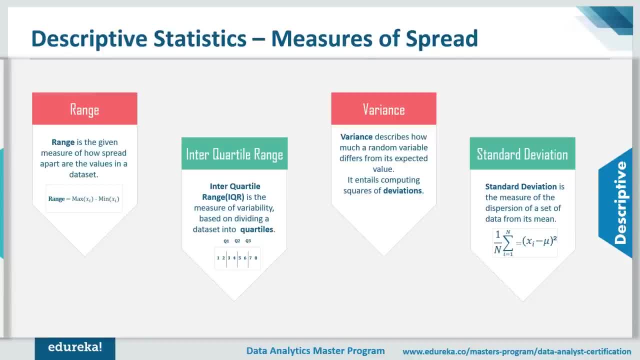 how you have to calculate each of these terms. if you want to learn more about statistics, I leave a videos link in the description box and you can refer to that video. that is basically statistics for data science, where you'll understand all these terms based on statistics. 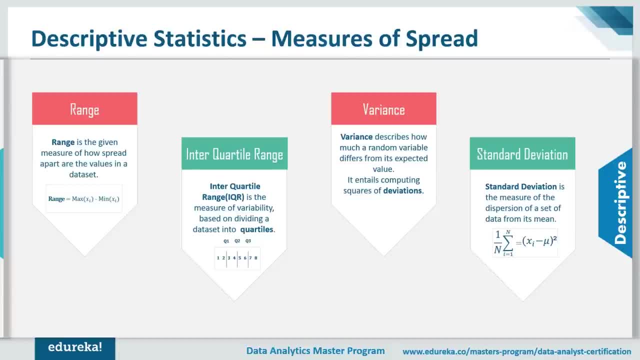 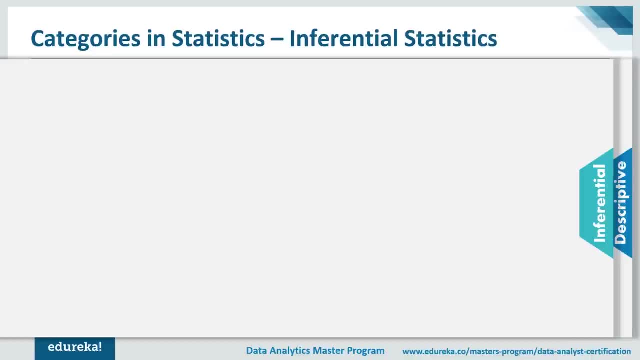 and you'll understand how you can calculate the values right. So, guys, that was all about various measures that you need to go through in descriptive statistics. Now, moving on to the inferential statistics, That is the second category in the statistics. This is basically used to build a model. 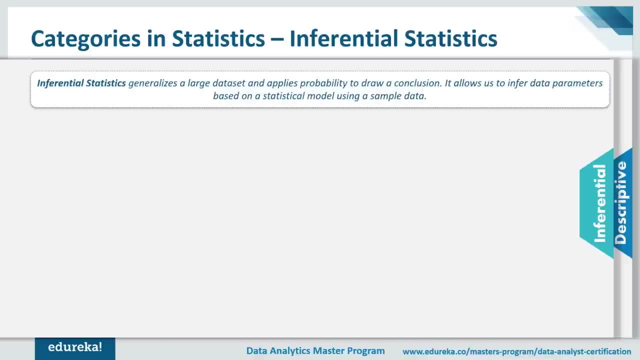 and then give a probable solution. So inferential statistics basically generalizes a large data set and applies a probability to draw conclusion. It allows us to infer data parameters based on statistical model using a simple data set. So again, let's just take the same example of. you know, 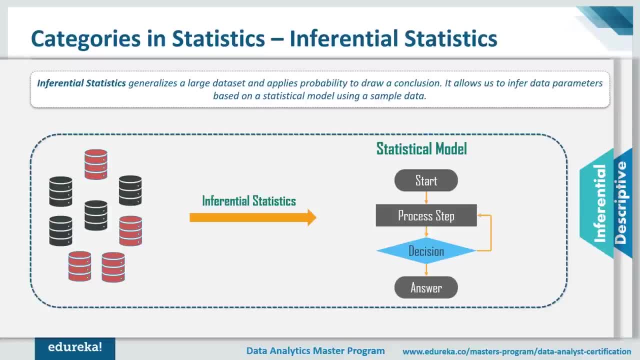 we have to segregate few objects based on the color. now, when you implement inferential statistics on the same objects, what would happen is a statistical model will be built and based on that a conclusion would be given. right. So that's how you know inferential statistics is. 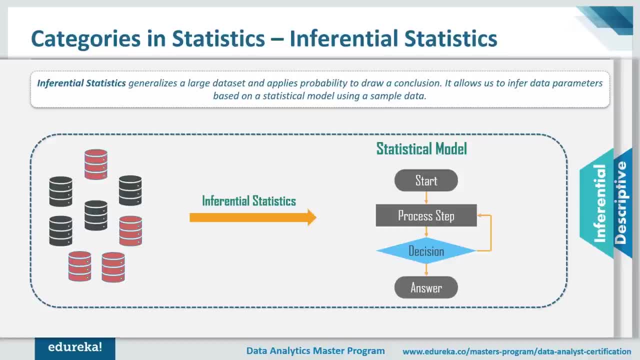 if you have to understand, if I have to generalize this for you, then you can again take the example of calculating average height of students in a classroom over here. What would happen is we would take a sample set of the class and then, if you want, 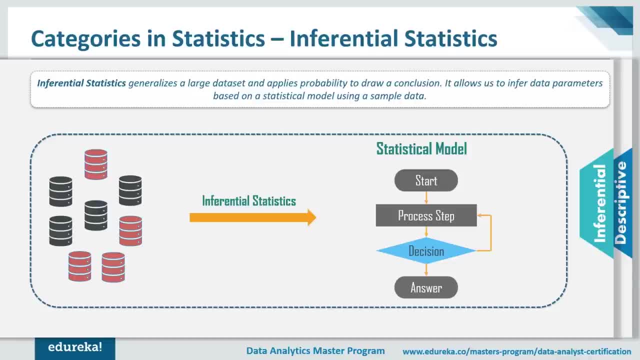 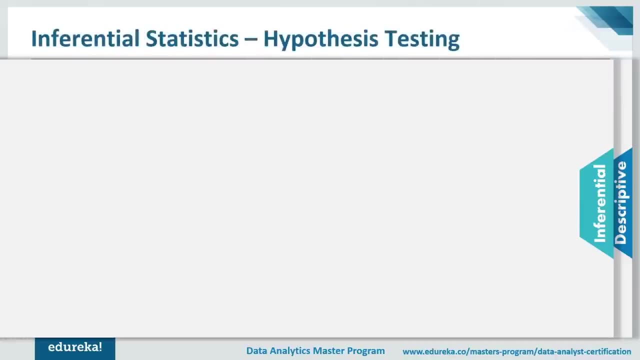 to apply inferential statistics. what we would do is we would group the students into tall, average and short height and then, based on this, we would build a statistical model and expand it for the entire population, right? So, guys, that was all about descriptor statistics and the inferential statistics. now, inferential statistics has one. 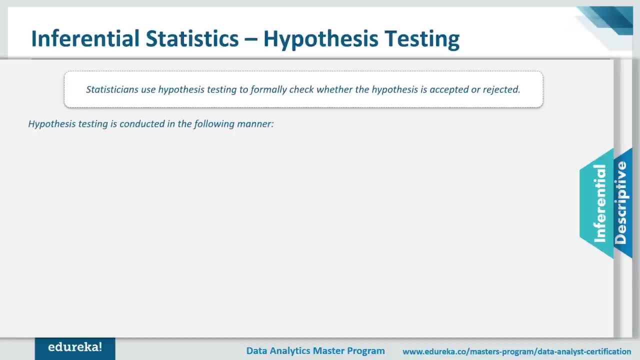 more term, that is hypothesis testing, that you need to understand. So hypothesis testing is an inferential technique to determine whether there's enough evidence in the data sample to info whether a certain condition holds true for an entire population or not. So what basically happens is under the characteristics. 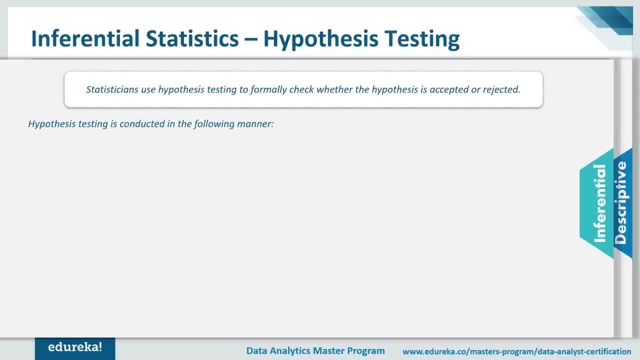 of general population. We take a random sample and analyze the properties of the sample, we test whether or not the identified conclusion represents the population accurately and finally we interpret their results right. So whether or not to accept the hypothesis completely depends on the percentage value we get from the hypothesis. 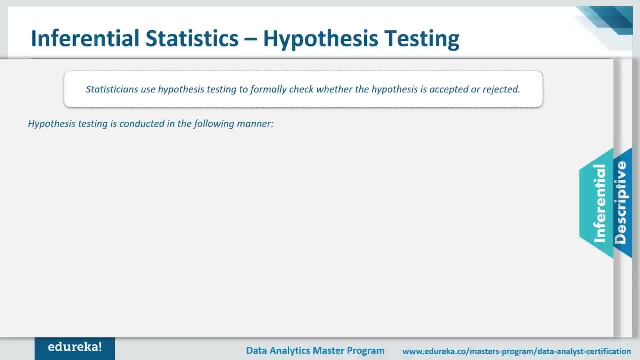 So hypothesis testing is basically conducted in the following manner that you can see on the screen. It starts with the state of hypothesis and this stage basically involves stating the null and the alternative hypothesis. Then we basically formulate an analysis plan where the stage involves the construction. 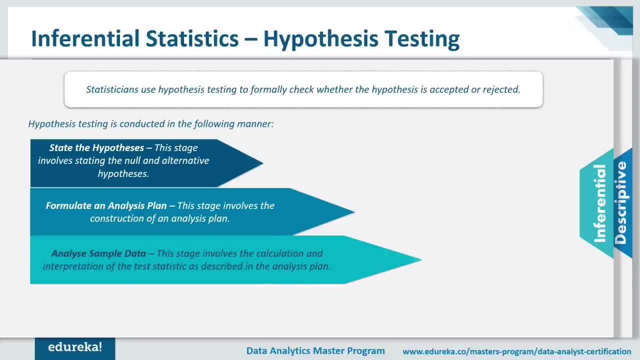 of the analysis plan and then we move on to analyzing the sample data. So in this stage it basically involves the calculation and interpretation of the test statistic as described in the analysis plan that we formulate before, and then they finally interpret the results. where you know, this involves basically the application. 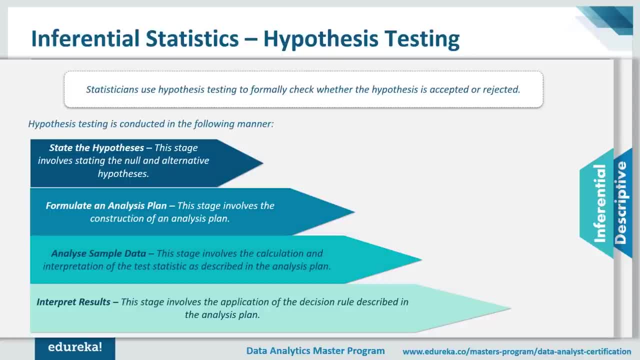 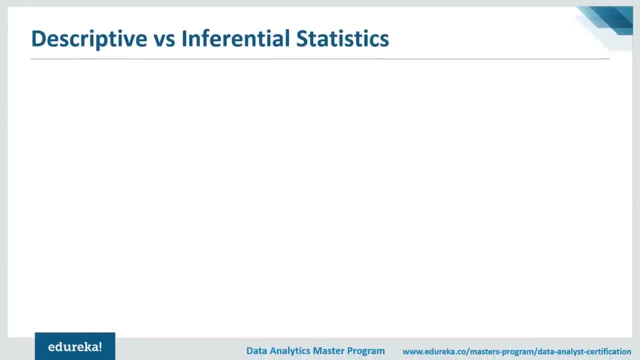 of decision rules described in the analysis plan, right? So, guys, that's how you conduct the hypothesis testing. So, guys, that was all about inferential statistics. So now let me just quickly brush you over the differences between descriptive statistics and inferential statistics. 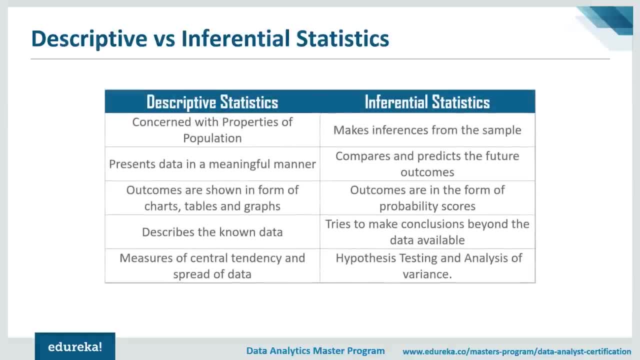 So descriptive statistics is basically concerned with the properties of population, Whereas inferential makes inferences from the sample. descriptive presents the data in a meaningful manner, whereas inferential compares and predicts the future outcomes. descriptive statistics, outcomes are shown in the form of charts, tables and graphs, and inferential statistics. 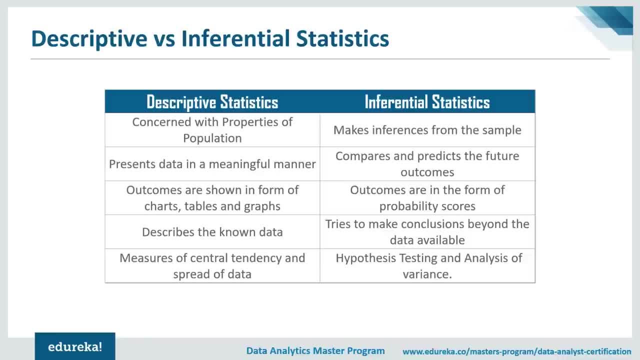 Outcomes are basically shown in the form of probability scores. in descriptive statistics It basically describes the known data, but in inferential statistics it tries to make the conclusions beyond the data as available. and finally, coming to the last difference, descriptive statistics has the measures of central tendency. 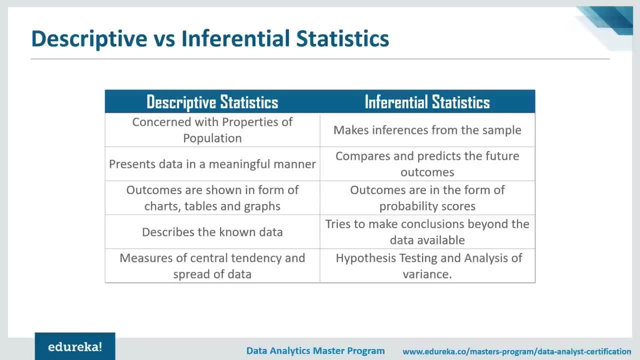 and spread of data, whereas inferential has hypothesis testing and analysis of variance, which is basically the NOA model, right? So I hope, guys, you know the differences between the descriptive and inferential statistics are clear to you, guys. So now let me just quickly move on to the next skill. 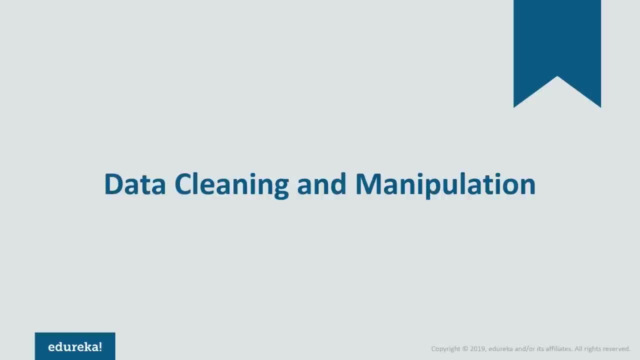 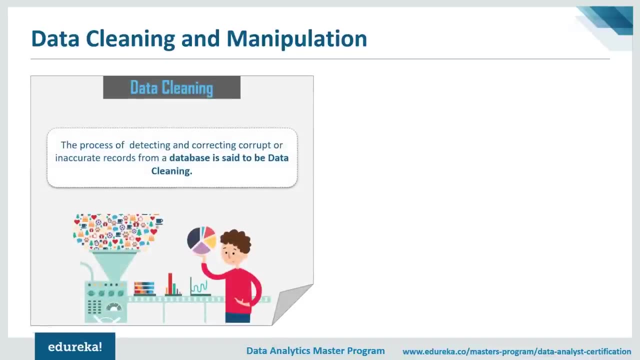 that is important for a data analyst. that is basically data cleaning and data manipulation. So once you get your data, the first step would be to remove all the unwanted data. So the process of detecting and correcting corrupt or inaccurate records from a database is basically said. 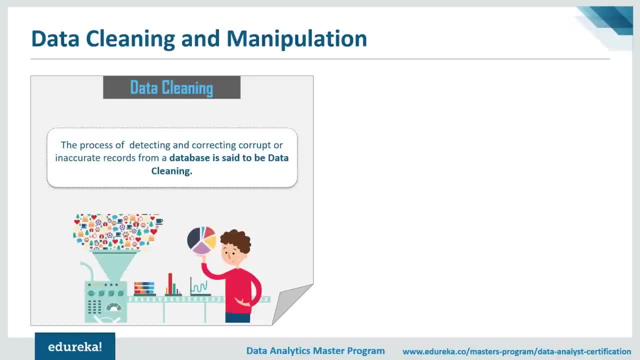 to be data cleaning or data cleansing or data wrangling. So you need to make sure that you know all the null values, the corrupted values or a column from the data removed before you start analyzing the data and once you remove such values from the data. 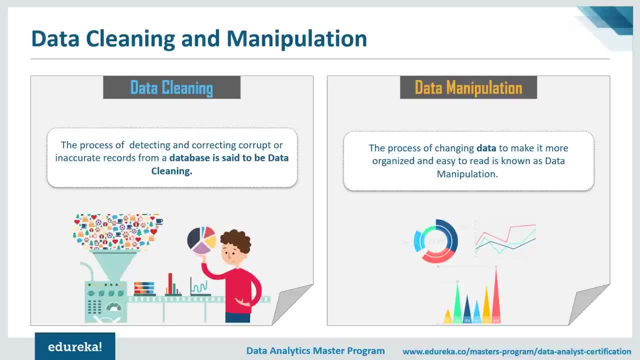 the next step to perform is basically data manipulation, which is nothing but exploratory data analysis. So if I have to just define data manipulation for you, then it's the process of changing data to make it more organized and easier to read, and this is nothing but data manipulation. 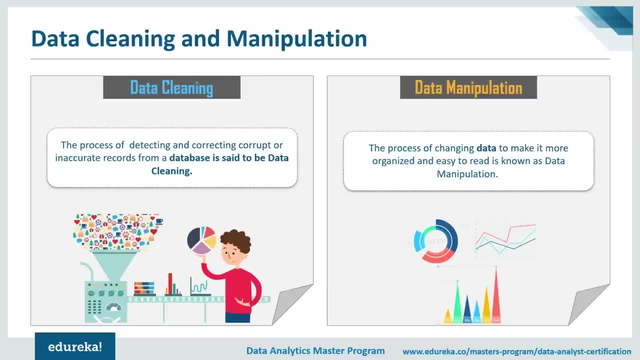 So, whenever you know, you make your data in a more organized manner. you make all the tuples clear and then you have all the column values in a clear manner and it's easy to read and analyze. It's basically known as data manipulation. It's not required that you know. 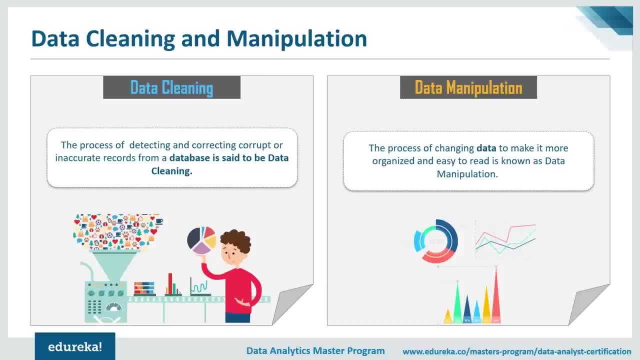 if you have 5,000 tuples, you view all the 5,000 tuples together. You can use some functions to just view the top 10 tuples or the bottom 10 tuples, so that you understand what are the various parameters or what are the columns that are present in the data set. 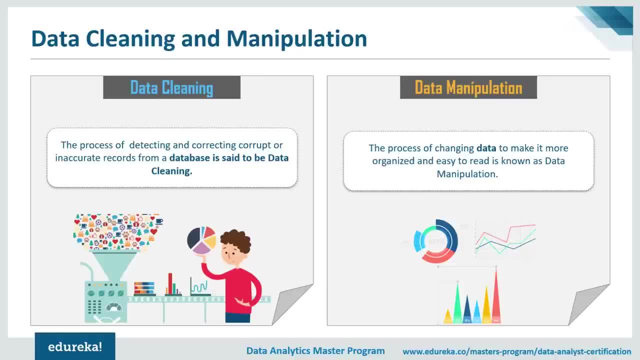 right. So in this particular step, what you can do is you can completely reorganize the data into various forms based on whatever column names that you wish or you know. you can just add few columns or delete few columns. You can remove few tuples. 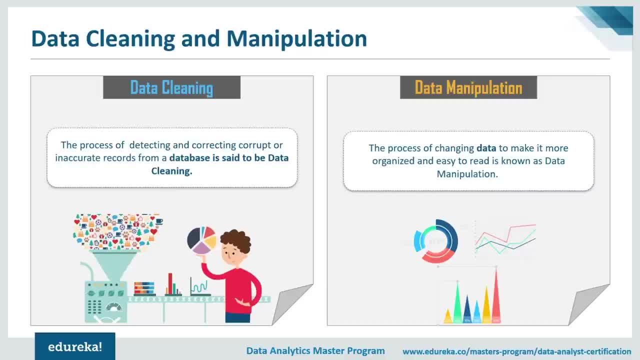 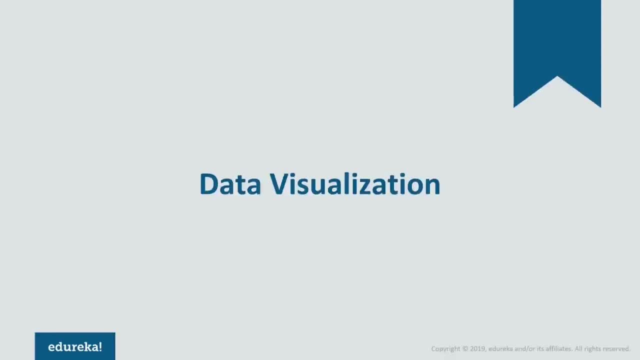 or you can just merge few columns and so on. So don't worry folks, I'll be showing you a demo where you know you will be performing data manipulation. now moving on to the next skill for a data analyst, that is basically data visualization. 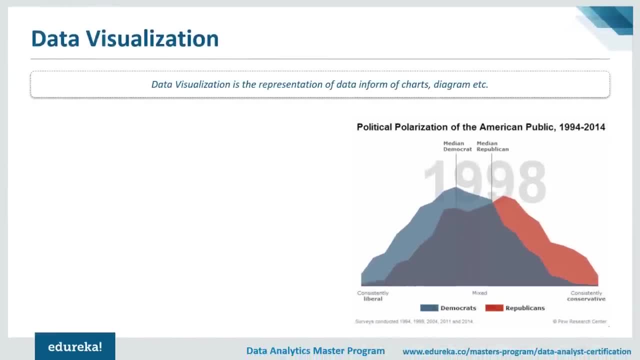 So data visualization is nothing but the representation of data in forms of charts, diagrams, etc. right, So you can represent your data either in the form of bar graphs, scatter plots, pie charts, box plots, line graphs, and so on. not only this, but you know. 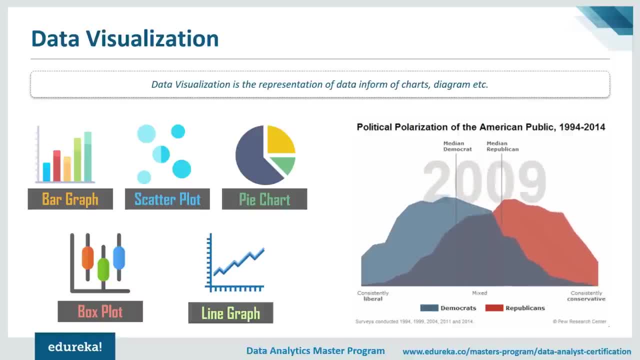 you can also visualize the data in form of complex plots like histograms, and use two to three different plots together. like you know, you can have a scatter plot which has a line graph, or you can have two different plots of you know histograms and then you can have a line graph over it. 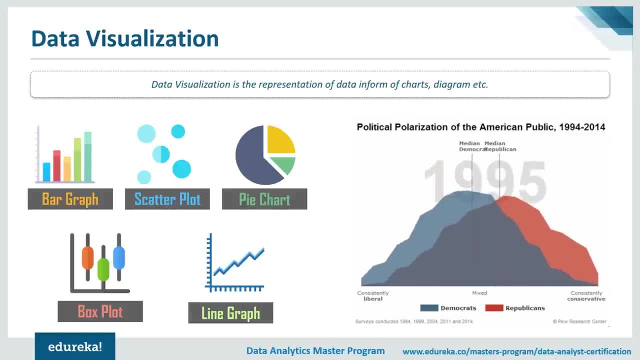 and so on, right? So it's completely based on your understanding of what kind of plot that you want, or it's completely based on you know how you want to see your data or how you want to visualize your data, right? So, guys, these were the basic skills. 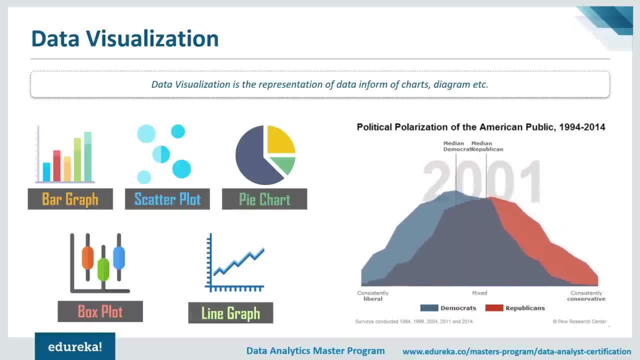 that you know, data analyst must have. we started with statistics and then I told you the various categories of statistics and how you can calculate the various measures in both of them. after that, you know, I told you about data cleaning and data manipulation, which is nothing but the exploratory data analysis. 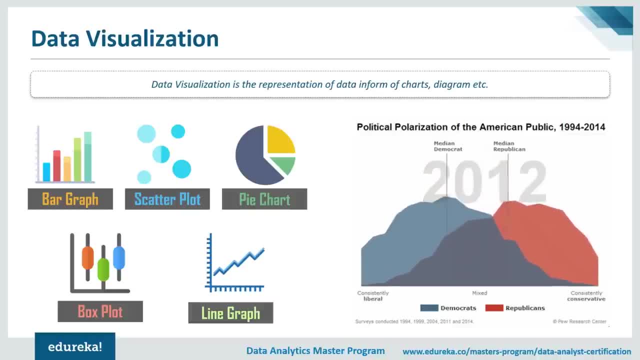 where you clean your data, remove all the null values or the corrupted values, and then you know you can reorganize your data, reorganize your columns. And finally we moved on to data visualization, where you know the columns between which you want to visualize the data. 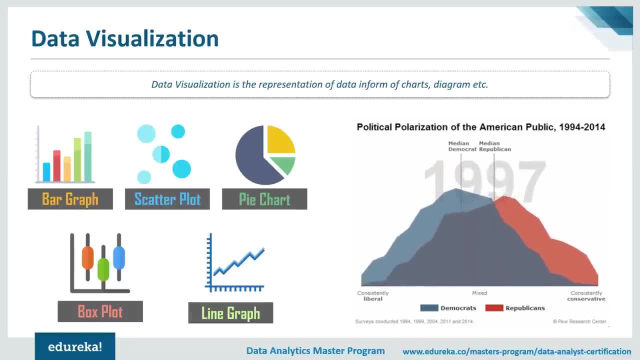 right? So these were some basic skills that every data analyst should have, but, yes, if you have an understanding of machine learning, then that would be obviously a plus point to your skills, right? So now let me just quickly tell you what machine learning is in short. 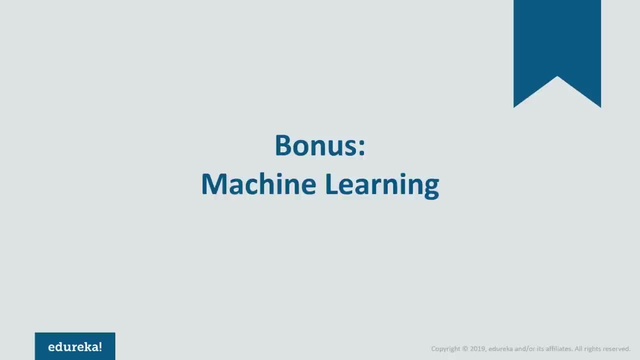 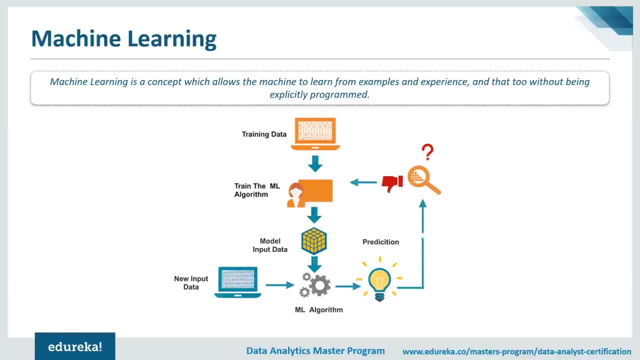 So that you understand what machine learning is, and then we'll quickly shift to the demo part. So well, machine learning is basically a concept which allows the machine to learn from examples and experience, and that, too, without being explicitly programmed. So what basically happens is whatever data. 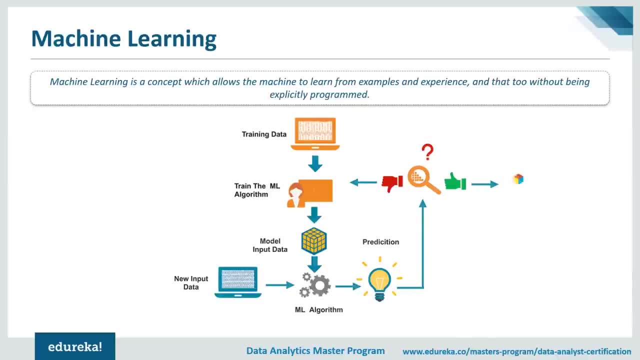 that you pass to the machine learning algorithm. the algorithm learns from the data and then you know it predicts the output for you. So, as you can see on the screen, we have a training data and then the data is passed on to the machine learning algorithm. 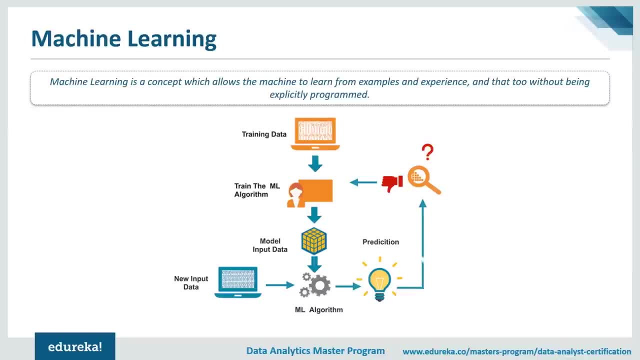 after that, the model is created. now over here, Even if we add a new input data, then that would pass to the machine learning algorithm which was created and a prediction would be given as an output. Now, once the prediction is given, you can just check. 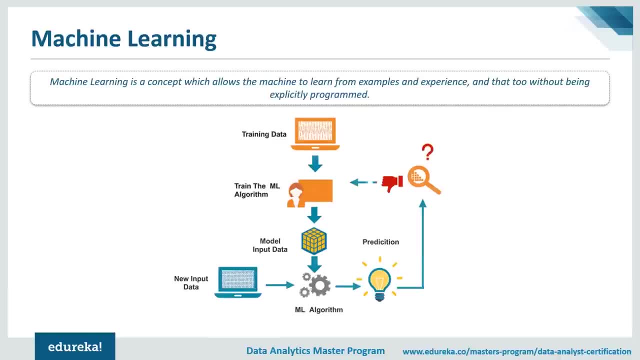 you know whether it's a successful model or not, based on the requirement that you have right. So that's about ml. guys, If you want to learn in depth about ml, I'll leave a video in the description box and you can understand from there what exactly ml is. 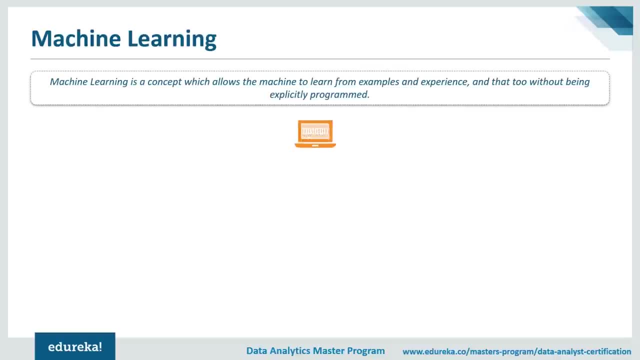 and where is it used, How is it used, What companies are using it, and so on. So, guys, these were all the skills for a data analyst. as I'm talking so much about data analyst, Let me just quickly tell you the roles and responsibilities of a data analyst. 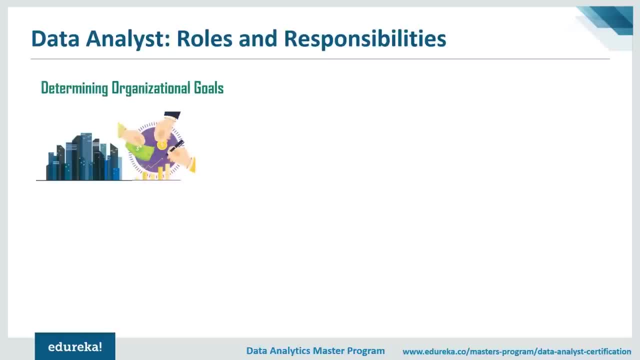 He or she should be able to determine organization goals. He or she should have the capability to mine the data- that is, basically performing data mining and also perform data cleaning. once you know data is being cleaned, he or she should be able to analyze the data properly. 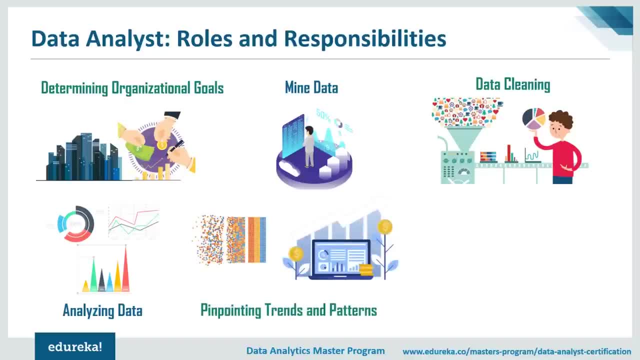 and pinpoint the trends and patterns, or you can say the behavioral patterns, and finally create reports with visualizations, right? So basically, if you become a data analyst, these are the various roles and responsibilities that you would be responsible for. you should be able to determine the organization goals. 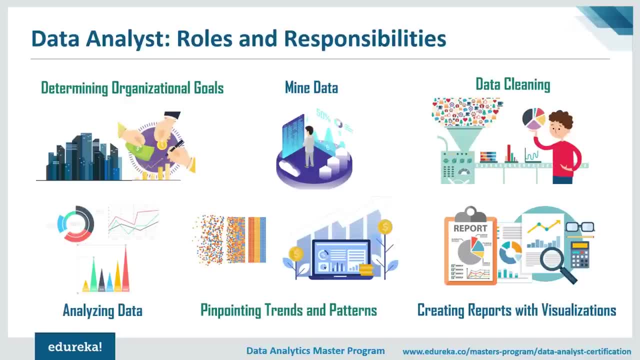 You should be able to mine data. You should be able to perform data cleaning or wrangling. You should be also able to analyze data and pinpoint the trends and patterns in the particular data and finally create the reports with visualization right. So I hope that you know the roles. 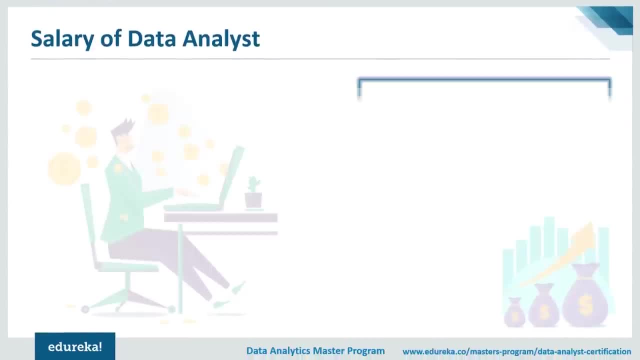 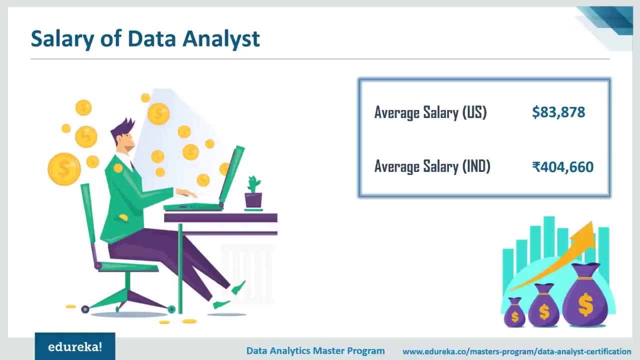 and responsibilities are also clear to you Now. looking at so much of roles and responsibilities, You might be wondering, right, What could be the salary of a data analyst? Well, the average salary for a data analyst in us is around eighty three thousand dollars. 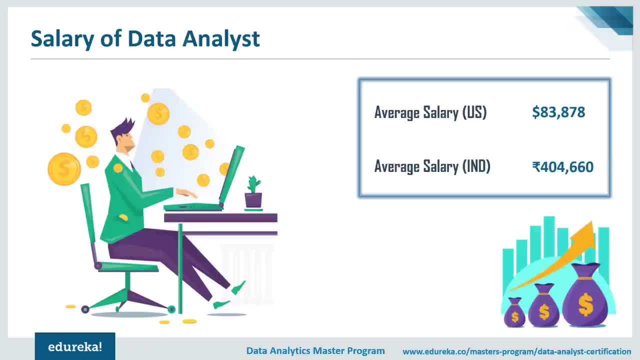 and in India is around four lakhs, right. So, guys, these are the starting salaries, but as and when you know you have a good expertise of data analysis and you're able to perform machine learning algorithms, you would be great in the market. 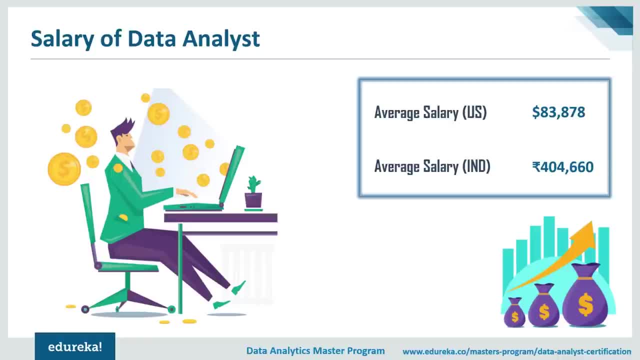 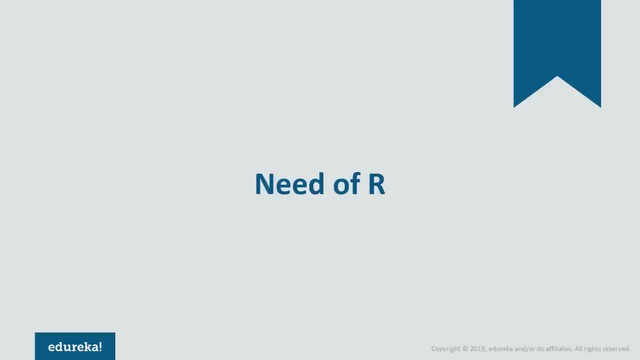 and you would have a great market value right? This was all about the skills, roles, responsibilities of outer data Analyst. now let me just quickly move on to the need of our, because the hands-on that I'm going to show you is based on our. so, basically, our is again a programming language. 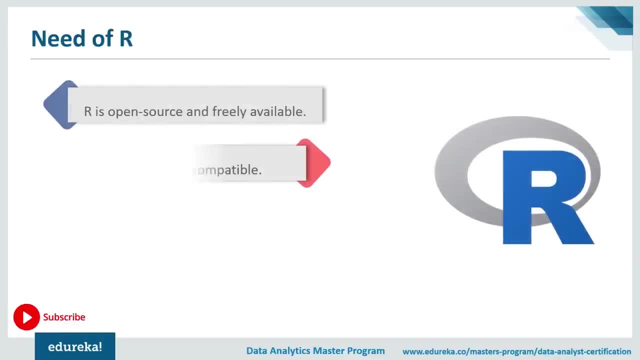 that is basically used for data analytics. So our is basically open source and it's freely available. It is cross-platform compatible. So you know, you can have our with power bi. So, as you know, power bi is a visualization tool. You can create reports using both of these tools together. 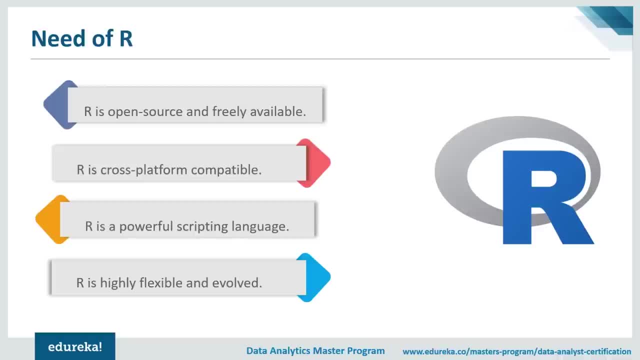 Are. there's also a powerful scripting language. It is highly flexible and is evolved and let me tell you, it's really simple to code and are because you just have to install few packages and then you just have to understand how these packages have various functions to take care of your deeds. 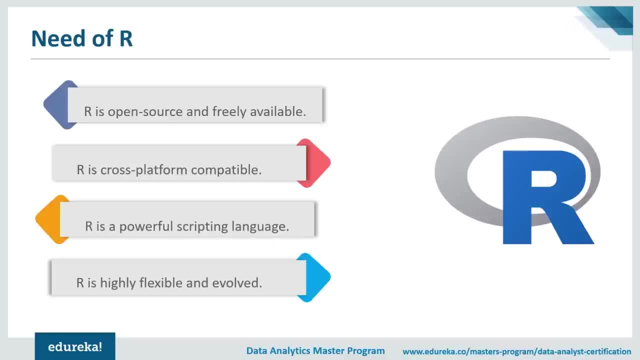 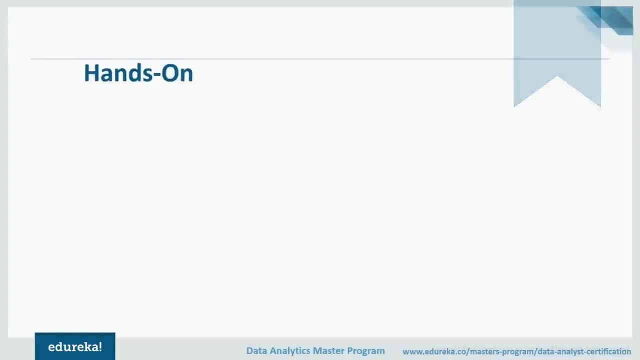 right. So, guys, this was all about the theory part of the session. I hope that you know. you've understood what exactly data analytics is. now Let me just quickly move on to the demo part. So what I've done is I've basically chosen a data set. 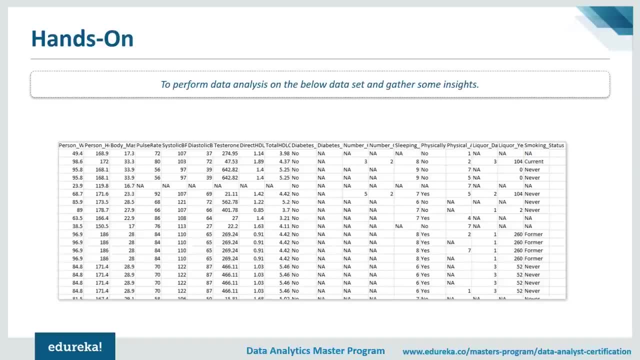 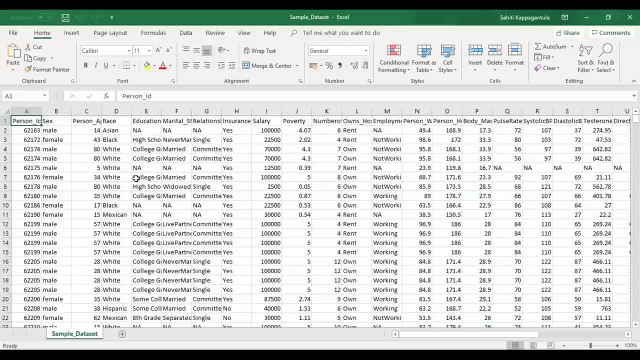 which has various columns like the person weight, the person height, body mass index, pulse rate and so on. So let me just quickly open the data set and show you what exactly the data set is about. So, as you can see on the screen, this is basically the data set that I've chosen. 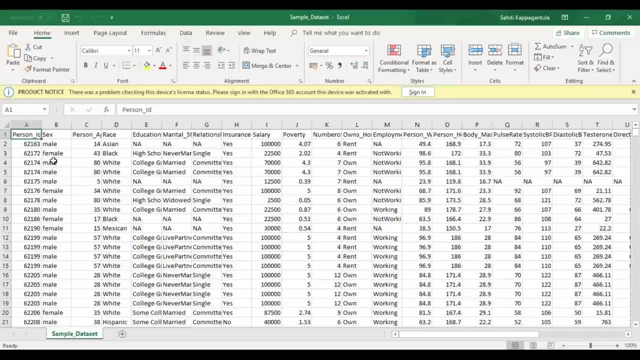 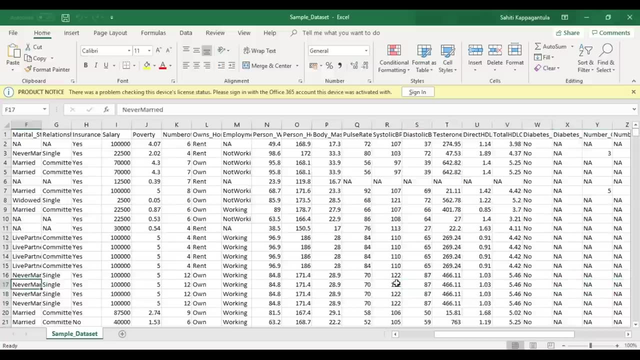 I have a personality, the gender, the person, age, race, education, martial status, the relationship status, and then insurance, salary, poverty, number of house own, if it's rented, the rooms, the person body index, pulse rate and then various other health parameters. right, So we're going to basically perform analysis. 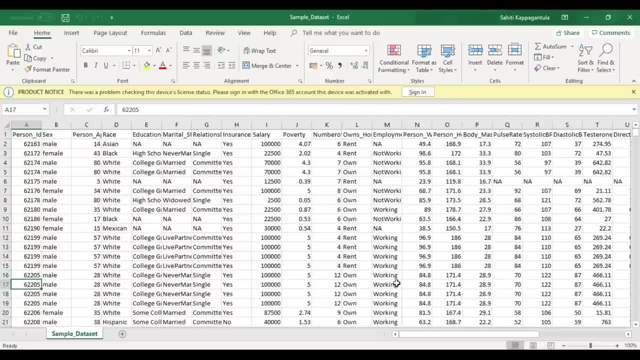 on this particular data. What we're going to do is we're going to first import the data set into our and then we'll perform descriptive statistics on it- that I was talking about in the theory path. after that, We're going to deal with the missing data. 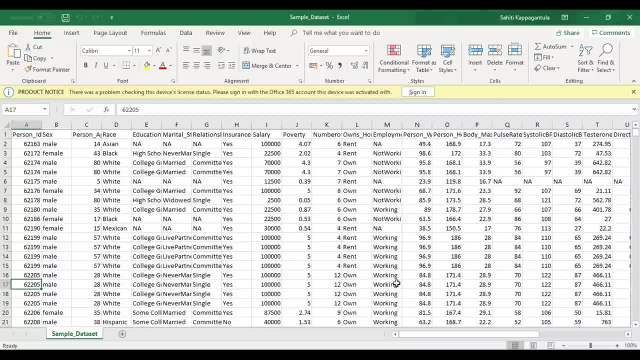 and then we'll perform data visualization. So we'll basically form data visualization between two columns so that you understand how the values in the two columns vary with each other, and then we'll move on to inferential statistics. So you know where I'll perform t-test for you guys after that. 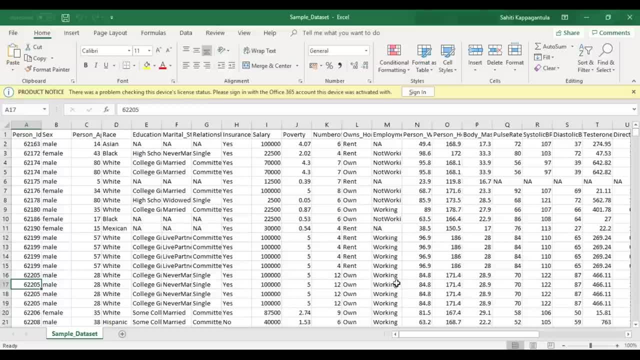 I'm going to just apply a machine learning algorithm, that is, perform linear regression, so that you understand how that's a plus point for a data analyst, right? So I hope that you know the process is really clear to you guys. So let me just open my R student, quickly show you the code. 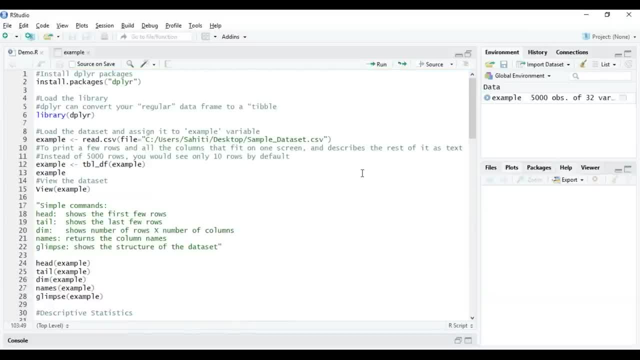 All right. So, as you can see on the screen, this is the code that I've previously written, So I'm just going to show you guys by running each of these command one by one. So the first step that I mentioned is to import the data set. 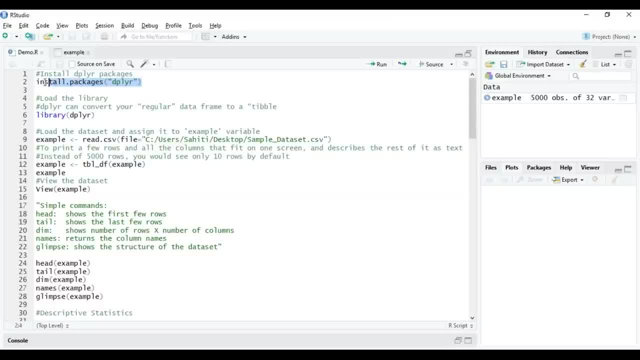 right now. before that, let me tell you that you know we're going to use the deployer package for this complete code. So the deployer package basically offers various functions by which you know we're going to perform various functions on our data set. 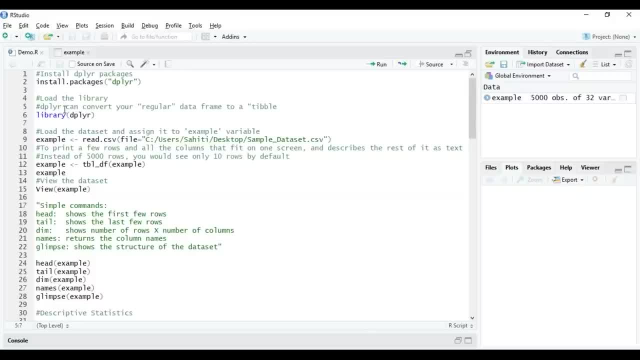 So you can just install this package if you don't have it installed on your R studio. but yes, if you do have it installed, you just have to use the library, right? So I've already installed in my R studio, So I'm not going to do that again. 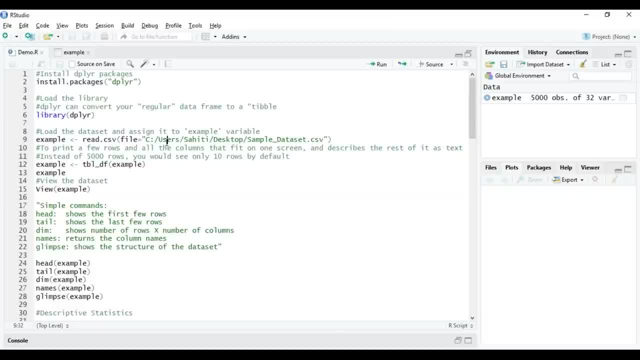 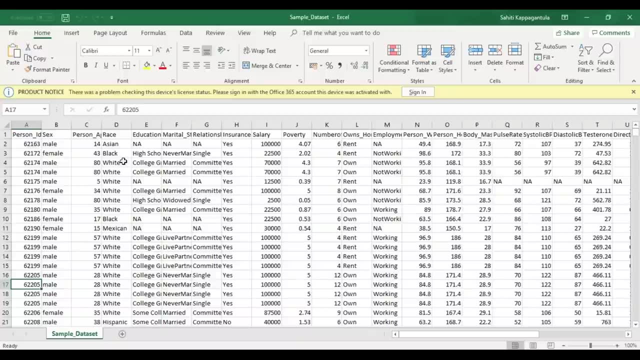 Now what I'll do is I'll just import the data set directly. So to import the data set you have to mention the readcsv file. That's because you know my sample data set is in the form of a CSV file, or, if you had any other types of file. 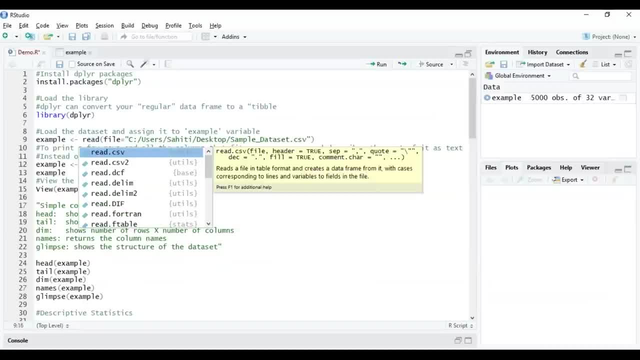 then you have to mention accordingly. Okay, So if you just type in read, you can see various options for various kinds of files. So since I have a CSV file, I'm just going to type in CSV, right, and then what I've done is I've mentioned the directory. 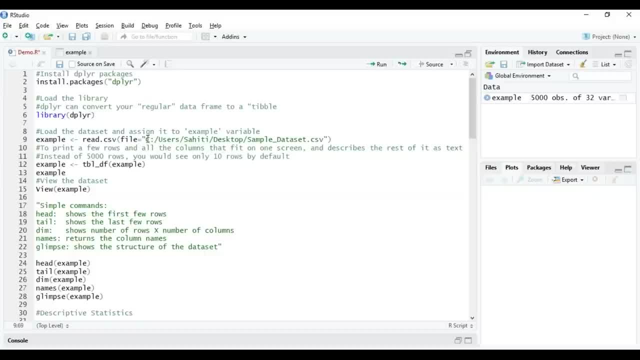 of the file, right? So since my file is present on desktop, I've just mentioned the directory and then I can just execute this particular command. But yes, let me tell you once the file is read. what I've done is I've just assigned it to a variable example over here. 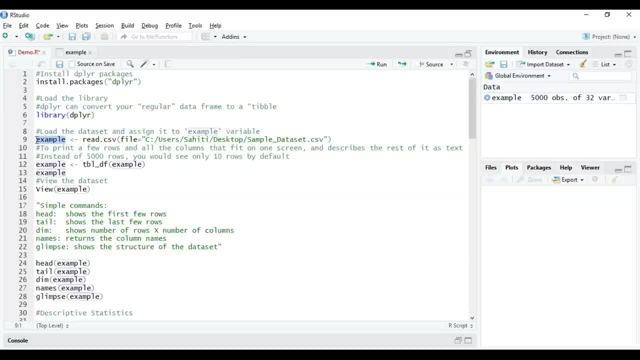 that will basically make it easy for me to use this variable again and again to perform various steps in the analyzing part. I've just assigned this complete file to a example. Now let me just run this particular command. So what I'm going to do is I'm going to just press on control- enter. 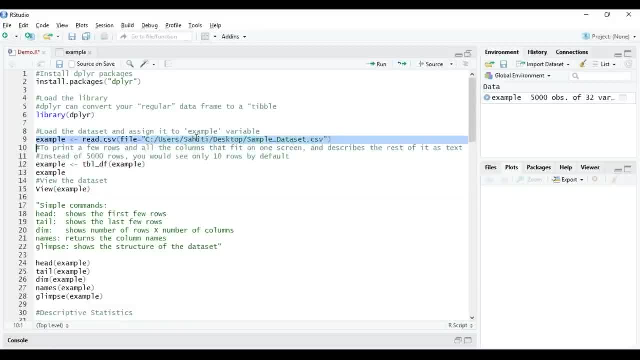 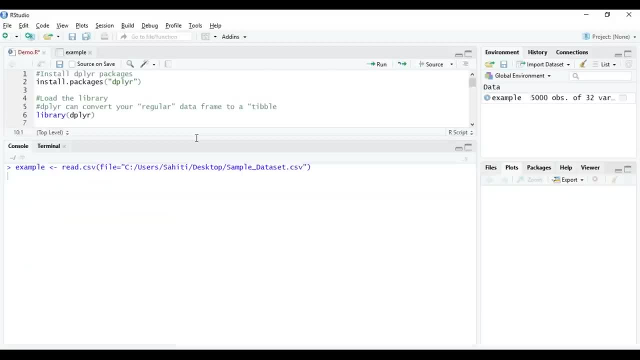 So that's basically a keyboard shortcut to run this particular line. If you just want to run the complete R script that you've written, then you can just press on control shift, enter, right? So I'm just going to press on control enter and you can see that you know. 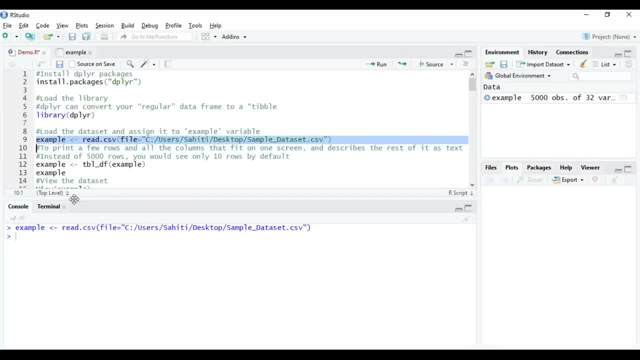 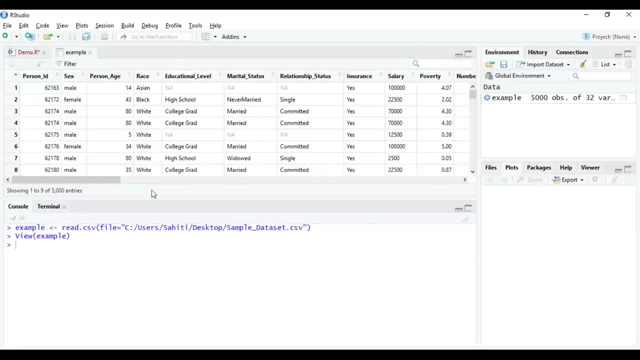 this particular command has got executed. Now, if you just want to view the data set, what you can simply do is you can just use the command view example, and then you can click on run and you can see that you know your complete data Set. that is basically your sample data set. 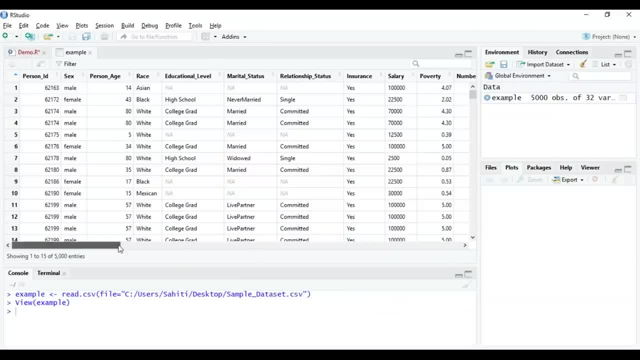 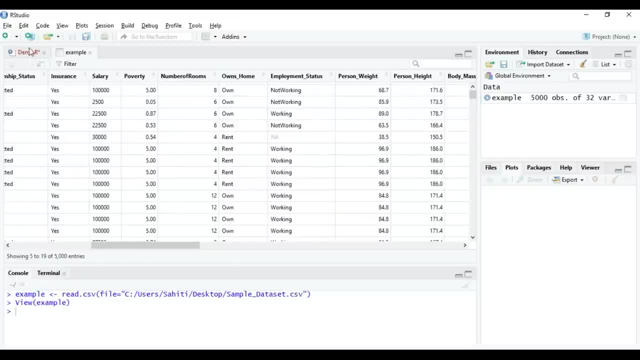 which was present over here, has got imported into the R studio where you can perform various analysis functions right, So you can see all the columns and all the values have come over here right now. If you observe this particular data set, you have 5,000 entries. 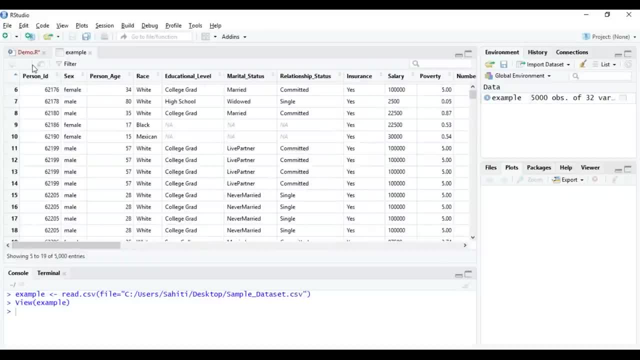 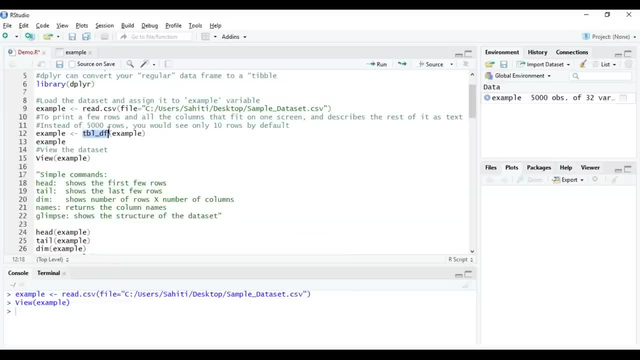 right now. it cannot happen that. you know, you observe 5,000 entries in your console, right So to just observe the top 10 entries. what you can simply do is you can use this function, tbl, hyphen DF. that is basically creating a data. 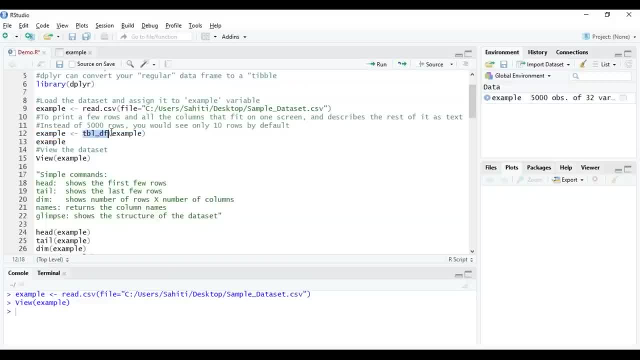 frame for your data set. So what I'll do is I'll just type in tbl DF, I'll mention this variable name- that is basically example over here- and then I'll again assign it back to example, right? So if I just run this particular command, 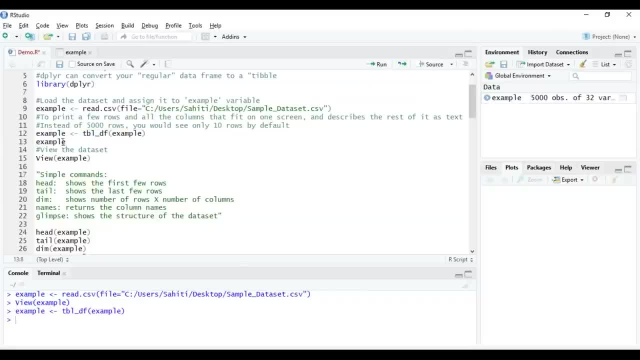 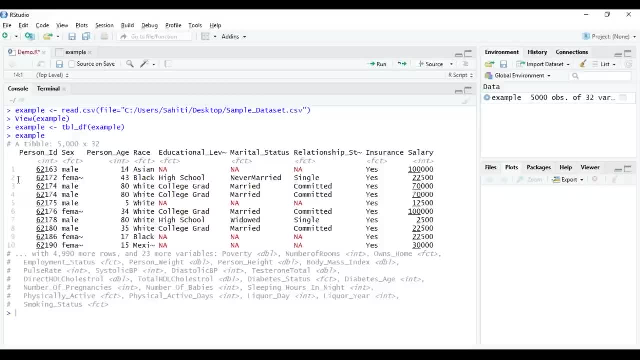 you can see that you know this gets executed. and then, if I just type in example, you will see that you know only 10 rows get printed. So let me just drag this up for you. You can see that you know we have 10 rows printed to check all the values. 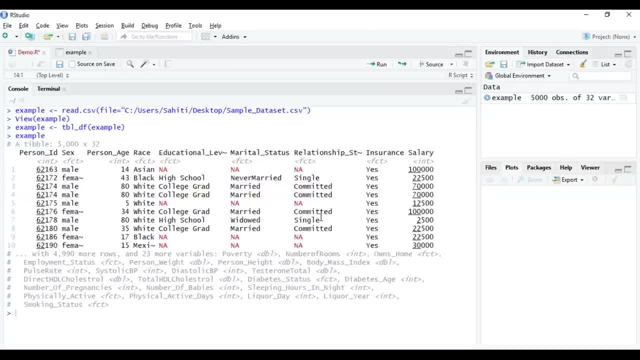 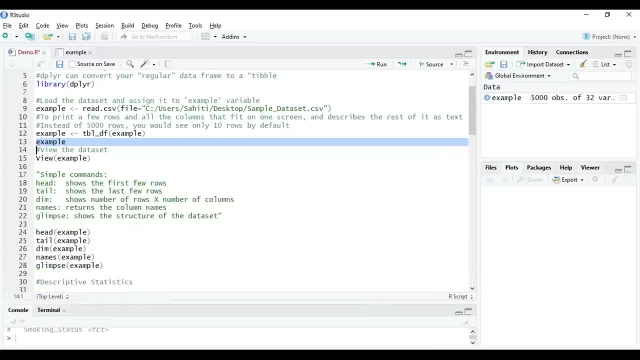 and we also have a table that is basically 5,000 into 32, which says that you know, we have 32 columns and 5,000 entries, right? So that's how, guys, you can use this particular function to see the top 10 rows. 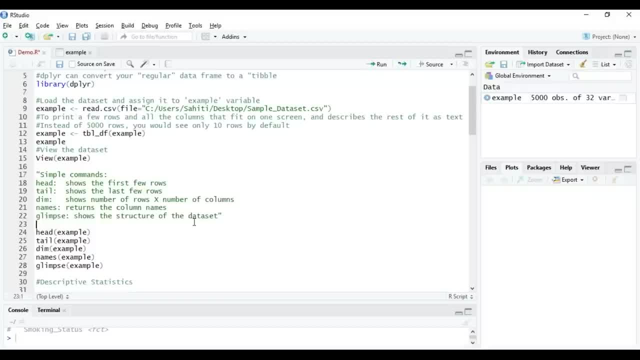 Now what we're going to do is we're going to just use simple commands like head, tail, dimension names and limbs to just look into the data set more clearly. So what the head function does is that it basically shows the first few rows. the tail, as the name suggests, shows 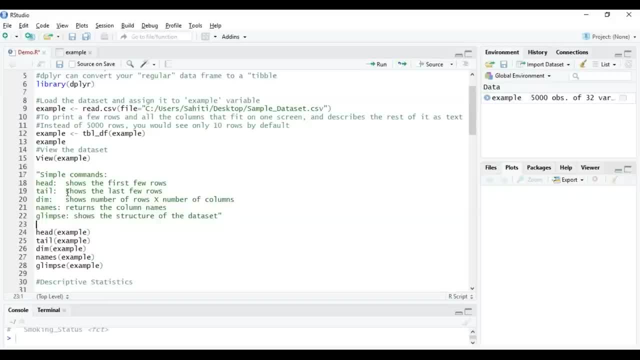 the last few rows. the dimension shows the number of rows into number of columns. So just in case, if you just want to look into the names of the columns, then you can just use names and glimpse basically shows the structure of the data set. So I'm going to first run head so that you see few rows. 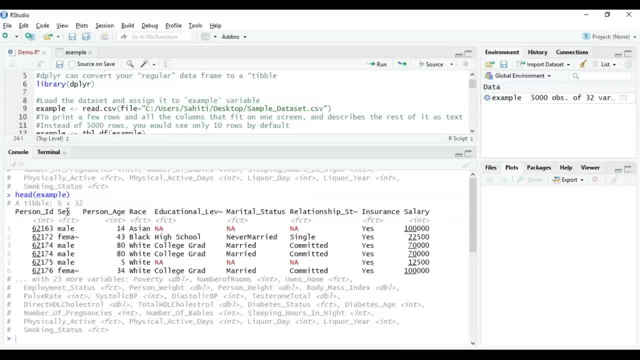 So, as you can see, you know it has printed six rows and it is printed around one, two, three, four, five, six, seven, eight columns, right. So it has printed six rows and eight columns and it has also mentioned that. you know. 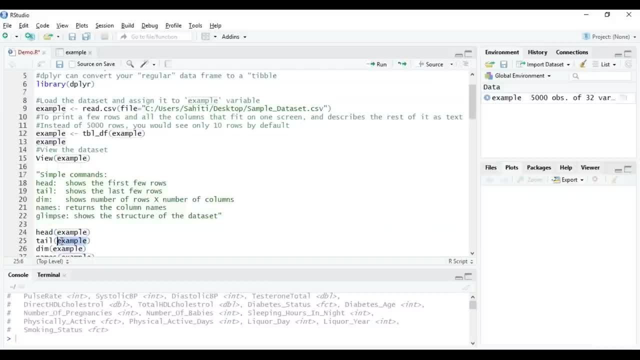 there are total around 32 columns Now. similarly, if I'd run tail, then you can see that you know the last few rows are printed. So these are few last rows of the data set that we have chosen. Now, moving on to the next command, that is, dimension. 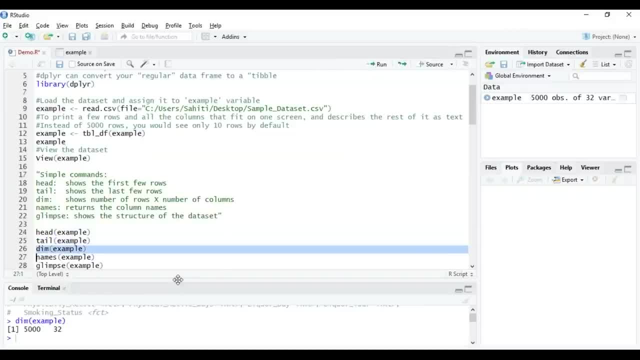 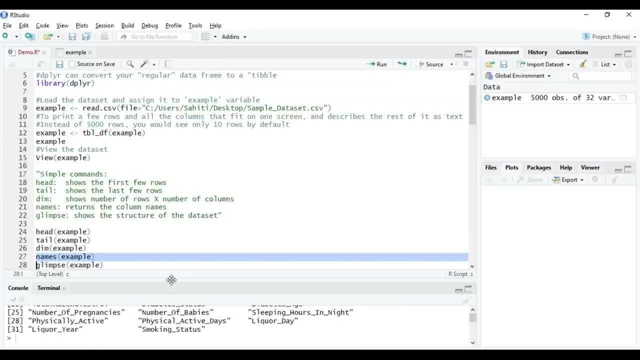 So, as I mentioned, dimension will basically give you the number of rows into number of columns, So that is basically 5000 into 32. now names would be basically giving us the column name. So I'll just run in names and you can see the 32 column names. 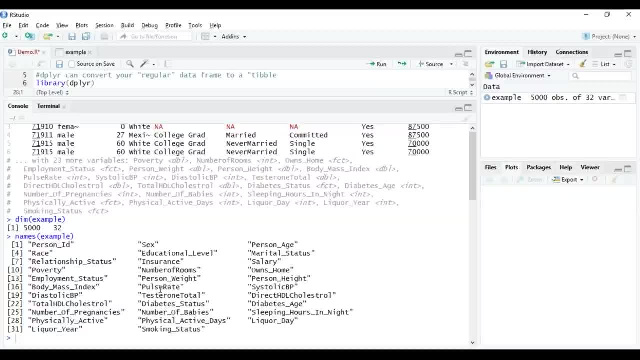 that we have. this will basically help you understand What are the different column names and what are the different columns names that you can use to find the relations between the values. So we have an ID, sex, age, race, education level, status, relations of status, insurance. 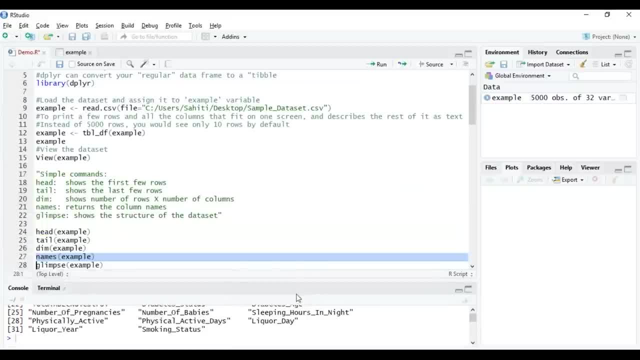 And so on. right, So these are few steps, guys, that are not really important, But, yes, these will help you understand the data set more if you're new to data analytics, because you know you have to start understanding if there are any null values. 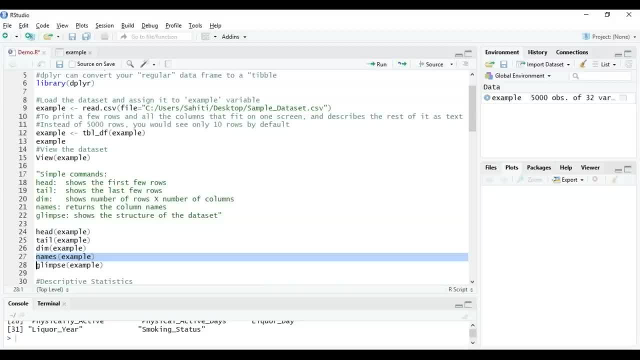 or you know what are the number of rows or what are the columns if you have larger number of rows. like you know, if you have around 50,000 tuples, then you cannot use 50,000 tuples to run each function right. that would require a lot. 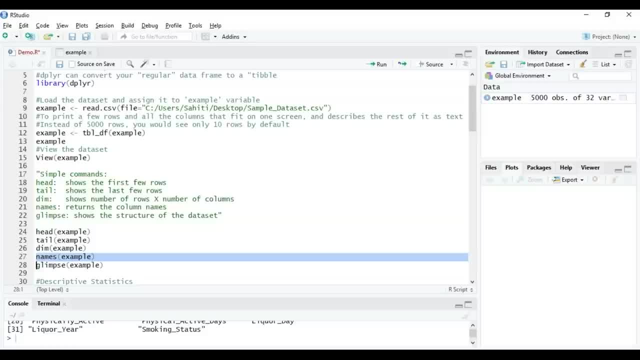 of memory. So for that you can just use a sample data set. like you know, you can just use 5000 rows And then you can use the built model for the 50000 one right now. moving on to glimpse: glimpse again just shows the structure. 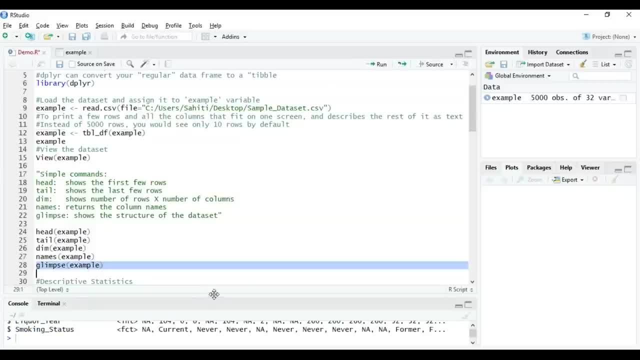 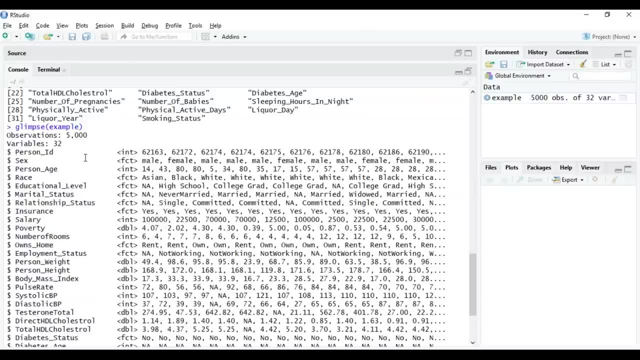 of the data set, as I mentioned before. So let me just run that command and show you so as you can see, it is printing out all the column names and then it is printing out all the values. So you can see that in the person ID is an integer. sex is: 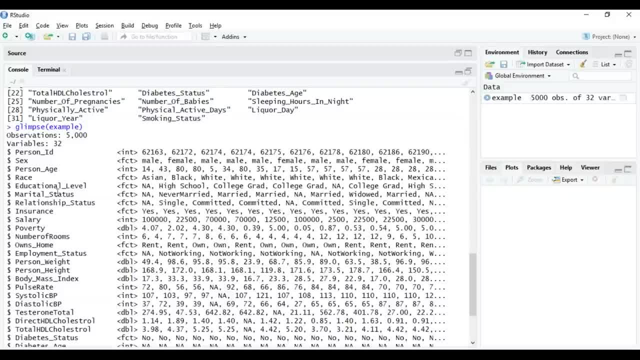 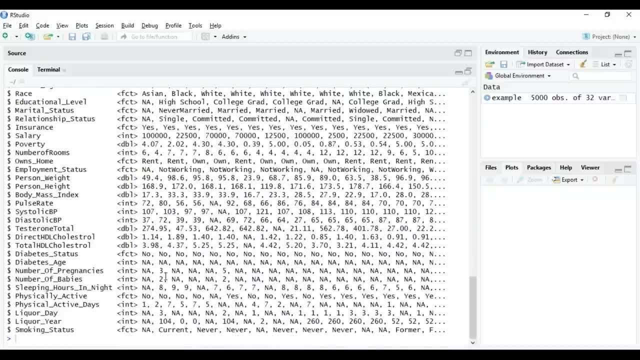 in factor and has male, female values. age is again an integer race is again in factor, poverty is again in decimal points, and so on. right, So you'll know the data type, you know what kind of values are present over there, and then you can. 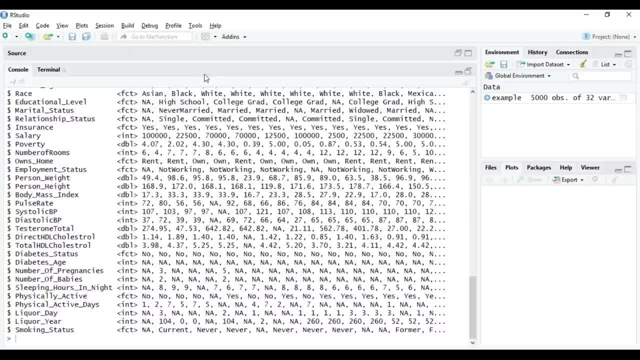 also know. and what are the columns which have different kind of values, right? If you observe over here, there are a lot of any values, right? So we're going to deal with them soon. So don't worry now. Let me just minimize it again. 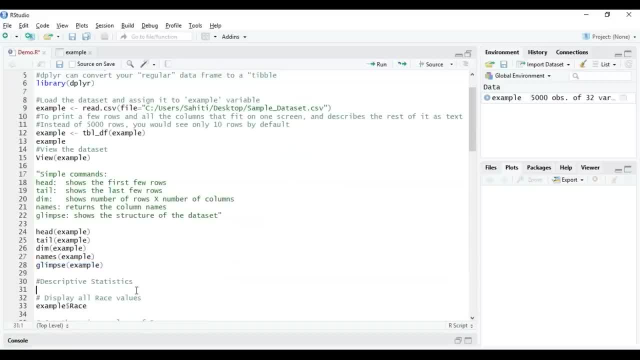 All right. So now that you know the basic commands in our you know how you can start for analyzing the data. Let's start with the second step, that is, the descriptive statistics. So if you remember, in the descriptive statistics part I told you that 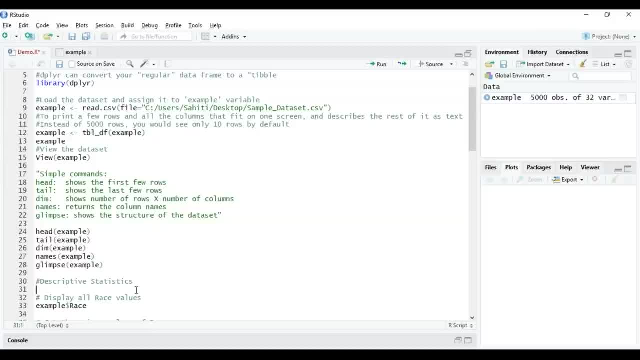 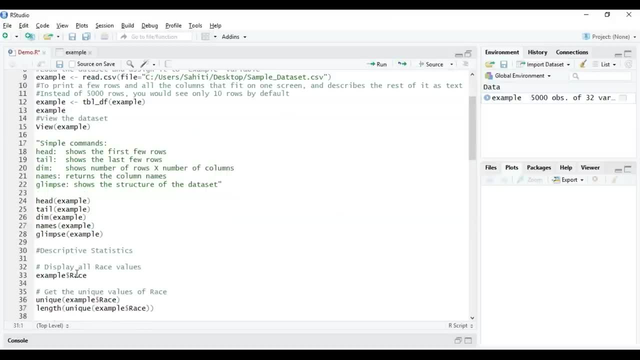 you know, there's measure of Center, which has mean median mode, and there is measure of spread, which has interquartile range, Quartile range, and so on. right, So what I'm going to basically do is first I'm going to display all the race values and then I'm going to display the unique 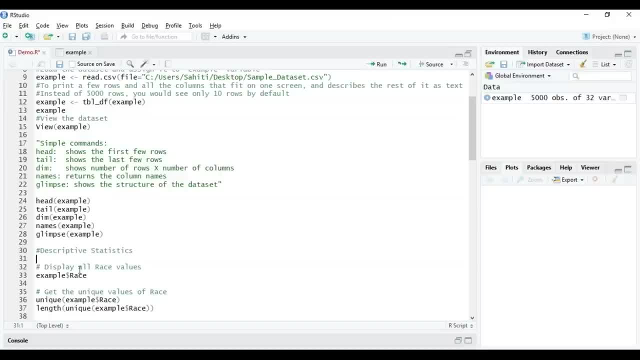 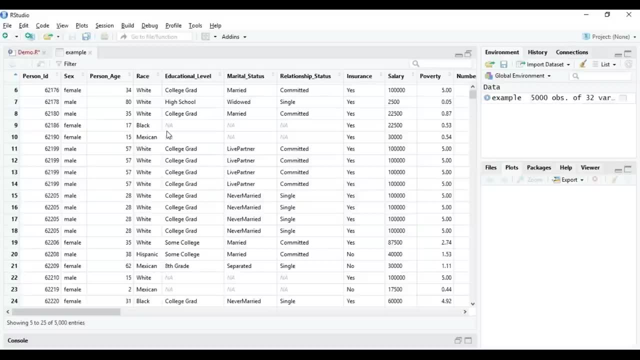 values of race and the length, right so to display all the race values. if you see, over here in the column we have different race, We have Asian, we have black, we have white, we have Mexican and so on. right now to display all these race values, what you? 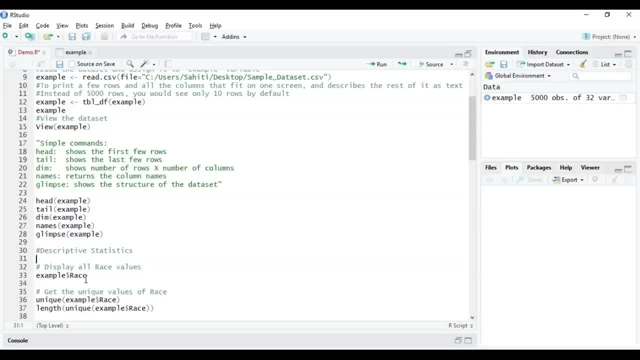 simply have to do is you have to use the variable for the data set- that is example, and use the dollar sign with the name of the column right. So over here it's example: dollar race. I'll just run this particular command and you can see the. 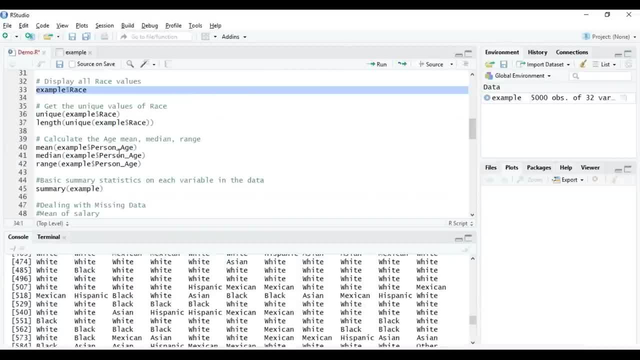 output that you know. we have got all the race values. Now, if you want to find out the unique values, what I'll simply do is I'll use the unique function and then I'll mention, example, dollar race. Similarly, if we want to find out the unique values for any 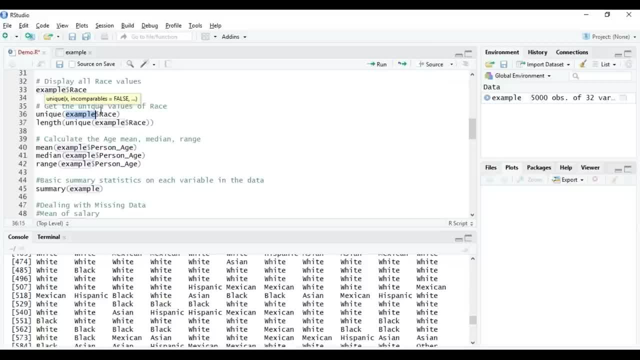 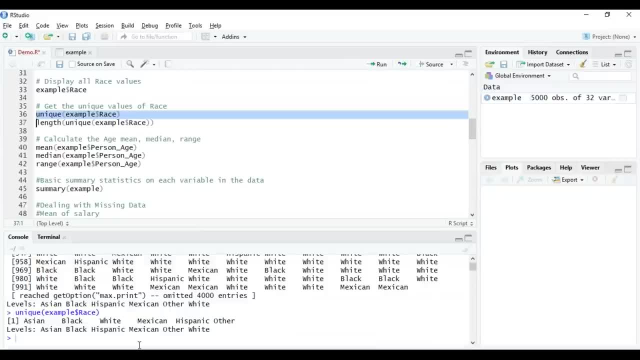 other particular column. we just have to mention that particular columns name over here. I'll mention unique example race and then I'll run and you can see that. you know we have Asian, black, white, Mexican, Hispanic, other, as various races present in the column right now. if you want to find. 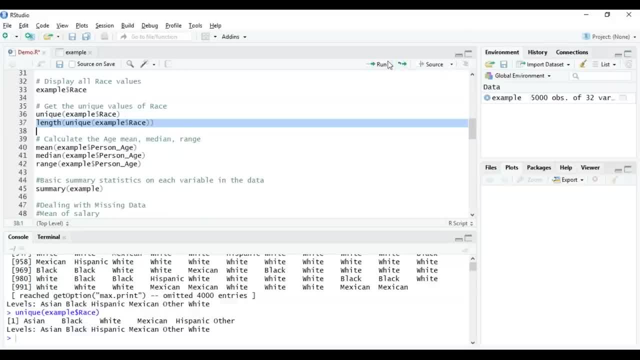 out the length of all these unique values. you just have to use the length function outside the unique function and then you have to run this particular query and you can see that you know the length is basically six. So basically, what's happening is, instead of counting Asian, 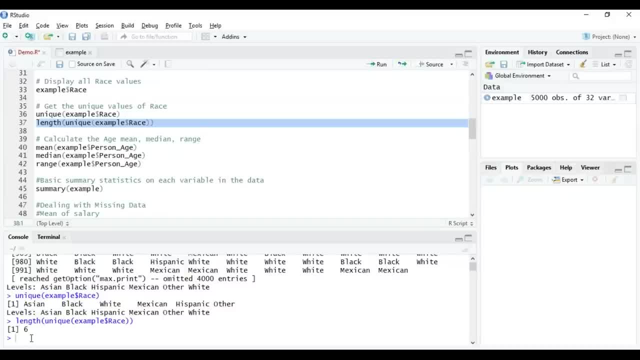 black, white, Mexican, Hispanic and other on fingers. What you can simply do is you just have to use the length function to find out How many unique values are present in the race column right. So that's how you can use the length function. guys, now moving. 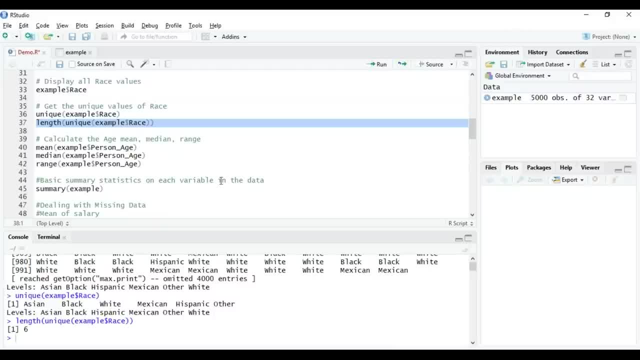 on to the next part. If you just want to calculate the mean median and range of any particular column, let's say age over here, What you simply have to do is you have to use the inbuilt functions in our, that is, the mean median range, and then you. 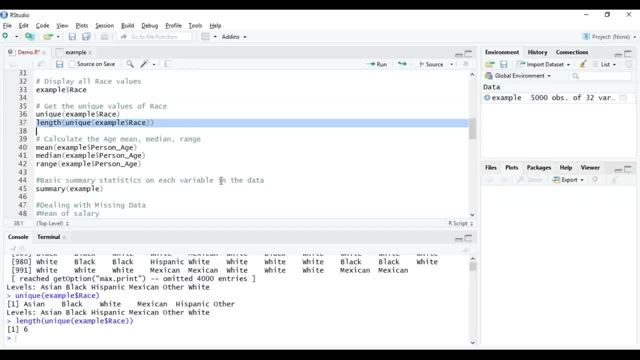 have to mention the variable name dollar and the column name, right? So if you have to calculate the mean, what you'll simply do is you'll type in mean and then you'll mention the variable name. that is example for the data set: mention dollar. that is. 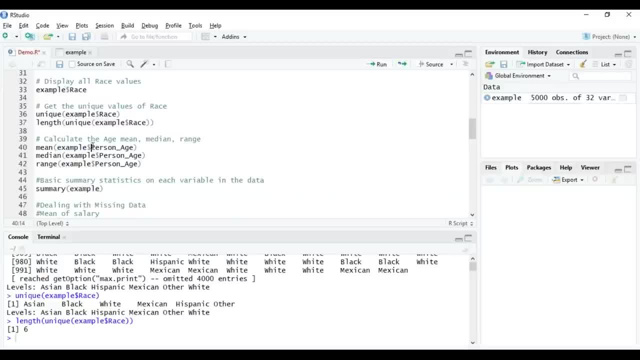 to Specifically access this particular column, that is, to specifically access the column age, right? So I just run this particular command and then you can see that you know, 36 is basically the mean age. Similarly you can calculate the median median is also 36. 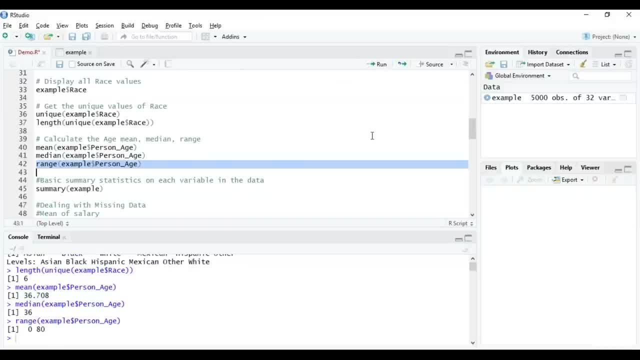 and the range is basically from 0 to 80. So that's how, guys, you can use descriptive statistics and are to find out the mean, median and reach. now, if you just want to get a summary statistics on each variable in the data, you can just use the function summary and then you have to. 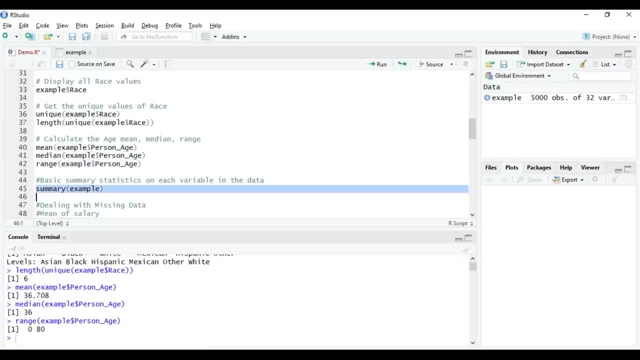 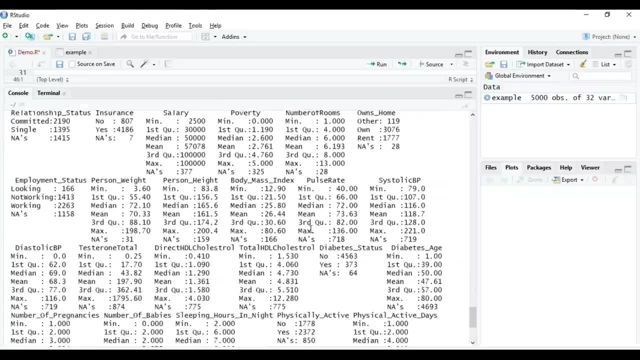 mention the variable name, right? So I've mentioned summary example And then if I run this particular command you can clearly see that you know we've got summary of all the 32 columns that we have in our data set. So when I run this particular command, 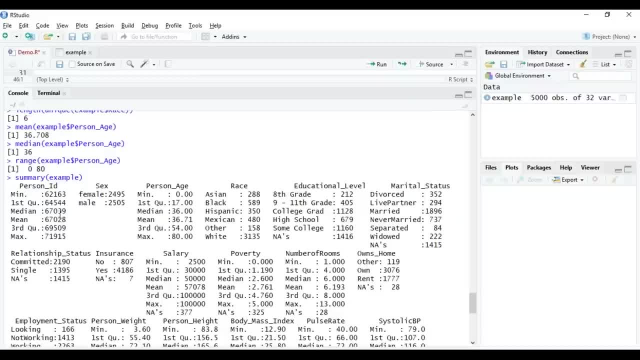 you can see that you know for all the columns with the data type and you get the minimum value, the first quadrant, the median, the mean, the third quadrant and the maximum value for the columns which have the data type factor, like, for example, sex. We have number of females to be 2495 and number of menials. 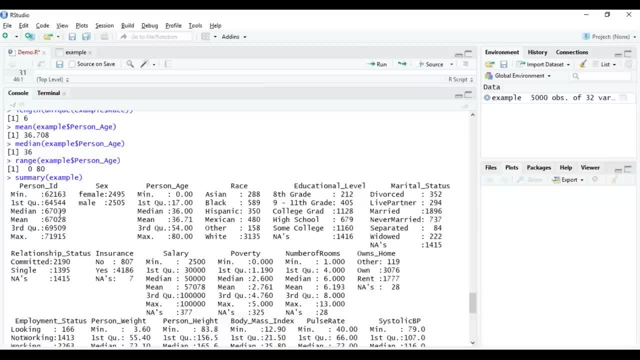 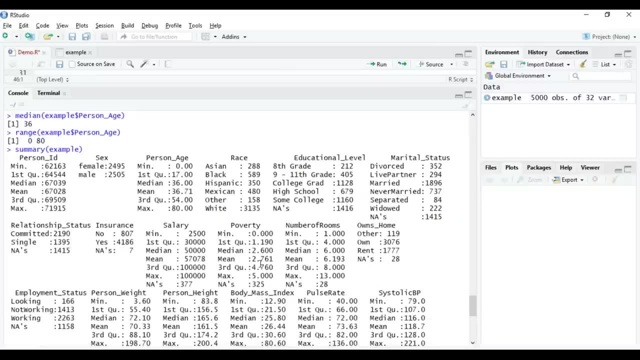 To be 2505. and similarly, when we see for race, we can see that. you know, the Asians are at 288, the blacks are at 589, and so on. Right, So that's how you can have an idea about you know. 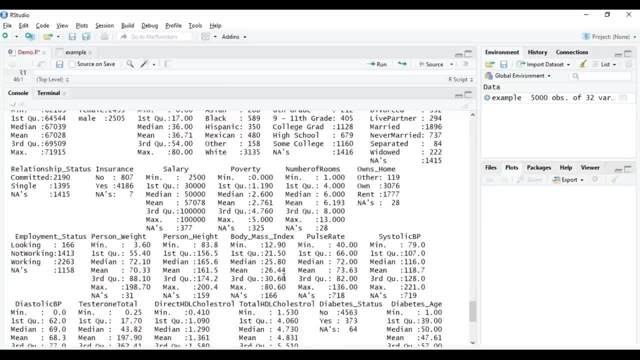 different values present for your data set, So you can get the number of values, the minimum, the medium, What are the various kind of values that are present in the column, and so on, with this particular function. that is summary right. So this is also one particular important feature that you need. 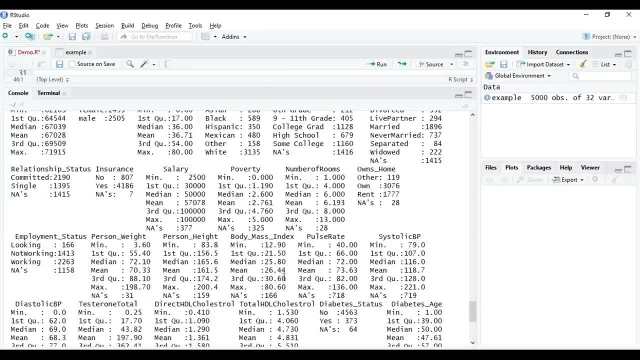 to analyze. in any data set that you get to handle to, you have Have to understand what are the various factors, or you know what are the various types of values that are present in your columns and what is the number of those values right. 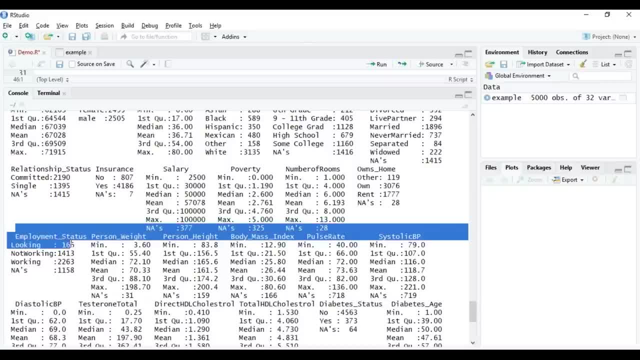 So if I look into the employment status, you can clearly see that you know, the looking is 166.. The not working is 1413.. The working is that highest, that is, 2263, and not applicable, That means it's null values. 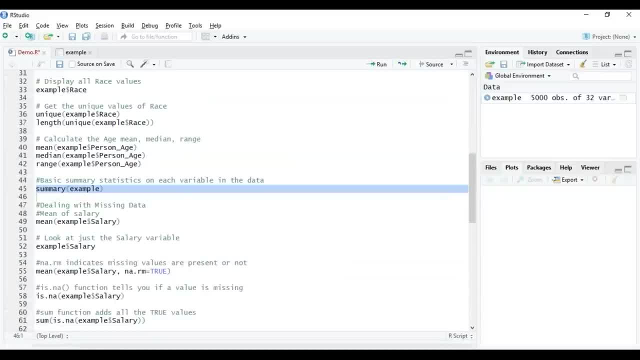 It is at one, one, five, eight right. So these are various features that you need to understand. now that you know you have implemented descriptive statistics, Let's move on to the third step, that is basically dealing with the missing data. So to deal with the missing data first, 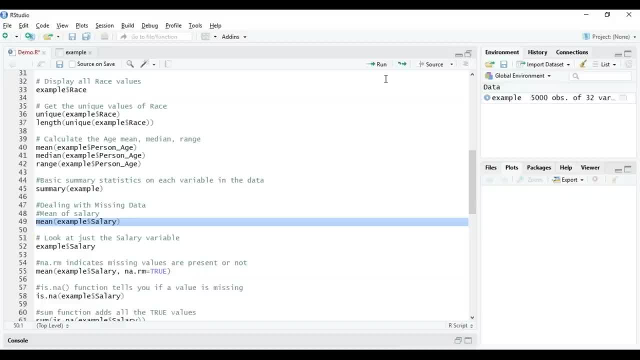 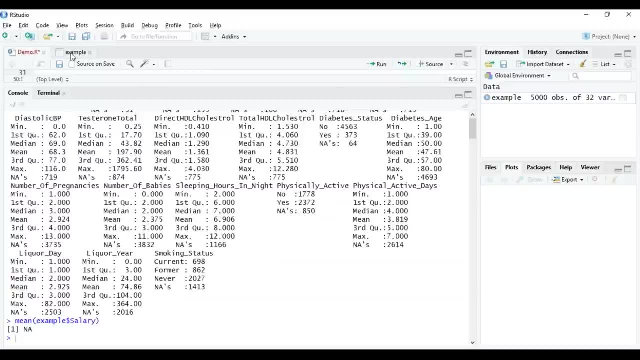 let me just calculate the mean of the salary and then I'll explain you why we have to deal with the missing data. So when I calculate the mean of the salary you'll see any. now if I just open my data set and if I show you the salary column. 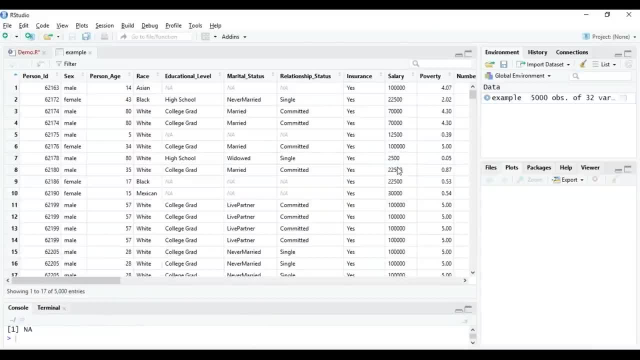 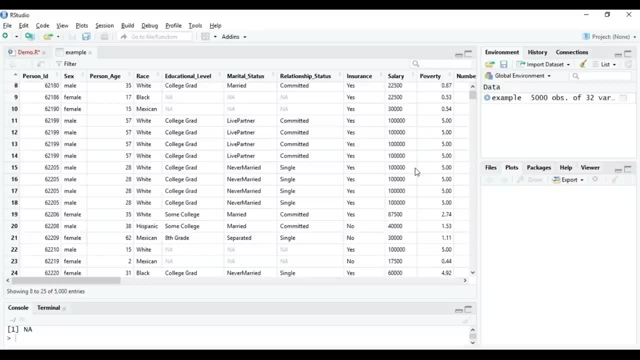 you'll see that. you know you have various columns which are not any right, But yes, we've got the output as any. that means it's definitely wrong. You need to get the mean of the income Now, since we have a lot of columns that could be. 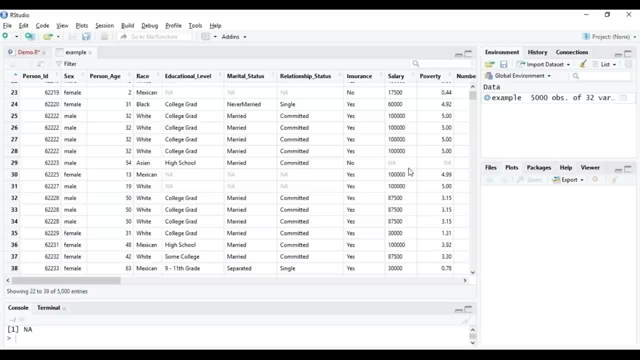 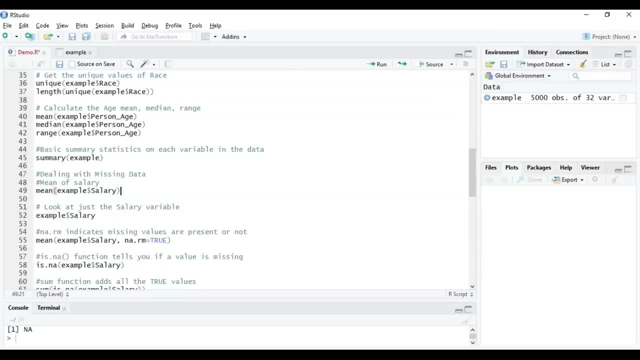 any in this particular column. that is the reason that you know we're getting the output as any right. So what we can simply do is we can just find out, you know, whether there are missing values or not here. I had showed you because the missing value occurred at the 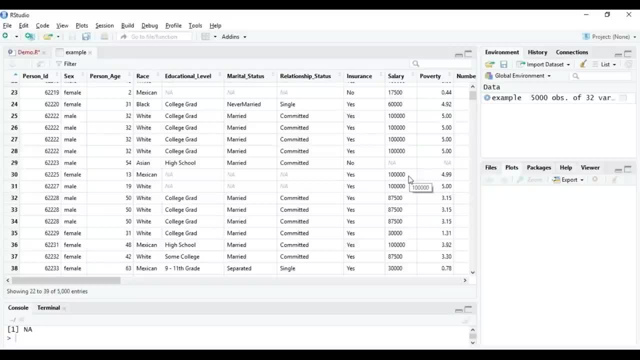 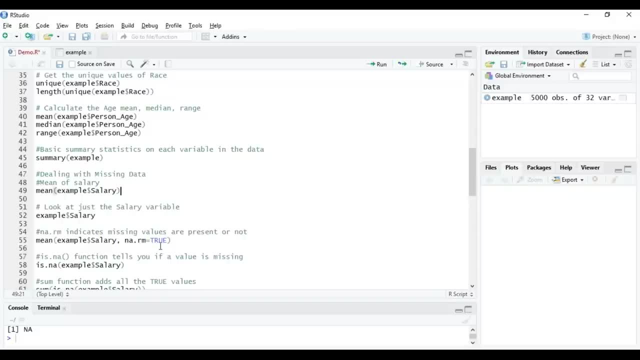 29th couple itself right. But just imagine, you know you have 5,000 couples and you don't know where is the any value coming. You need a way to find out that right? So that's by using the any dot RM parameter. 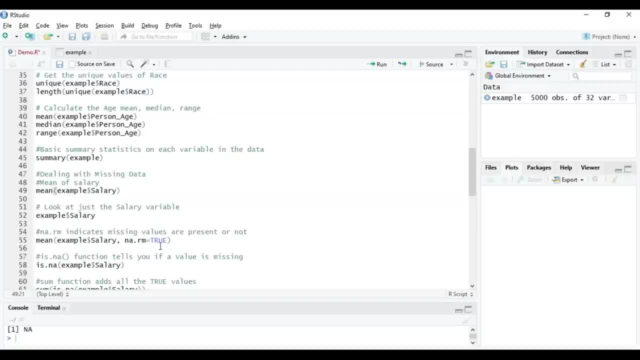 So any dot RM basically indicates if you know whether there are missing values present or not. by default, this parameter is assigned to false, But yes, I'm mentioning it over to be true so that you know whether, if we have any missing values. 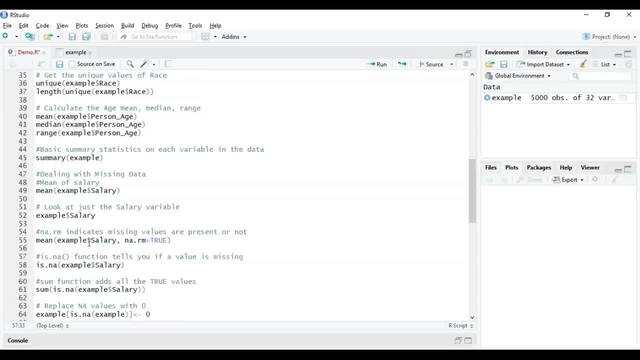 then this would return an output for us. So with this particular command you can see that. you know if the example data set salary has any null values- that is basically true over here- then obviously we can calculate the number of null values present. 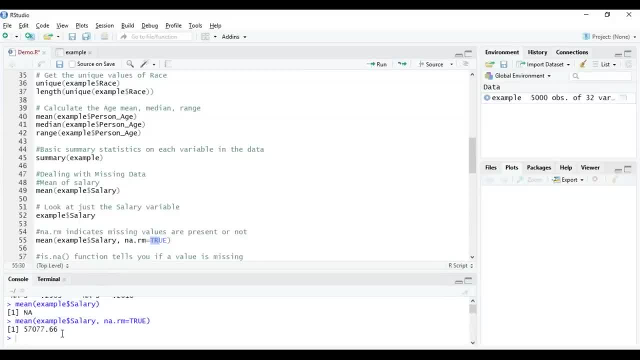 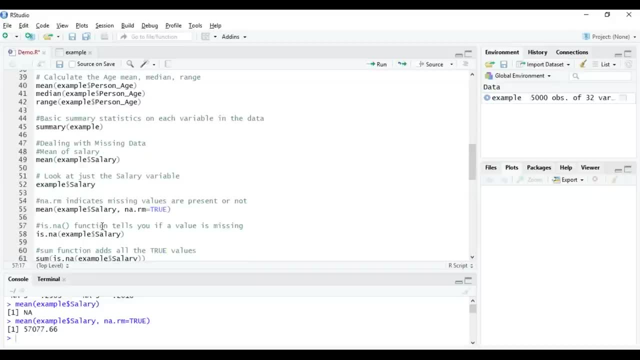 So what you can do is, if you just run this particular command, you can see that the mean value is basically 57,000.. Now, apart from this, you can also use a is not any function- which basically tells you if your value is missing. 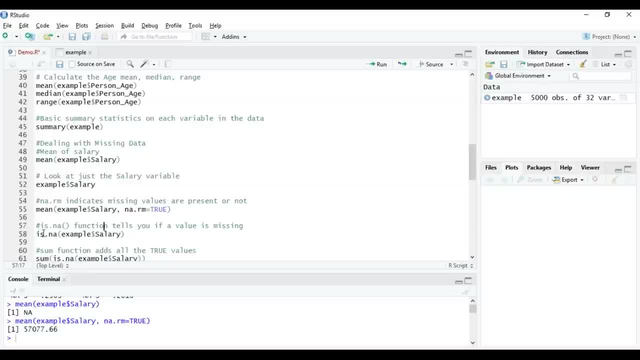 or not again. So what I'll simply do is I'll just mention this is not any function, and inside that I'll mention the data set dollar, the column name, since I want to find it for salaries column. I just mentioned that particular column and I'll run this. 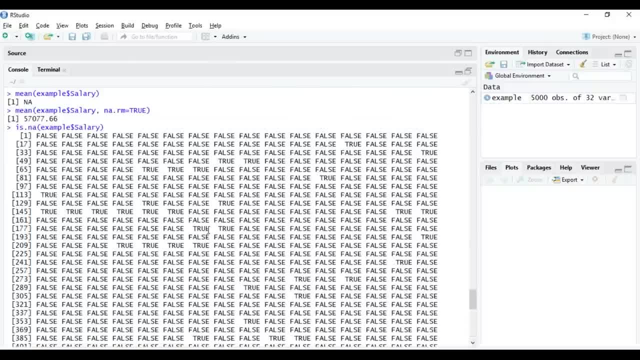 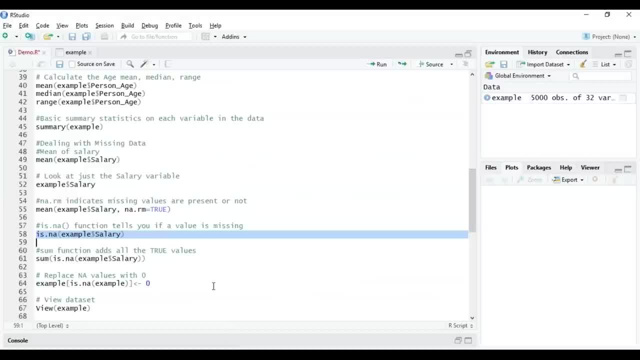 particular command. So this would basically return all the tuple values with either false or true. false means that you know there's no any value with it, and true means that there's an any value with it. So that's how you know you can find out if there is null value present in which. 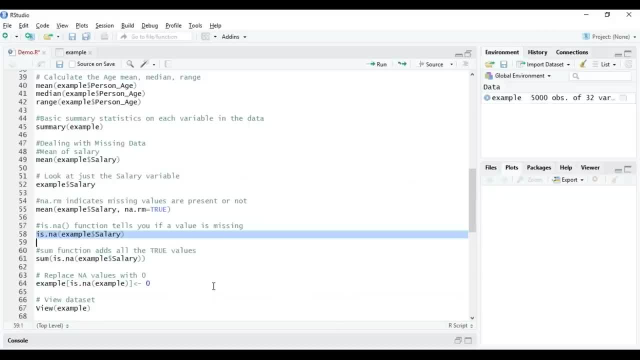 row or which tuple. that you have to understand, if you know. if you want to just add all the number of null values to calculate how many null values are present in total, You can just use the sum function. that is basically the aggregate function. in front of that is not any function to. 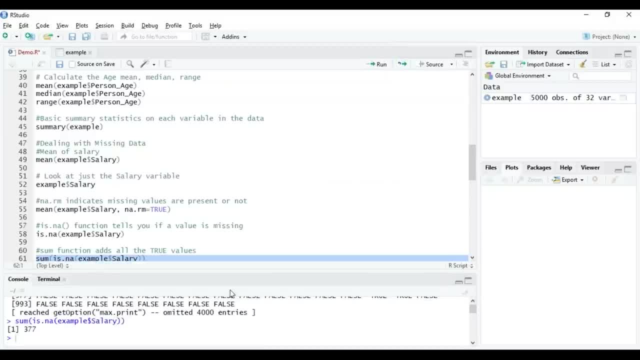 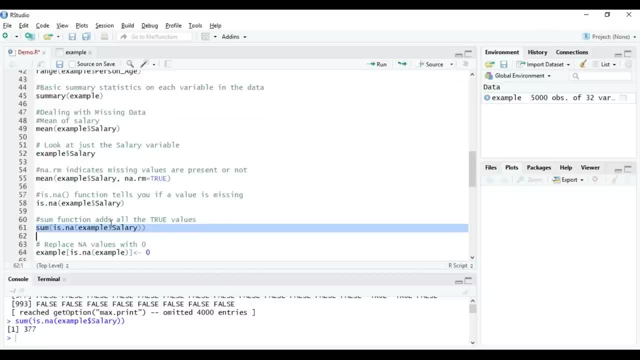 calculate the number of null values. So that's basically, it would count the number of true values and then it would print for you. So you can see that you know we have 377 values which have null values in the column of salary. 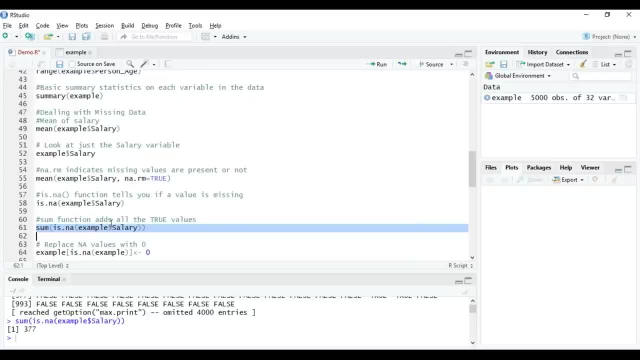 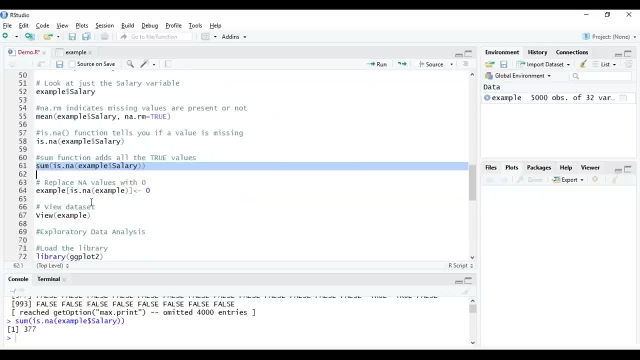 right. So now what I'm going to do is I'm going to just remove all these null values and then I'm going to replace them with the zero right. So for that, what you simply have to do is you just have to use this function of is not any mention the data set name. 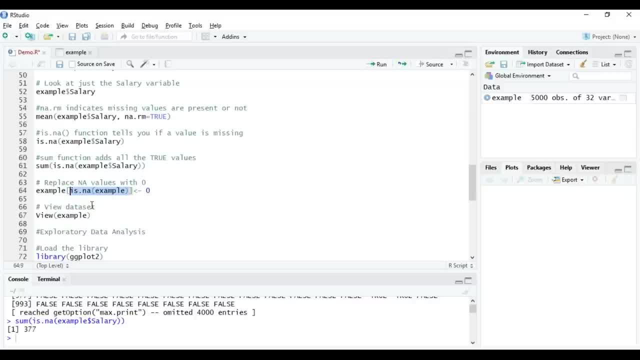 and then assign a zero to it and then assign it back to the data set, right? So I've put a zero and I've said: if is not any example, that means if there's a true value in the example data set, just replace it with a zero and then assign it back to the 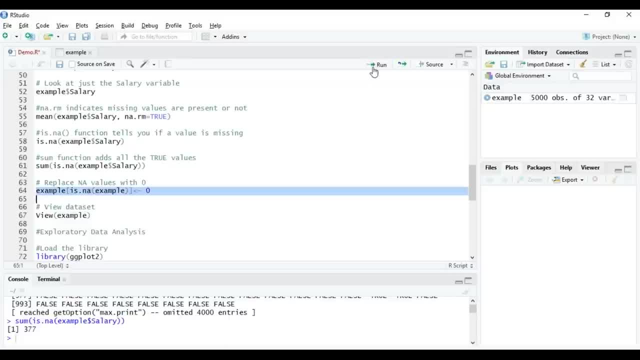 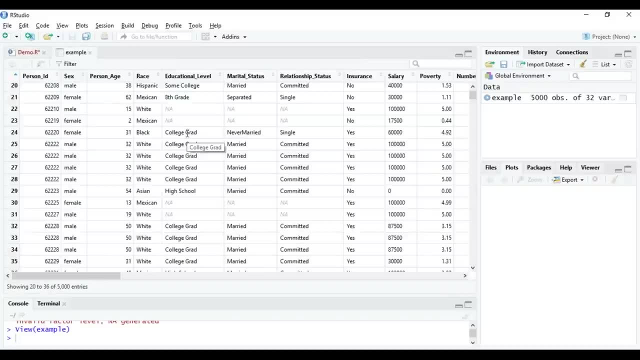 same data set. that is example, right? So I'll just run this particular command. and now let's just view the data set again. So I'll just view the example again. Now you must have observed one thing over here. That is all. the column with any values did not get replaced. 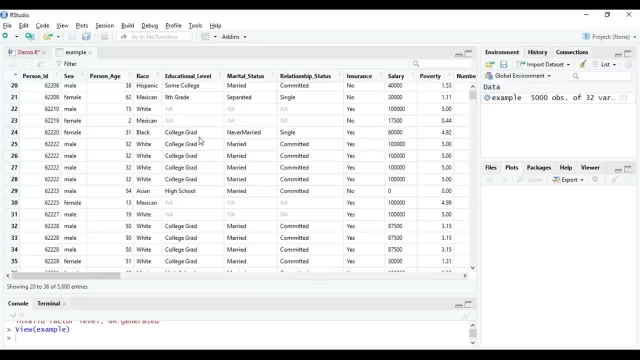 with zero. only the values you know which had the data type of end and they had. any values, got replaced with zero right for the other factors, like you know, your education level, martial status, relationship status. You can handle the null values based on various parameters. 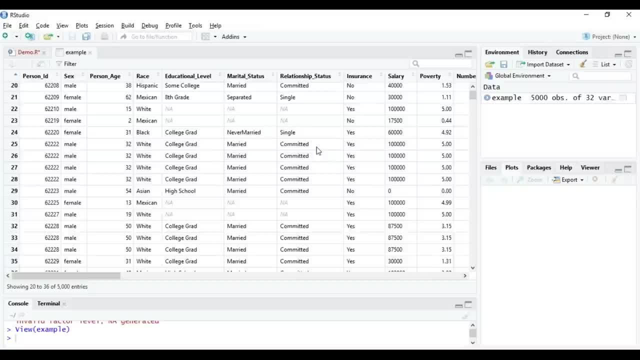 Like you know, you can just remove the tuples completely. You can just compare two factors and then mention the value Suppose. you know, if I just compare educational level and martial status, so I can see that you know, all the females belonging to the Mexican race can go to. 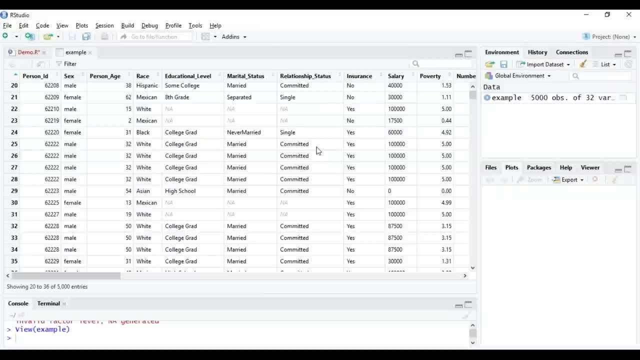 educational level of high school and our martial status are married right. So I can just replace these values- any values like that. So it's completely based on you how you want to deal with the missing data set Initially. I've just shown you how you can just remove the values and 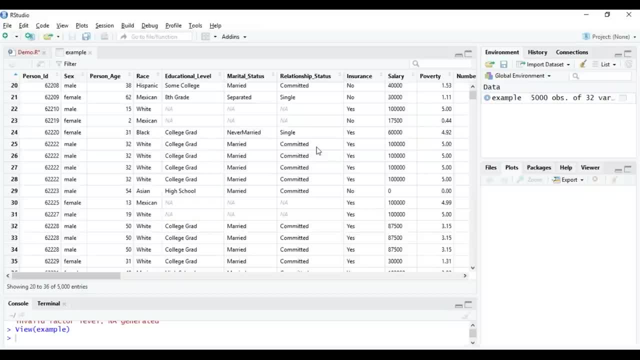 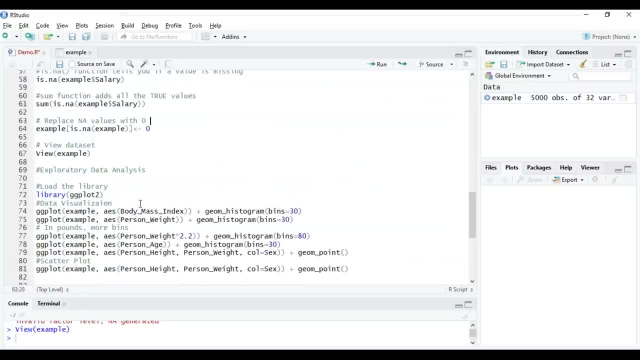 then how you can replace null values with something right. So I just leave that part to you so that you explore how you can do that. Now, moving on to the next part, that is basically the expertly data analysis, since we have analyzed the data and we have 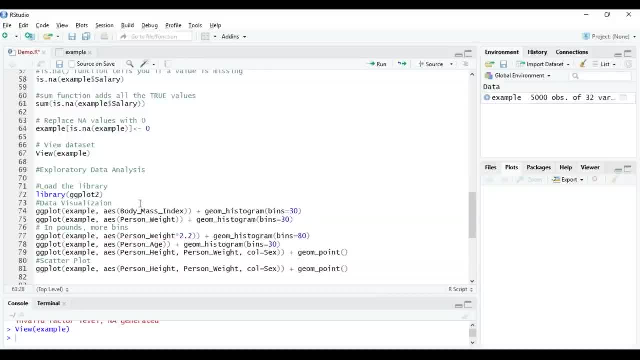 understood what are the various columns that can be analyzed and you know what are the various columns that have null values and how some values got replaced with zero. What I'm simply going to do is I'm going to perform the next step. that is basically the data visualization where I'm going. 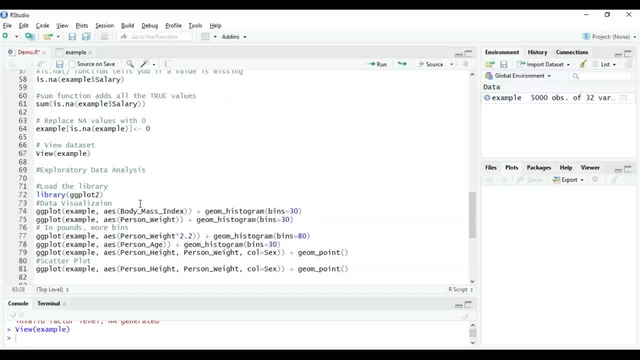 to plot histograms for different column values, right? So what I'm going to do initially is I'm going to use this GG plot to library, just in case you know, if you do not have it installed in your RStudio, you can again just install this particular package by just 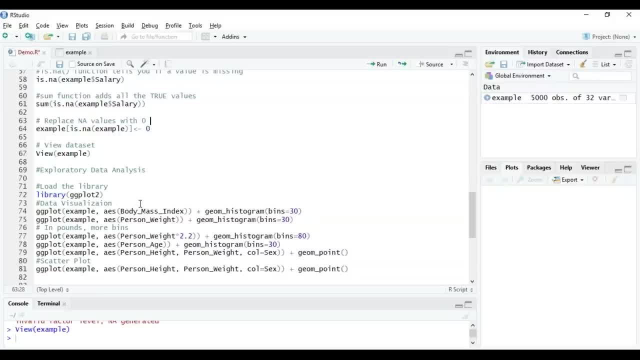 using the command installed or packages, and then just mention the package name and then you just have to load the library. since I've already installed the package in my RStudio, I'm just going to run this particular command to just load the library and then I'm going to perform data visualization. 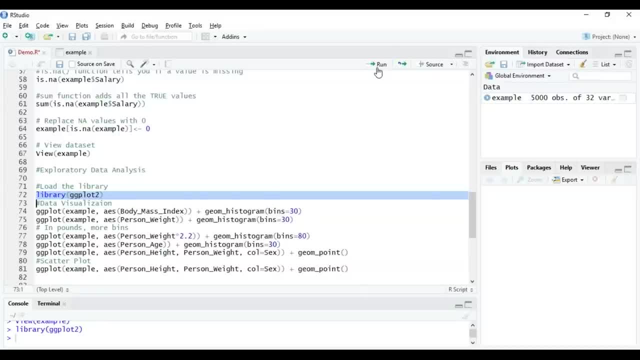 right. So if I just have to plot a histogram for you, what you can simply do is you can just use GG plot and then you have to mention the data set name- That is basically example- is variable- and then you have to mention the parameter based on which you want to plot the data. 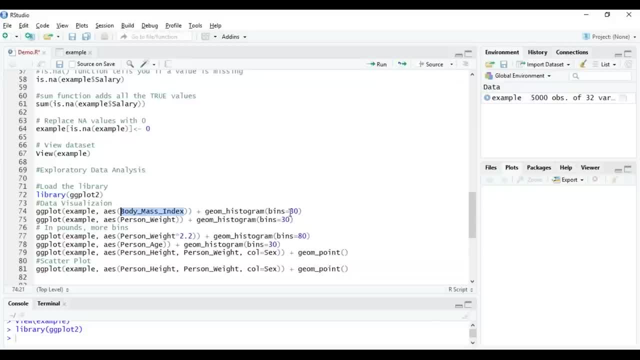 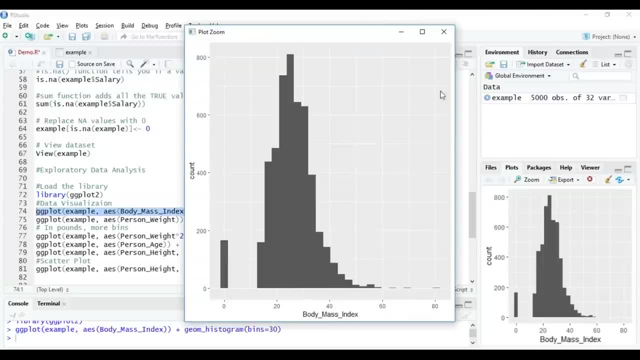 So initially I want to plot the data for body mass index and then I'll mention the bins to be 30, right? So I'll just run this particular command and then you can see the plot. So if I just zoom in this particular plot, 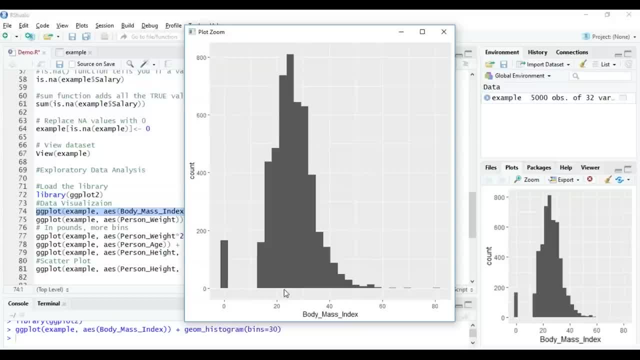 you can see that in a body mass index at the count around from 20 to 40- like let's say, you know around 30 or you know less than 30, is at the maximum right. So with this we can get the count of. 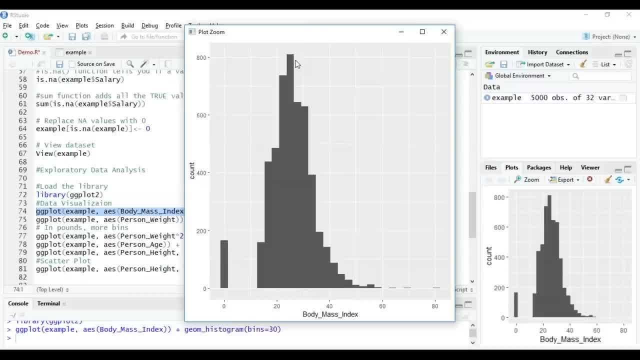 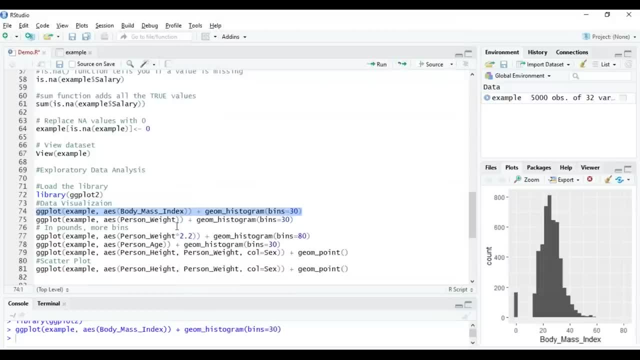 you know what is the least value of body mass index? What is the maximum value of body mass index? that is basically the least count and the maximum count, right? Similarly, I can plot a histogram for a person weight, So I'll again just use the GG plot function. 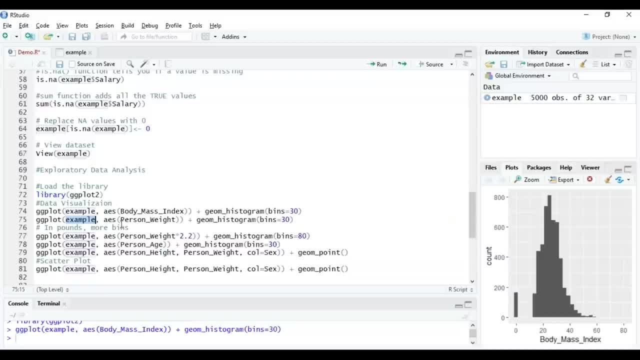 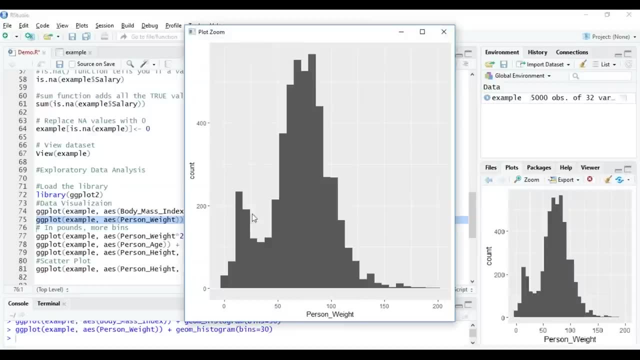 I'll mention the data set variable and then I'll mention person weight. that is basically for which I want to visualize the histogram, for so let me just run this particular command and let me just zoom in this plot So you can see that it is a person weight ranging from 50 to. 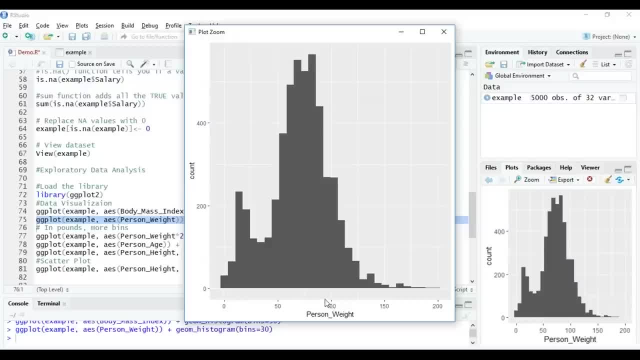 100.. Let's say, you know this is around 75, that is less, but it more than 75 to 100 is at the maximum values. So most people weigh around, you know, from 75 to 100 and very less people lay around from. 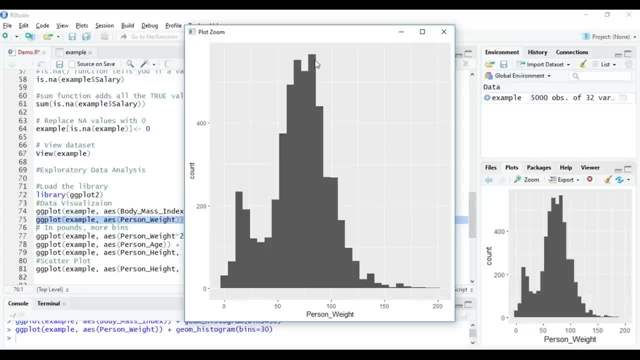 50 to 200 on. you can say: none of them almost weigh around 200, right? very few people wait. So with such kind of visualizations you can have a clear idea of you know how many people weigh more than, let's say, 100 or how many people. 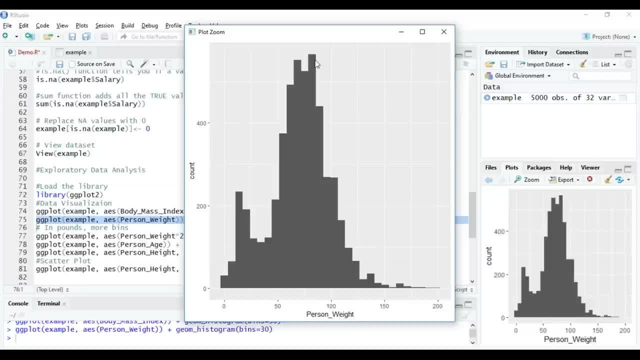 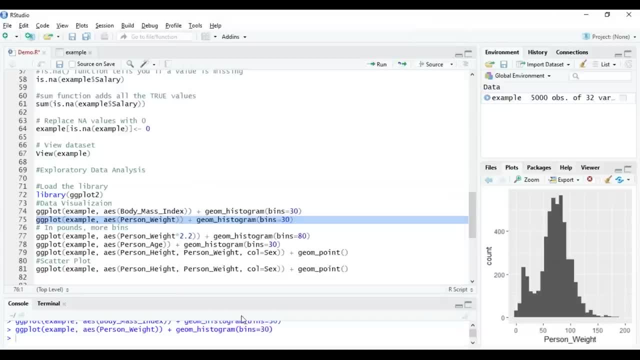 weigh less than 100, or what is the maximum weight around the samples data set that is given to you, or what is the minimum count of a weight of the sample set that is given to you, and so on. right, So now what I've done is this person weight histogram was: 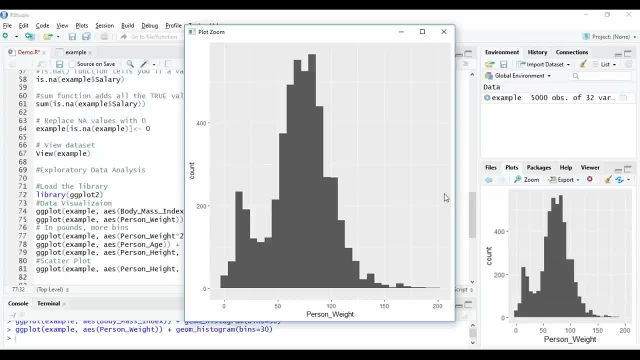 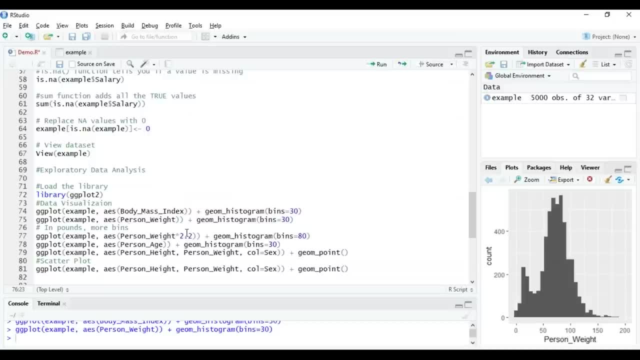 basically plotted on based on kgs. right now, if I have to just convert into lbs, what I've just done is I've just multiplied it with 2.2 and then I've given a lot number of bins, so that you know we get a clear visualization. 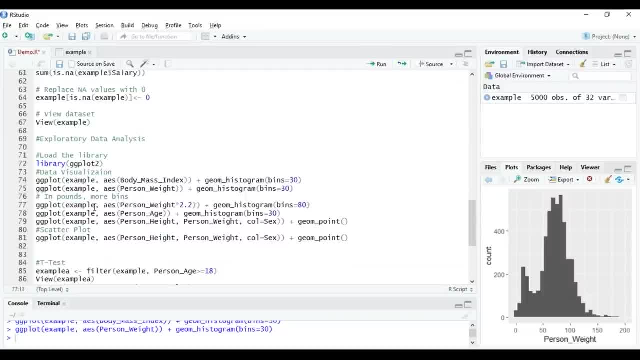 So I've again used the ggplot function and then I've mentioned the example data set and after that in the ace column I've mentioned person weight into 2.2, so that we want to convert the kgs to lbs, and then we've mentioned the number. 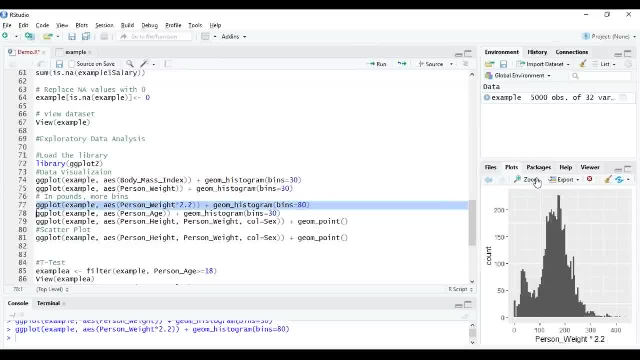 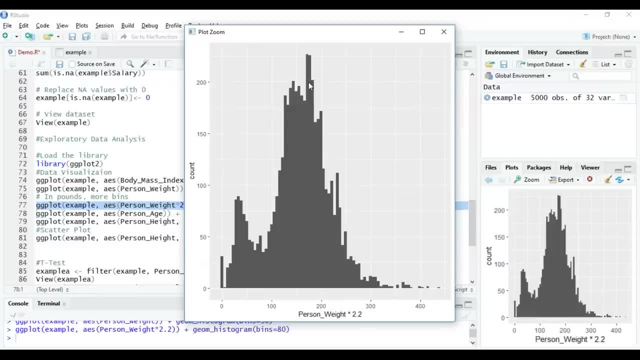 of pins. So I'll just run this particular command and then what we'll do is we'll zoom in so you can see that you know the weight- around 150 to 200 lbs- has the maximum number of count. if you just continuously keep zooming in and you keep increasing the 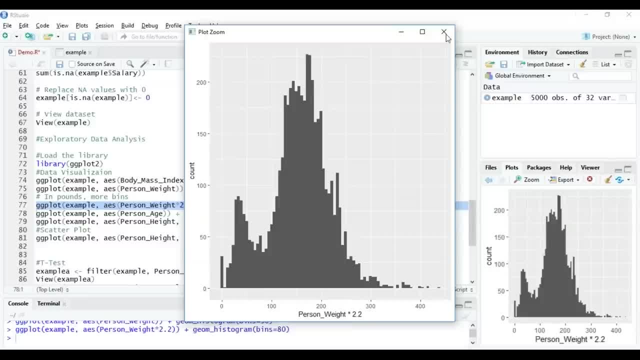 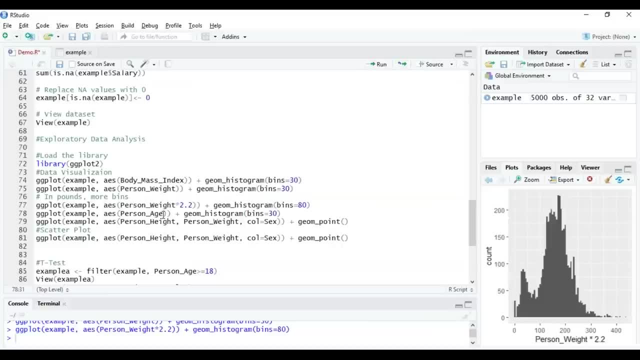 bins, you'll see the outputs more clearly, right? So that was about this plot, guys. Now, Similarly, what I've done is I've again plotted a histogram for age to know whether you know there are kids present at the age Distribution or not. 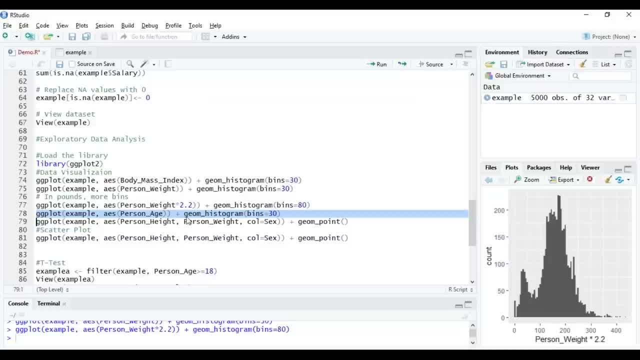 So what I'll do is I'll just run this particular command again, where I've mentioned ggplot- that is basically the ggplot function, the again data set name, the person age, that is basically the age column, and then I mentioned the pins. So when I zoom in, you can see that. you know. 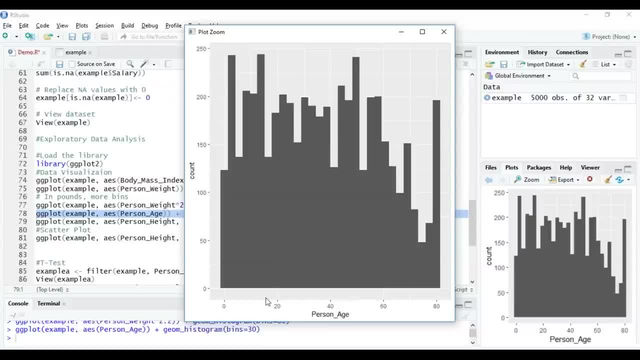 there are a lot of number of children's that are present in the sample data set whose age is less than 18.. So this is one category that you can again use to visualize or, you know, to analyze the data set. you can just divide your data set into children's data set and then adults data set. 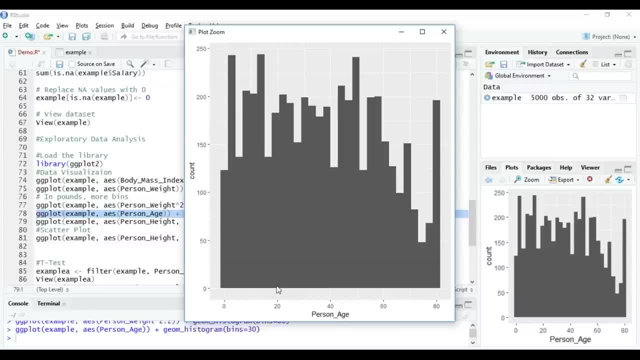 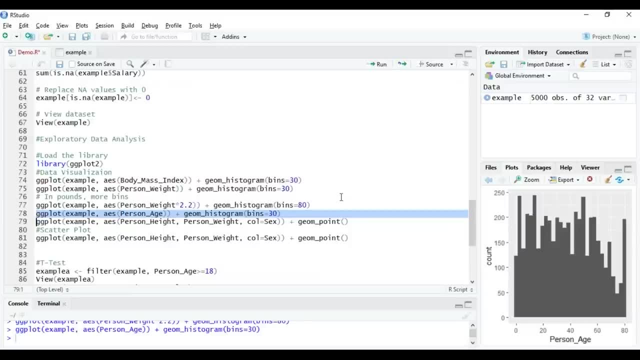 and perform various actions. So that's how you can use this particular visualization for your benefit. now, not only histogram guys. So, as I mentioned in the visualization part, in the theory section there are various number of plots, like bar plots, care plot line plot, box plot and so on. right, 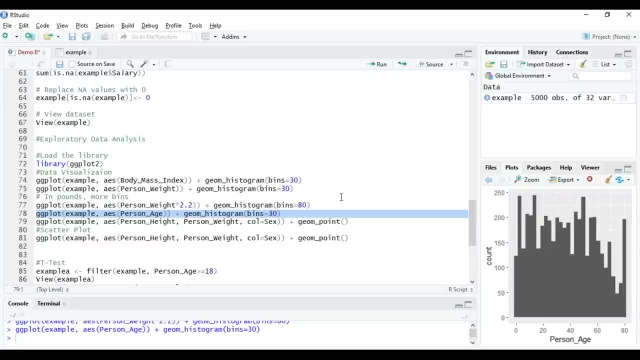 It's completely based on your understanding and your need. which kind of plot that you want to plot now? suppose I want to, you know, compare the person's height with the person's weight, and then I also want the parameter of gender to be present. what I can, 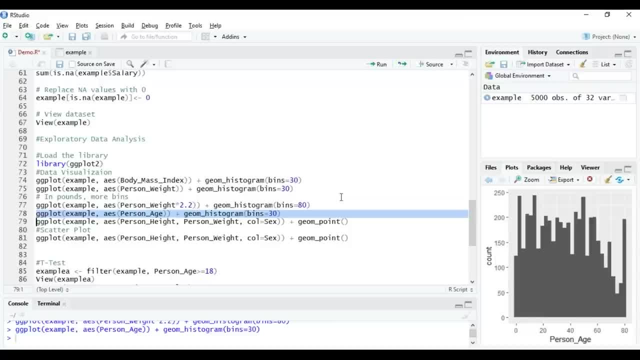 do is I can just simply plot a scatter plot where I'll compare person's height to person's weight and then just color the scatter plot with the help of gender right. So for that you can again use the GT plot. you can mention example. that is basically the data set, and then I'll mention. 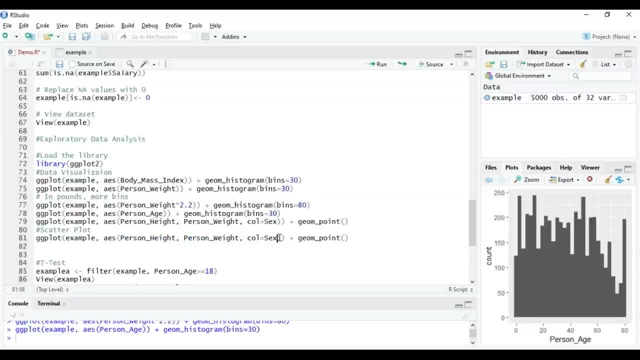 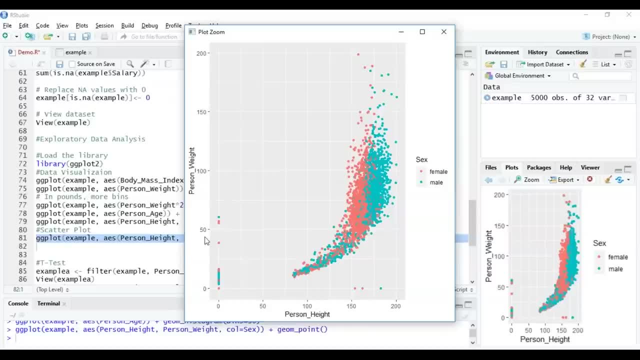 person height, person weight and then color by sex. that is basically a gender right. So when I run this particular command you can see the output that you know. we've got a plot, you know, of person's weight, person's height. So person's weight is compared with person's height. that is. 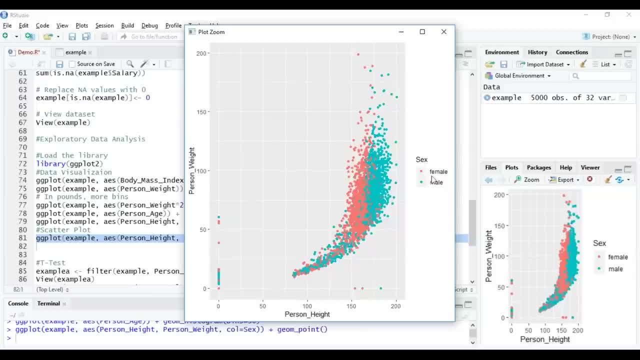 on the right hand That you can see that. you know the pinkish red color represents female and the blue color represents the male. if person's height was around hundred and that would be maximum of, you know, male people present in this particular section. 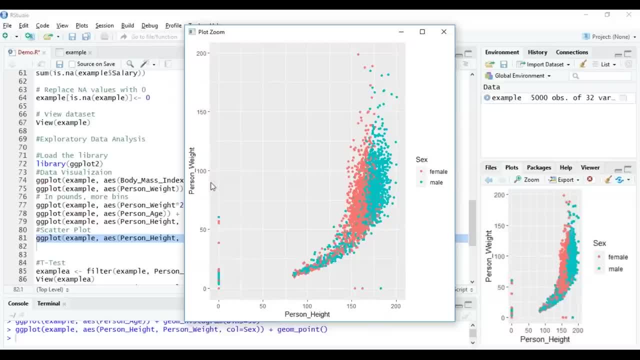 Let's say, you know the person's height is around 150 and the weight is also around, you know, hundred. we can see that you know there's a lot of female section present, right? So, guys, that's how you can use data visualization to perform. 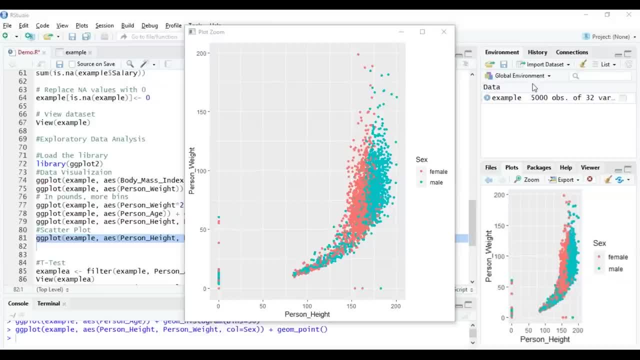 and understand various relationships between data. These were just few columns that I compared them and these were just few columns Or examples that I showed you when you can play around with data as much as you want. So this is just one more trick that whenever you create a 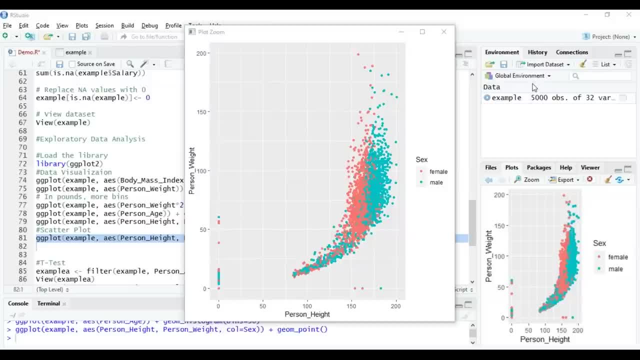 visualization. just make a note of it. What are you getting out of it, Right? So out of the visualization that you can see on the screen, What I'm basically getting is the person's weight to person's height comparison and how many female and male population is. 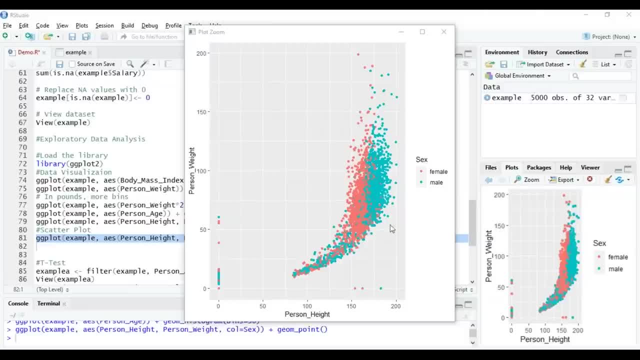 present in that particular scenario. So, as you can see, the maximum population is present in this particular range, you know, where the person's height ranges around 150 to 200 and the person's weight ranges around, again you know, let's say, 125. 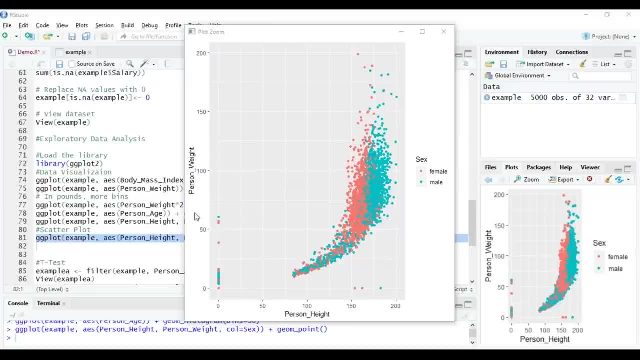 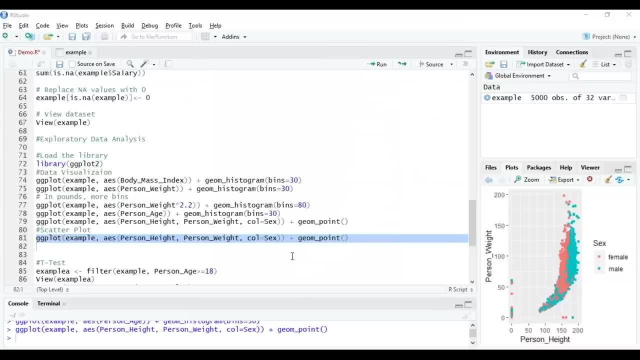 250, right. So that's how you can analyze data and gain some hidden insights. now, moving on to the next part, that is basically the inferential statistics. What I'm going to do is I'm going to perform t-test. So when I say t-test, t-test are a type of hypothesis testing. 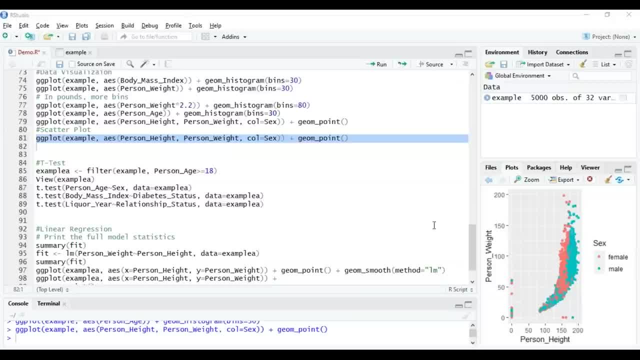 by which you know you can compare means. so each test that you perform on your sample data basically brings down your sample data to a single value, That is the t-value. So, as you can see on the screen, this is basically the formula of t-value. 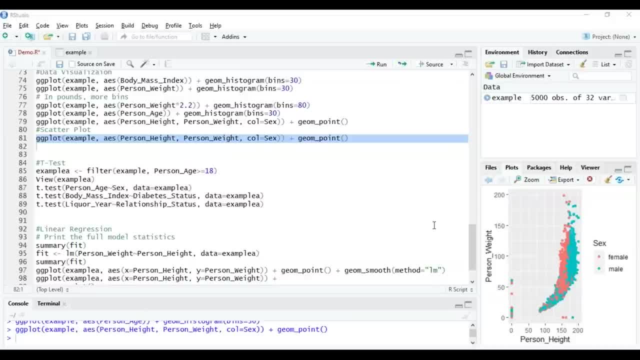 So now what I'm going to do is I'm basically, you know, go to filter the data set first. So, to filter the data set, what I've just used is, I've used the filter function, I've used the data set name. that is basically example- and then 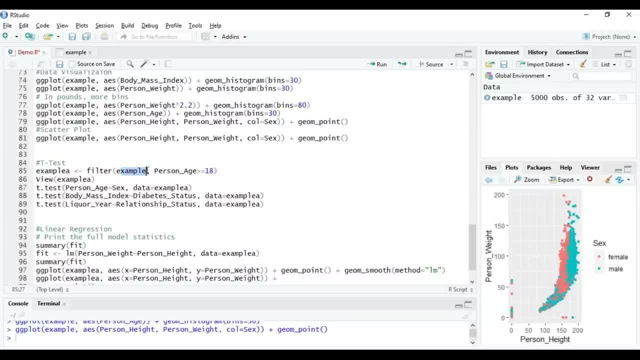 you have to mention the parameter based on which you want to filter the data set. Now, what I'm going to do is I'm going to just consider the adults, So I've just mentioned person's age to be greater than or equal to 18. after that, the complete data would be assigned to an. 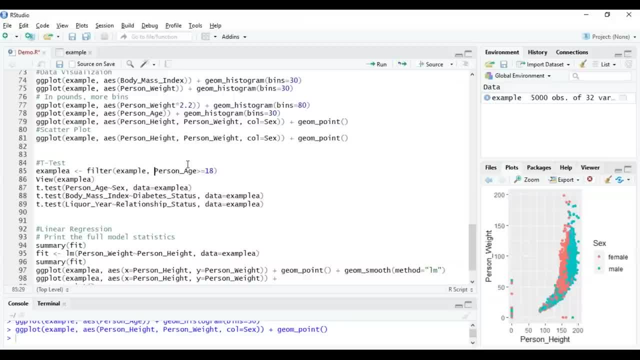 different variable, that is, example, a right. So that's how you can filter the data set. So now, if you have any question that you know, why have I filter this data set? Well, this is just like a precaution measure to you know. 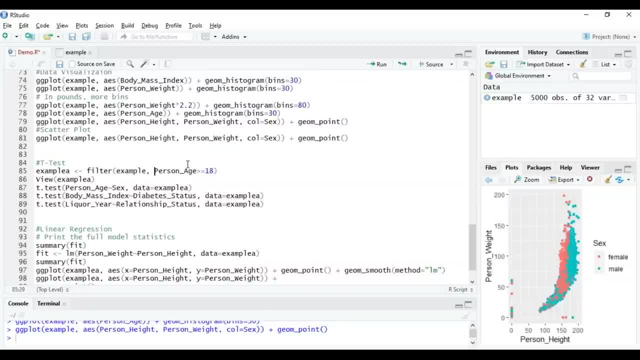 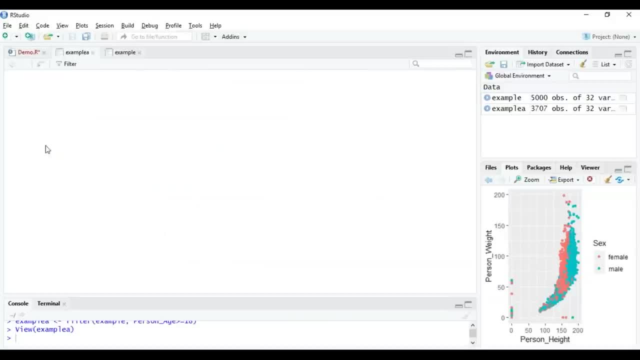 to make us prevent from making any mistakes downstream when we keep analyzing the data, right? So now what I'll do is I'll just run this particular command and then I'll view the data set. So when I say view example a, you can see that you know. 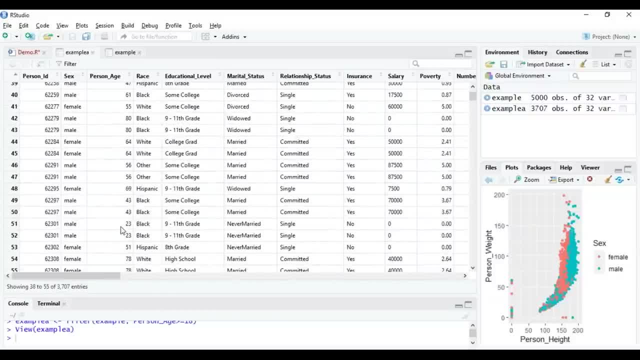 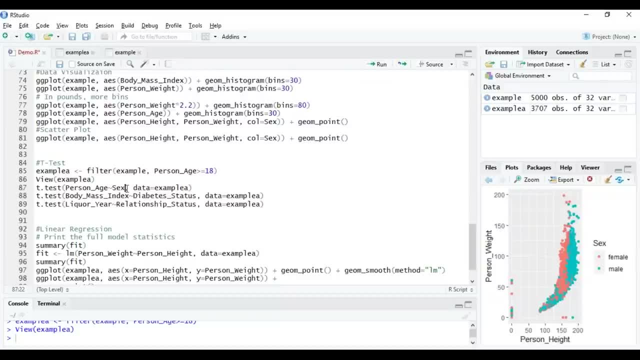 the a person's age is obviously greater than or equal to 18.. So there's no child present in this particular data set. Now, what I'm going to do is I'm going to perform t-test. So, as I mentioned before, t-test is basically used to compare the. 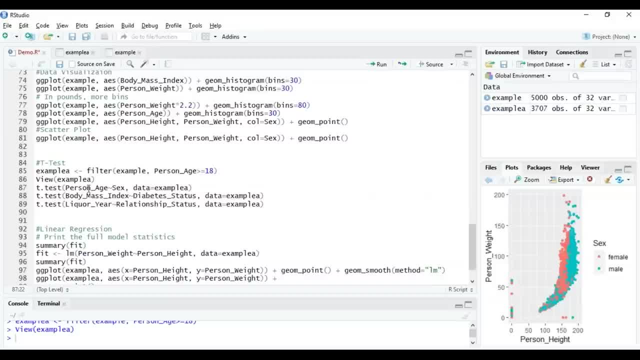 means. So what I'm going to do is I'm going to use this predefined function in R to perform t-test- that is ttest- and then I'm going to perform the t-test between person age and sex, right, So the person's age is basically the response and the sex is. 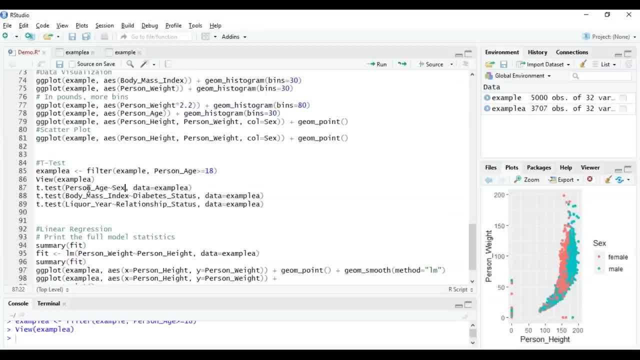 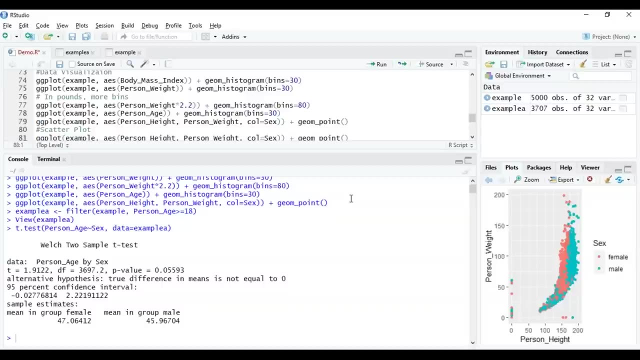 basically the group. So this is basically a formula method to perform t-test in R and data is basically your data frame. that is example a over here. So when I run this particular command you can see an output that you know. we have data to be person age by sex, and t is 1.9122.. 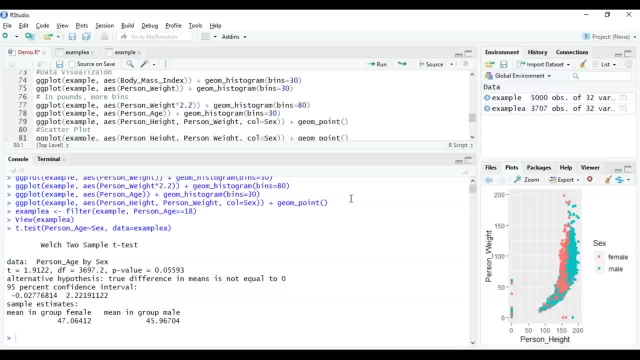 That is basically the t-value that is calculated and the p-value is 0.05593.. So when I say t-test, t-test is basically used to calculate the p-value. that is basically the confidence value. So this value basically tells us that. you know. if the p-value is less than 5%, that is 0.05, then the t-test between these two values, or you can say the alternative hypothesis between these two values, is getting rejected. But yes, if it is more than that, then you can consider that unit is around 95%, correct or apt? 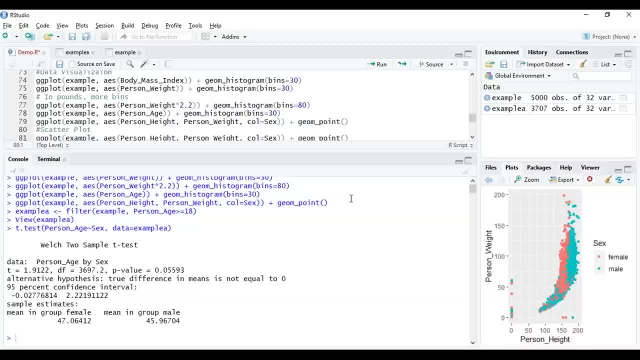 to the sample estimates, right? So basically, with the t-test that I perform for person's age and sex, what I'm basically trying to find: is there any difference for the age of males versus females in this particular data set? So, since the p-value is greater than 5%, you can see that you. 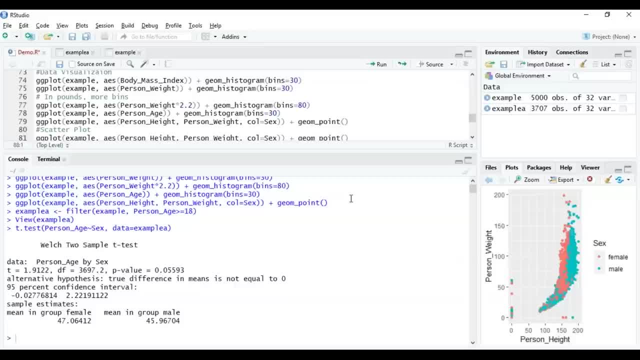 know the mean in group of female is around 47 and mean in group of male is around 45. So yes, you can see that you know it does. there is a difference in Age of males versus females in this particular data set. now, 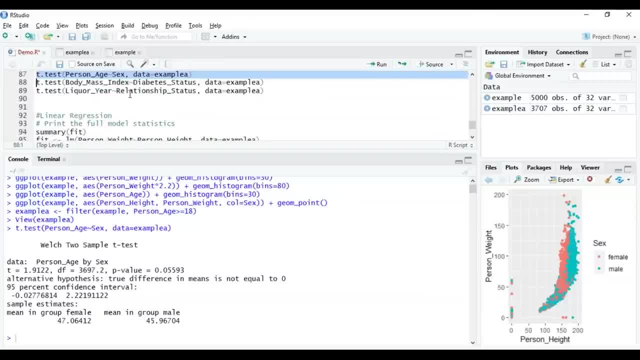 moving on to the next t-test, that is basically the t-test between body mass index and the diabetes status. Well, I'm performing the status to identify whether the body mass index differs between diabetics and the non-diabetic patients. So again, 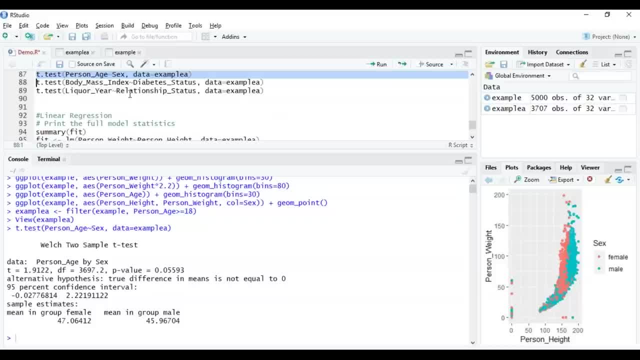 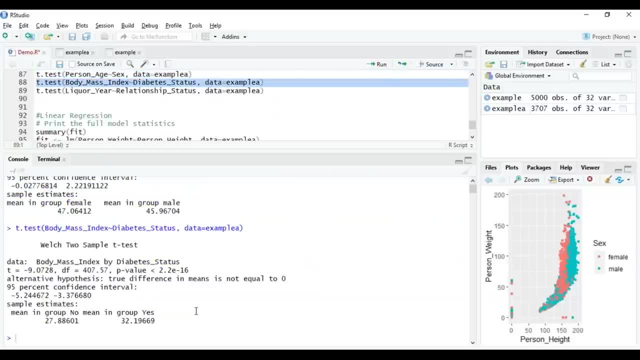 what I'm going to do is I'm going to choose this function, tt test- and then I'm going to mention body mass index over diabetes status, and then I've mentioned the data frame, right, So I'll just run this particular command here. 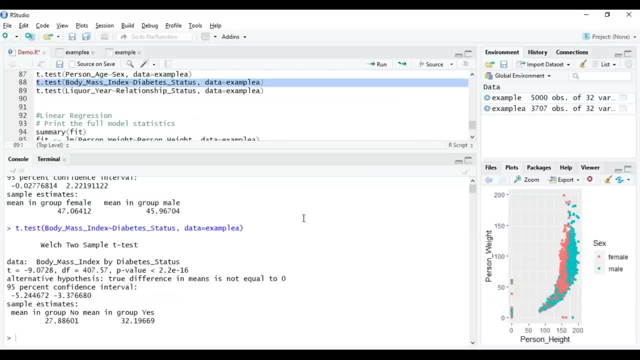 You can see that. you know the p-value is less than 5%. That means that obviously your hypothesis is going wrong. And then obviously the answer to this question is no. that means the body mass index is not differ between diabetics. 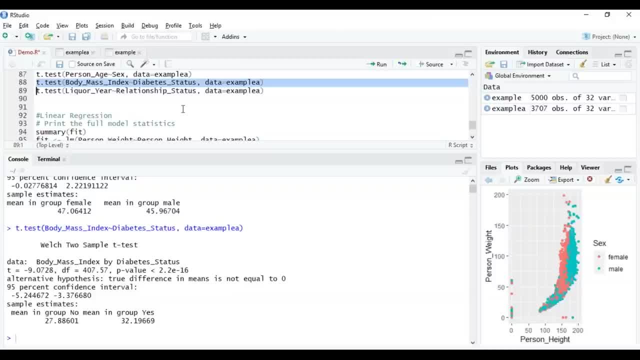 and non-diabetic patients. Moving on to the third t-test that I want to perform, that is liquor year versus relationship status. So basically this t-test is trying to answer to single or married people drink more alcohol or not? So again, I've just mentioned tt test. 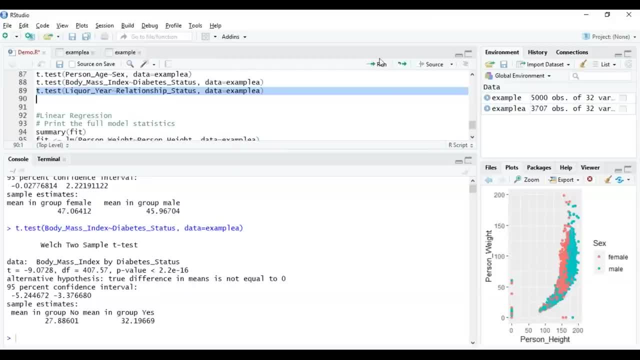 I mentioned liquor, year, relationship status and the data frame, I'm name and then I'll run this particular command and you can see that you know p-values again, less than 5%. that means obviously there is no connection between both these values. So that's how folks, you can understand how various columns 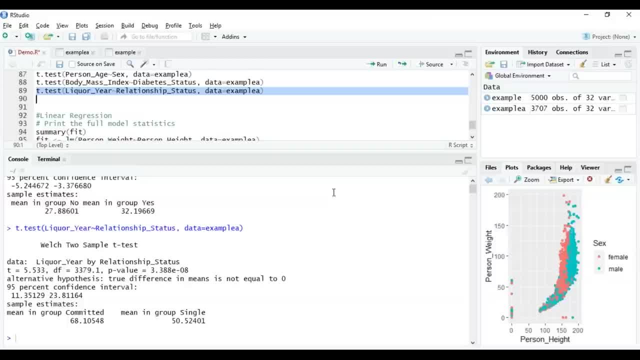 differ over each other or various columns can be related with each other. Well, so that was all about details, guys. Now, these were the ways, kind of skills, as I mentioned before, a data analyst should possess. now, moving on to the last skill, that is basically the machine learning. 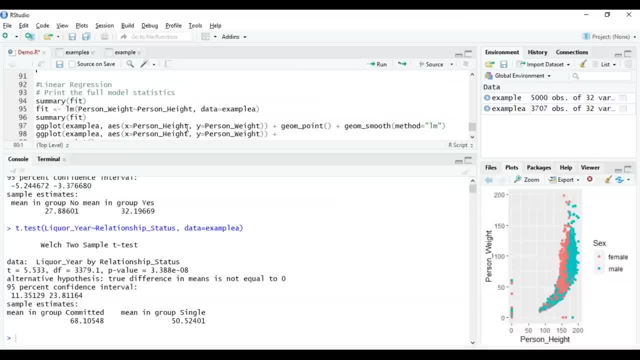 So, as I said before, knowing machine learning is a bonus point. now, obviously, how would you perform machine learning? that is, basically, you have to understand the algorithms and you have to build a model for it. So what I've done over here is I am going to just use the 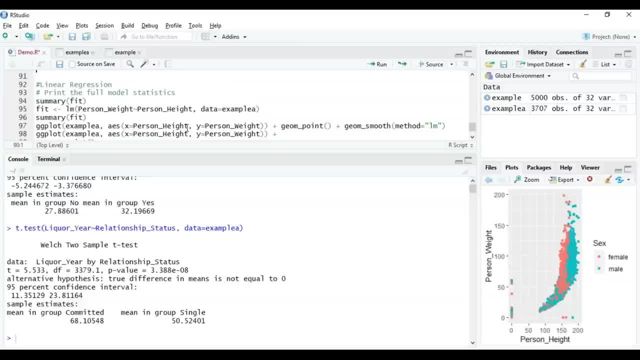 linear regression over here. So, as you know, the linear models are basically the mathematical representations of the process that we think give rise to our data right. The model basically seeks to explain the relationship between a variable of interest, that is basically our Y variable. 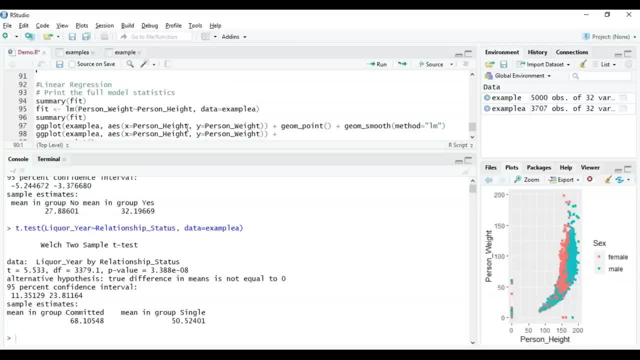 which is also the outcome response or the dependent variable, and one or more X predictors are the independent variables. So if you have Y equal to B naught plus B 1 X, then you know X is basically the independent variable and Y is the dependent variable and B naught is the intercept and B 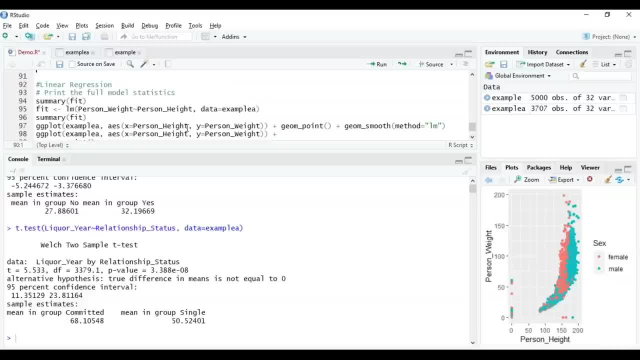 1 is basically the coefficient that describes what one unit change in the X would do, the outcome variable Y, right? So that was a basic about linear regression, guys. now building a linear model basically means that you know, we propose a linear model and then estimate the coefficient. 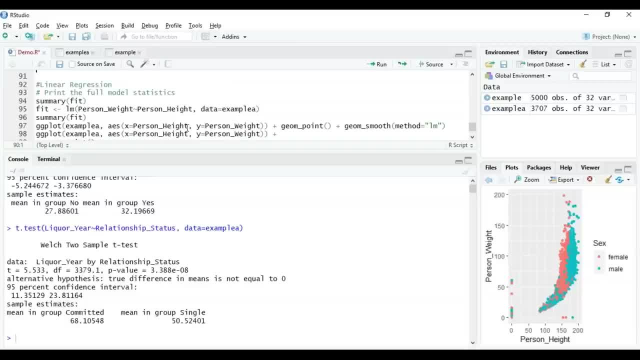 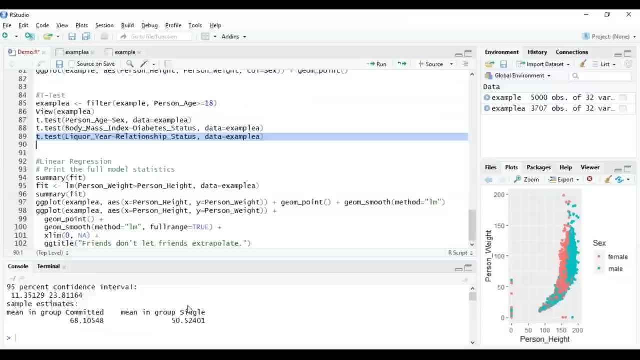 And the variance of the error term. So, as you can see, if you want to build a linear model in R, then you can just simply use the inbuilt function for linear regression, that is, LM function, and then you have to mention the columns between which you want to calculate these values. 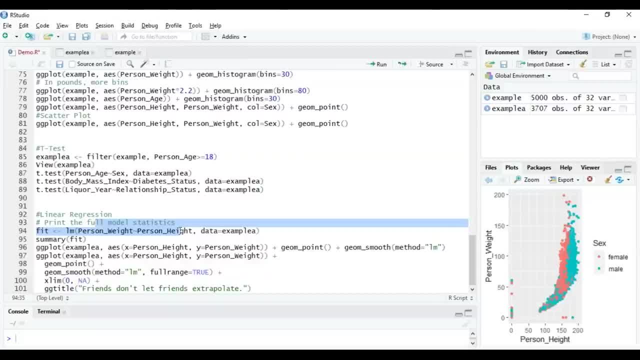 right. So basically, I've decided to find the linear regression model for about person's weight upon person's height and then over here in the data. I've mentioned my data frame right now. after that I'll just assign it to fit. So let me just run this particular command. 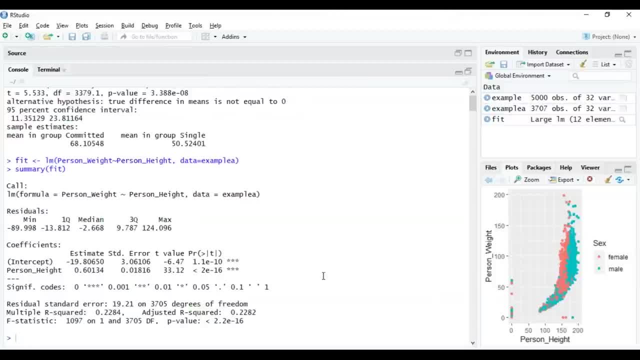 Now, after that we'll just find the summary of fit, right. So when we find the summary of fit you can clearly see that. you know the p-value is less than 2.2 into 10 power minus 16. So that means the intercept term is not very useful most of. 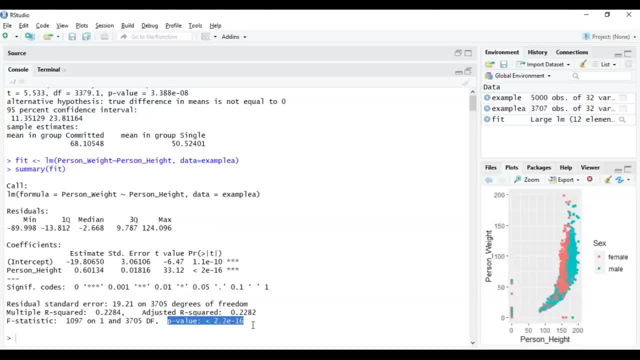 the time. So this basically shows us what the value of weight would be when the height would be zero, right, So the value of weight would be around minus 19, which is impossible, So that could never happen. But if you observe the height coefficient, we can see that you. 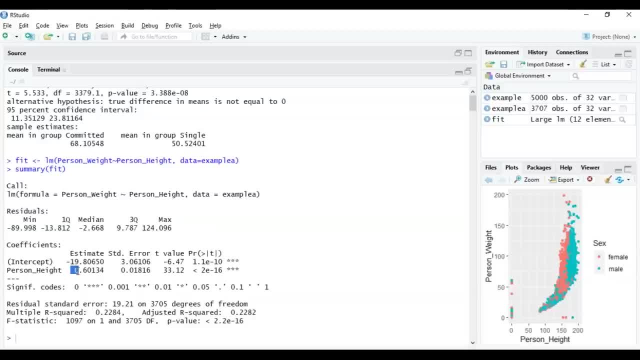 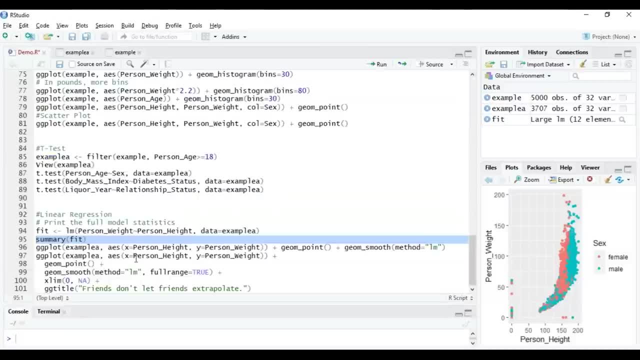 know it's really meaningful, because each one unit increase in the height results in around 0.6 increase in the corresponding unit of the weight. right Now, if you just want to visualize this particular model, what you can simply do is you just have to use the ggplot function. 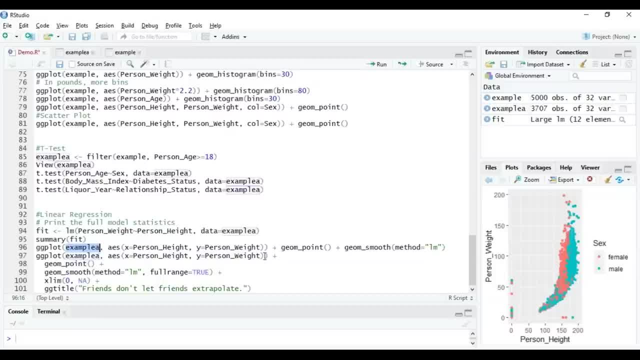 and then you have to mention the data set, that is, example a over here mentioned person height, person weight, gm point and GM sport method to be LM right. So if I just run this particular command you can see that you know we get a plot. 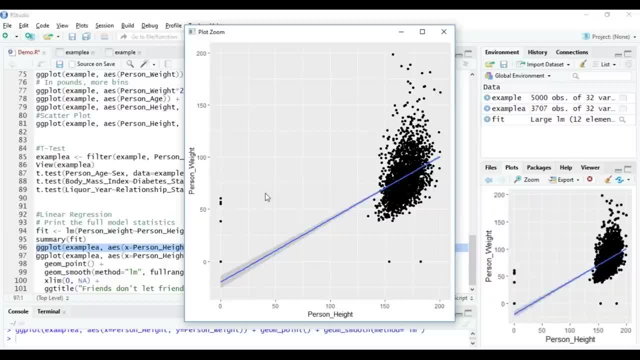 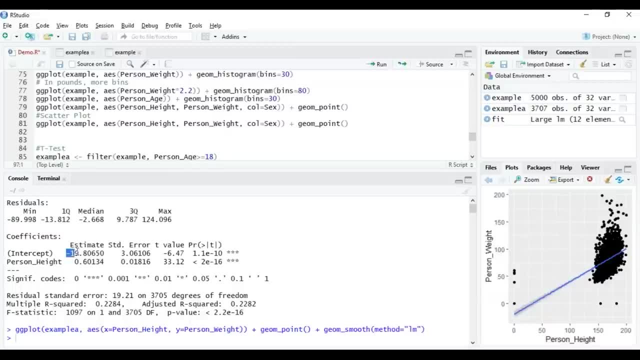 So, by default, you can see that you know this is only going to show the production over the range If the data, which is very, very important to know. So, for example, if you clearly see the linear model, tells us that you know the weight would be around minus 19.8 kgs when the height is. 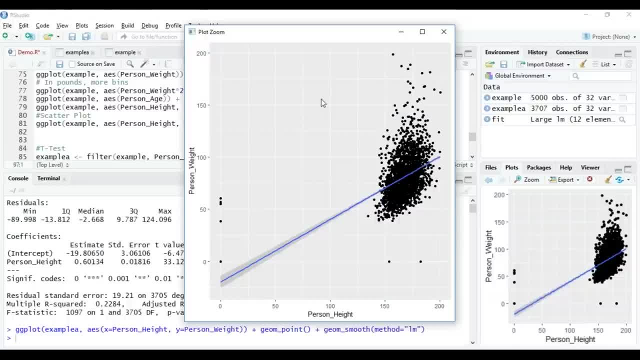 0. now let me also tell you that you know you can extend the predicted models regression line past the lowest value of the data term to hide 0, and also the bands of the confidence intervals basically tell us that the model is apparently confident within the regions that is defined. 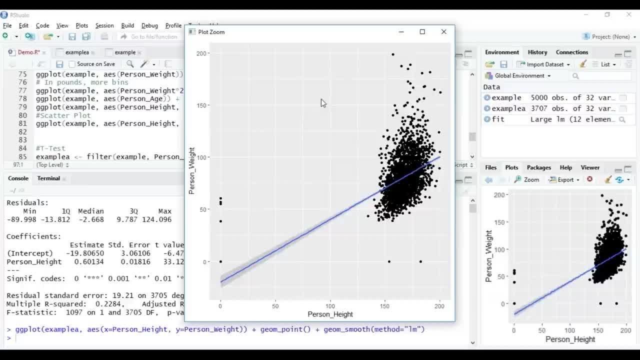 by the gray boundary. But if you just think about one thing over here, we would never see a height of 0 right? So basically, predicting past the range of the available training data is not a great idea, I would say, because there's no point is predicting the past. 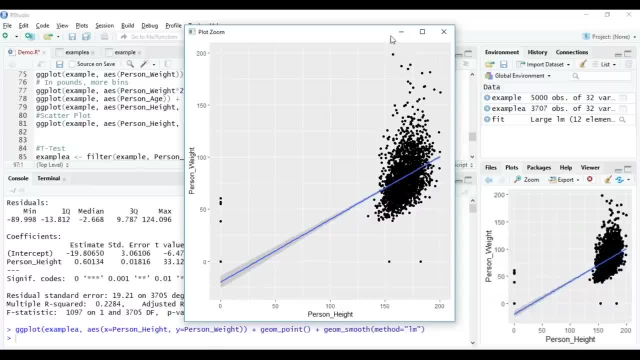 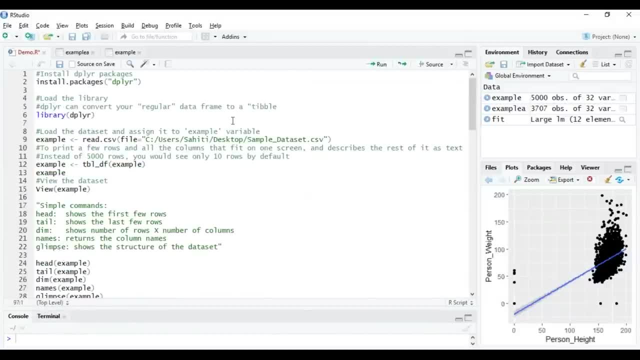 range of data, as the height would never go 0, right. So, guys, that was about linear regression. So what we did in this particular demo was we started by importing the data set and then we learned how to view the data set. after that, we went through few simple commands. 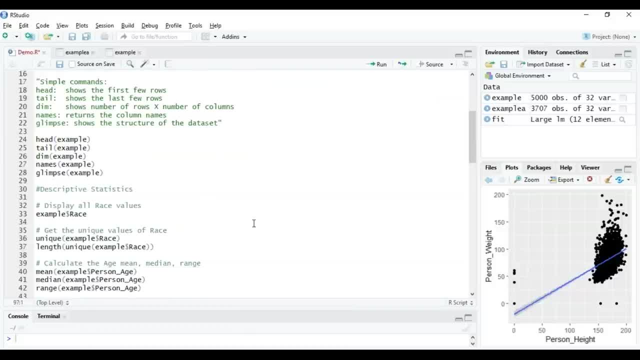 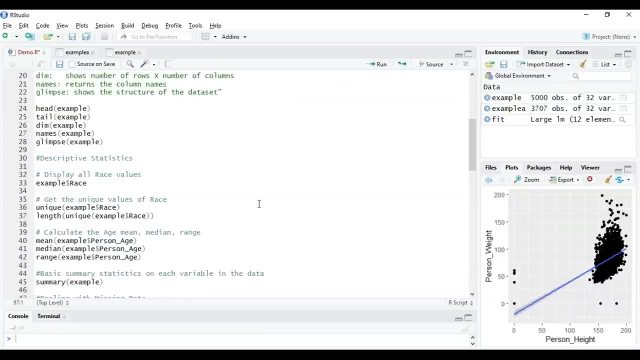 That is the head, tail, dimension, names, limbs. and then we understood how to perform descriptive statistics Six on a data set. So we understood how to use the unique function, the length function, the mean median and the range function. after that I also told you how you can deal with the missing data that 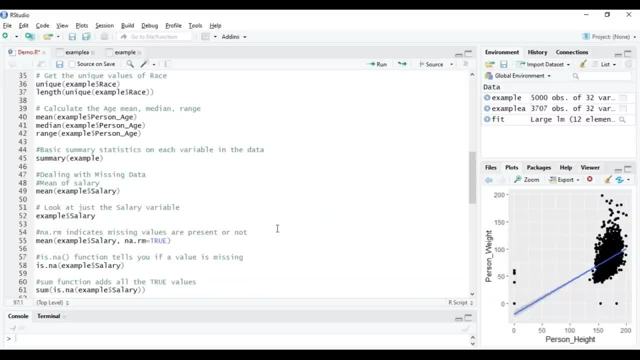 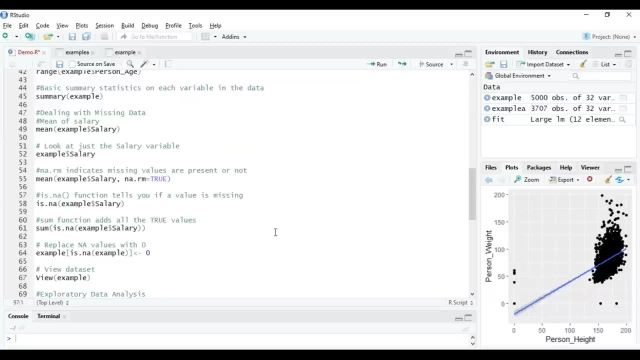 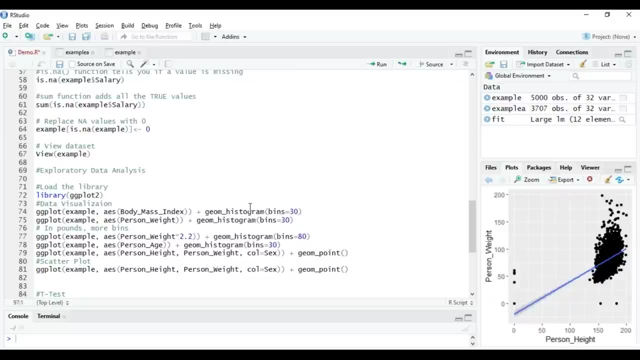 is basic by using the na dot rm parameter and also the is dot any function. and finally, you can replace all the na values with the zero, but only for those column with the data type end. and then we performed exploratory data analysis, where we perform visualizations between various columns and we 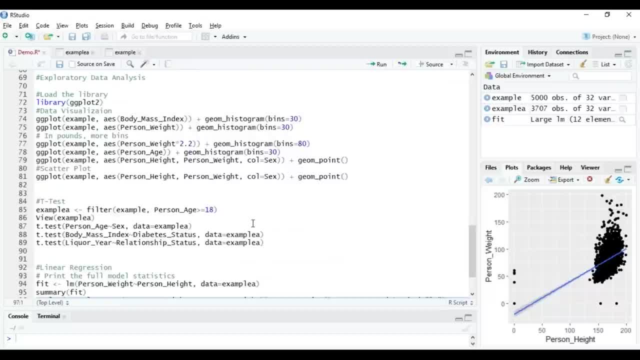 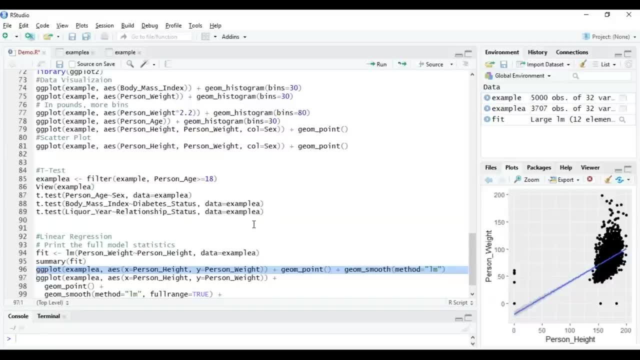 understood the relations between them. And then we finally perform t-test to understand and answer few questions and perform linear regression. that is basically a machine learning model, right? So I hope that you know you've understood this particular part of the session. So, folks, that was all about data analytics.